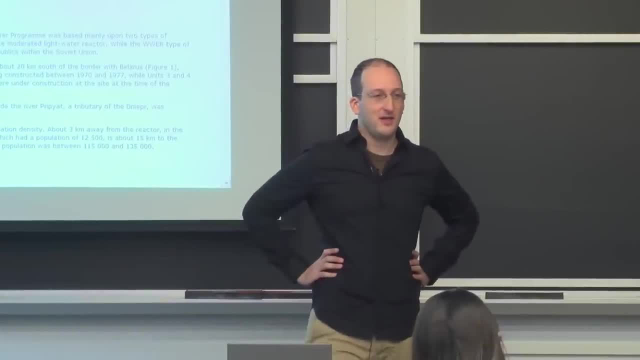 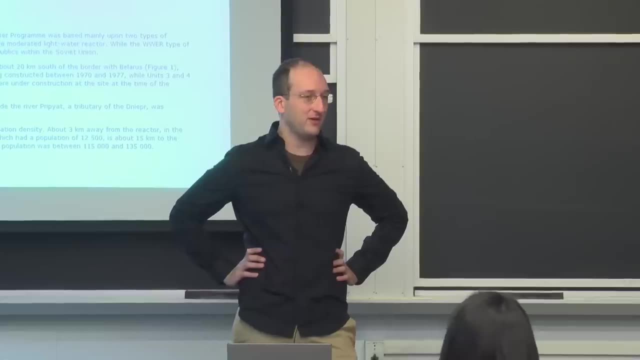 All right. so, like I told you guys, Friday marked the end of the hardest part of the course and Monday marked the end of the hardest p-set. So because the rest of your classes are going full throttle, this one's going to wind down a little bit. So today I'd say sit back, relax and enjoy. 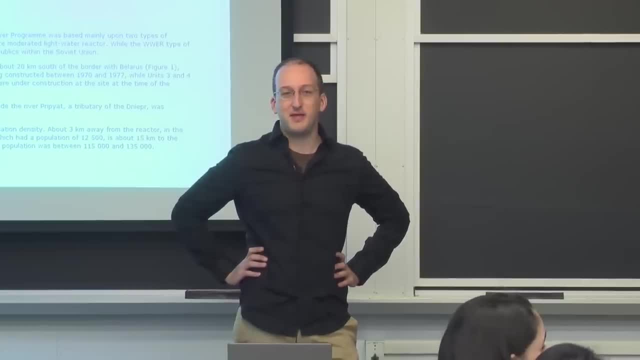 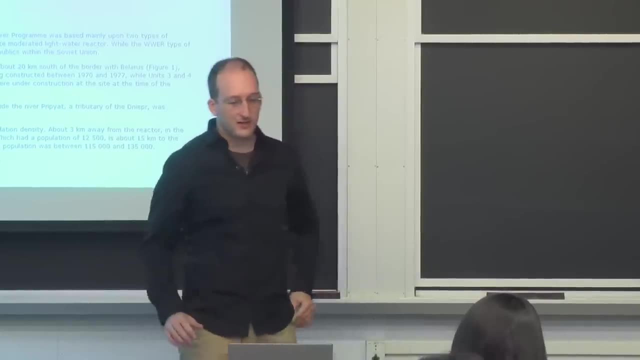 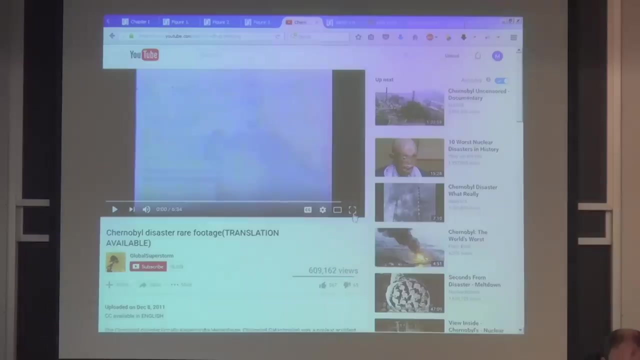 a nuclear catastrophe, because we are going to explain what happened at Chernobyl. now that you've got the physics and intuitive background to understand the actual sequence of events. To kick it off, I want to show you guys some actual footage of the Chernobyl reactor as it. 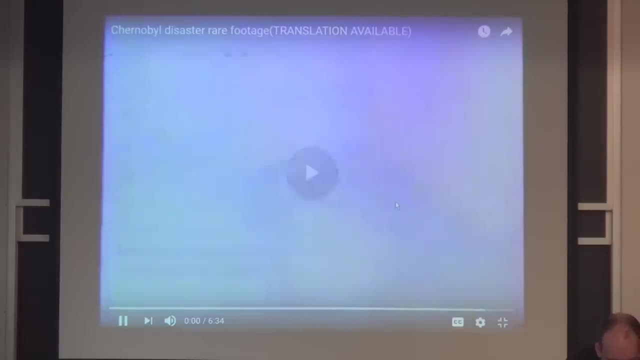 was burning. So this is the part that most folks know about. This is footage taken from a helicopter from folks that were either surveying or dropping materials onto the reactor. That was probably about it, But I would definitely say this is a bad idea. 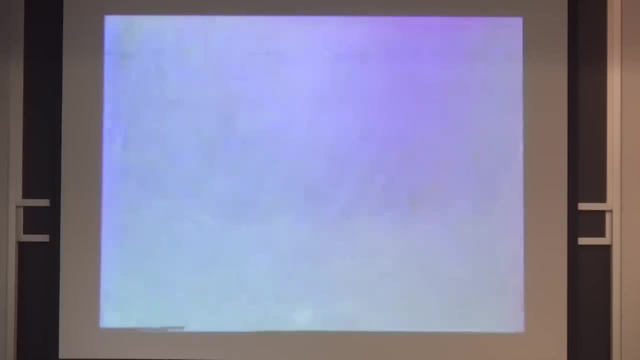 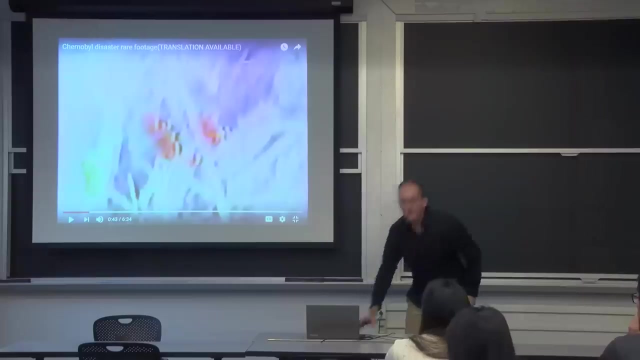 Hold where the smoke is. We'll get into what the smoke was. So that red stuff right there, that's actually glowing graphite, amongst other materials of the catastrophe, amongst other materials from the graphite fire that resulted from the RBMK reactor burning. after the Chernobyl accident, caused by both flaws in the physical design of the RBMK reactor and absolute operator stupidity and neglect of any sort of safety systems or safety culture. We're lucky to live here in the US, where our worst accident at Three Mile Island- was not actually really that much of an accident. There was a partial meltdown. There was not that much of a release of radionuclides into the atmosphere because we do things like build containments on our reactors. If you think of what a typical reactor looks like. 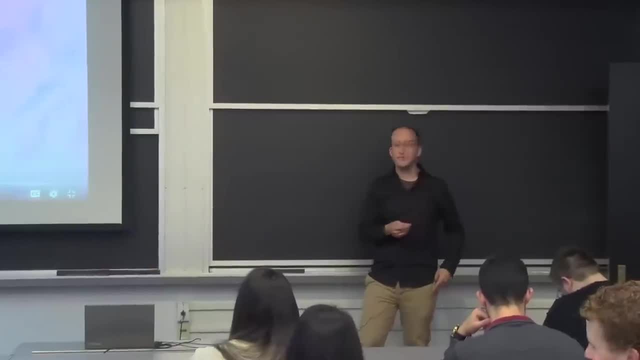 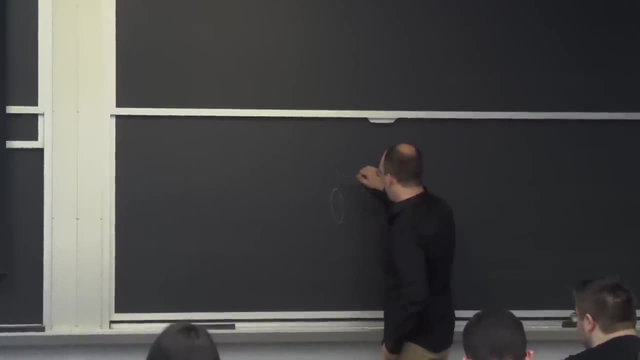 like if you consider the MIT reactor as a scaled-down version of a normal reactor or, let's say, a commercial power reactor. you've got the core here, you've got a bunch of shielding around it and you've got a dome that's rather thick. 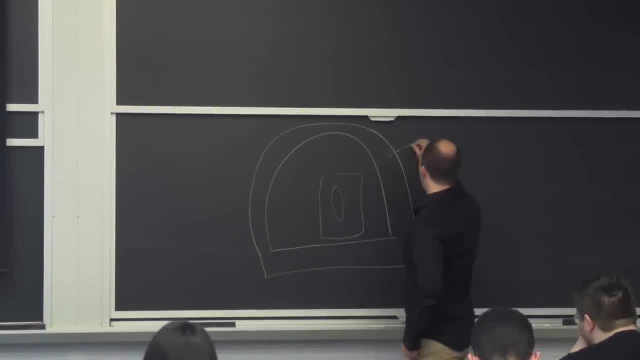 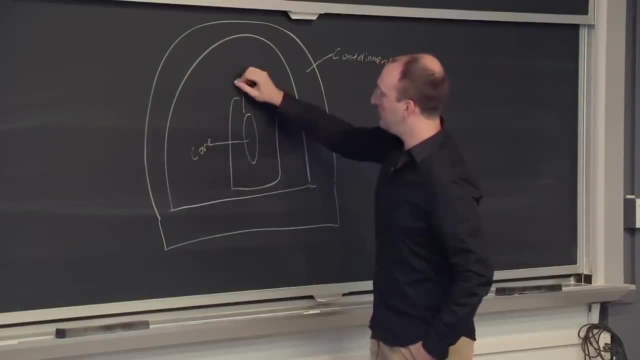 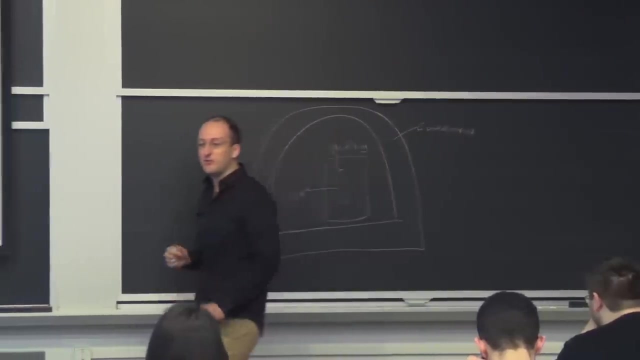 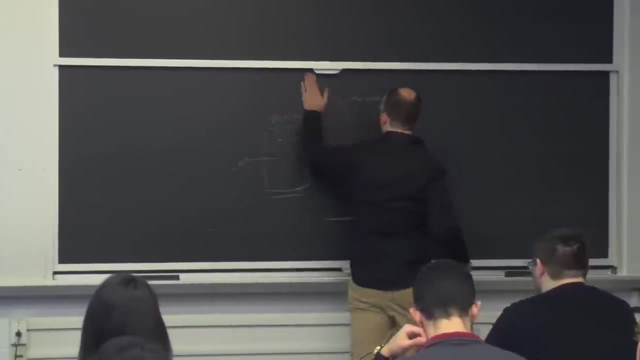 that comprises the containment. That would be the core. This would be some shielding. So this is what you find in US and most other reactors. For the RBMK reactors there was no containment because it was thought that nothing could happen. 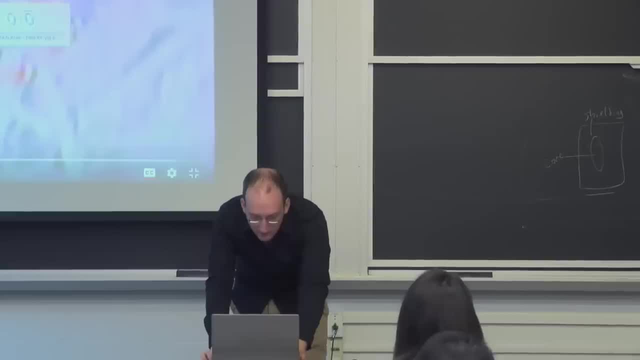 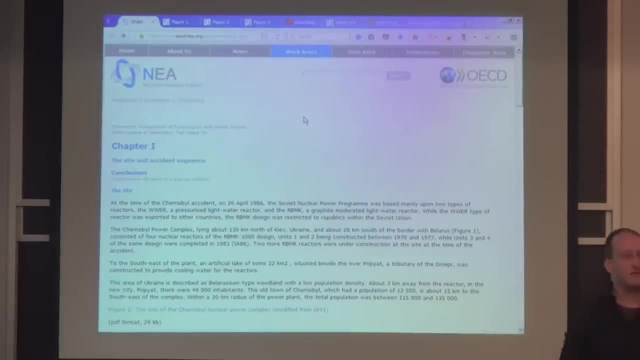 And boy were they wrong. So I want to walk you guys through a chronology of what actually happened at the Chernobyl reactor, which you guys can read on the NEA, or Nuclear Energy Agency website, the same place that you find, Janus. 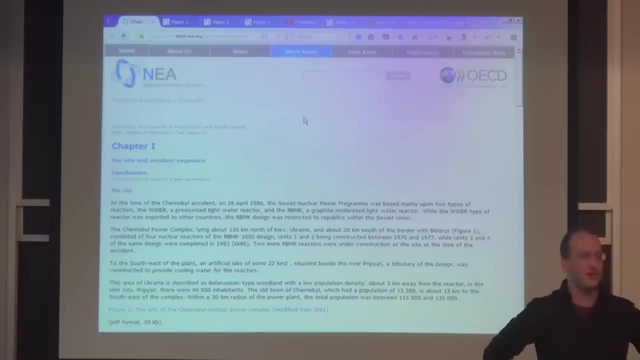 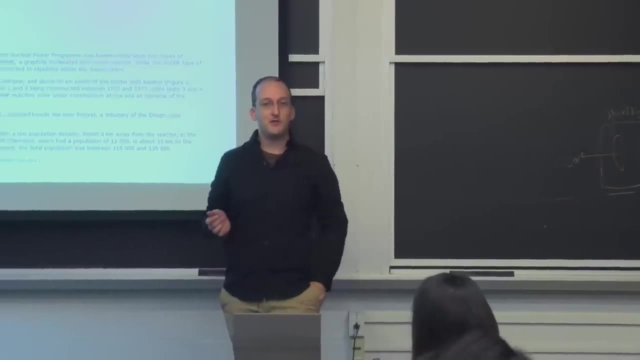 And we're going to refer to a lot of the Janus cross-sections to explain why these sorts of events happened. So the whole point of what happened at Chernobyl was it was desired to see if you could use the spinning-down turbine after you shut down the reactor. 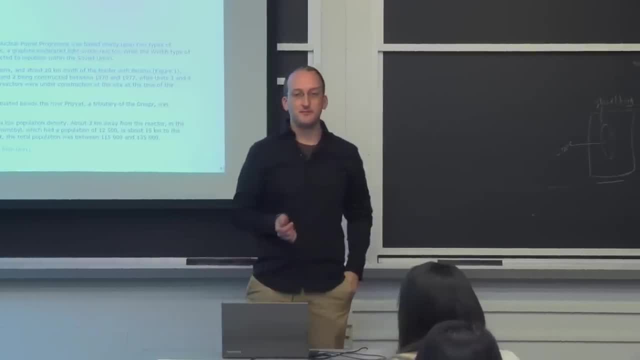 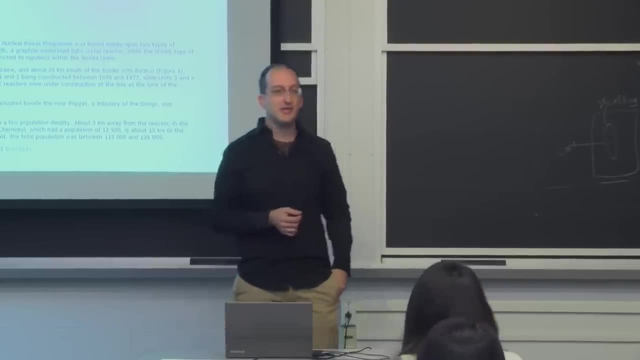 to power the emergency systems at the reactor. This would be following something what's called a loss of off-site power. If the off-site power was lost, if the off-site power or the grid was disconnected from the reactor, the reactor automatically shuts down. 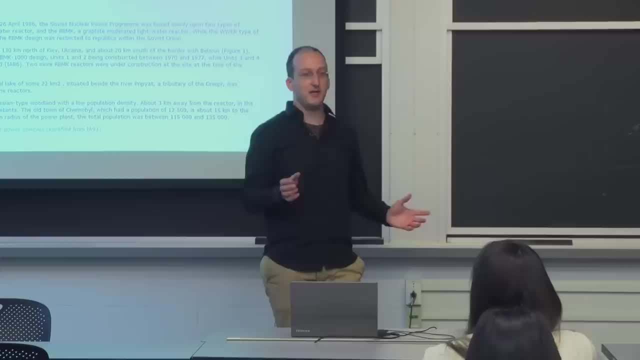 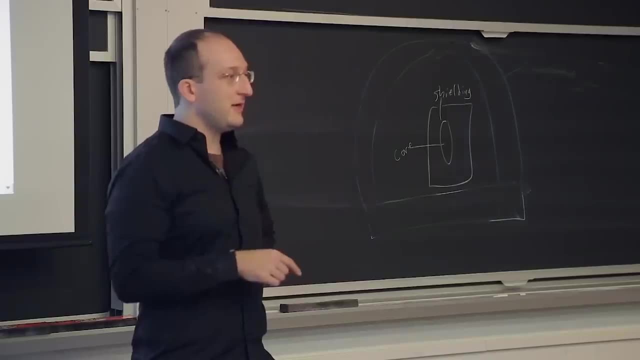 But the turbine, like I showed you a couple weeks ago, is this enormous spinning hulk of metal and machinery that coasts down over a long period of, let's say, hours. And as it's spinning, the generator coils are still spinning and still producing electricity. 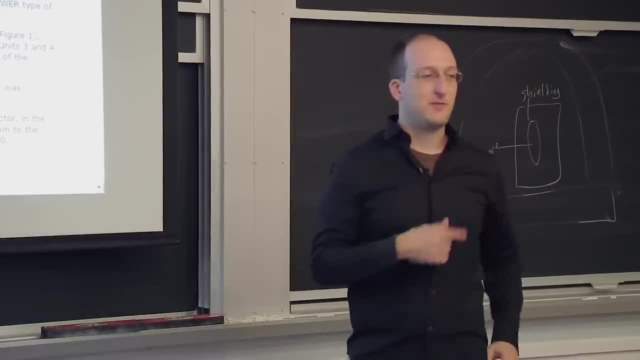 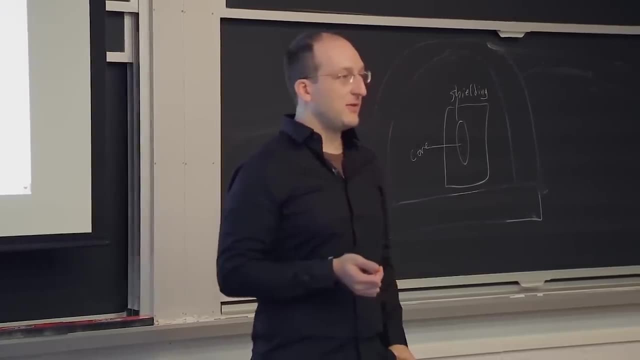 or they could be, So it was desired to find out. can we use the spinning-down turbine to power the emergency equipment if we lose off-site power? So they had to simulate this event. So what they actually decided to do is coast down the reactor to a moderate power level. 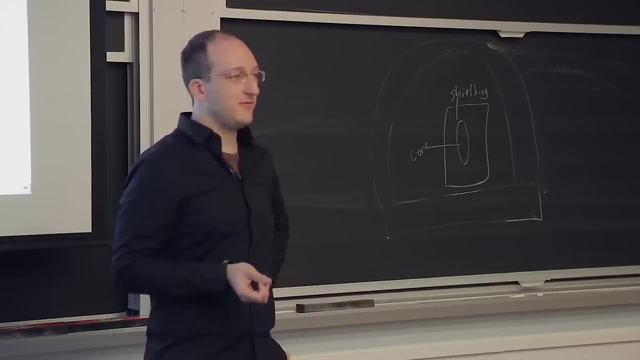 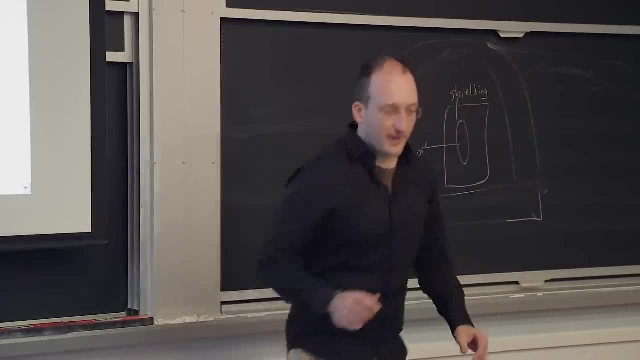 or very low power and see what comes out of the turbine itself or out of the generator, rather. Now there were a lot of flaws in the RBMK design and I'd like to bring it up here so we can talk about what it looks like. 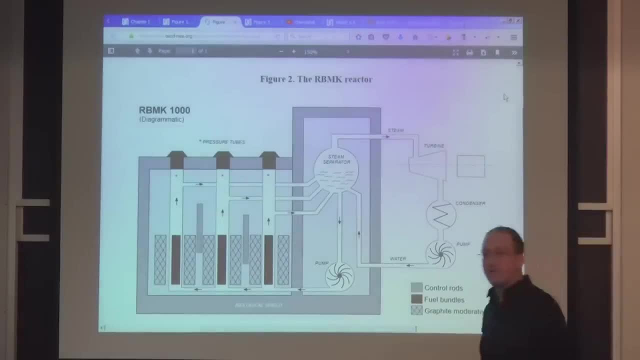 and what was wrong with it. So the RBMK is unlike any of the United States light-water reactors that you may have seen before. Many of the components are the same. There's still a light-water reactor coolant loop where water flows around fuel rods. 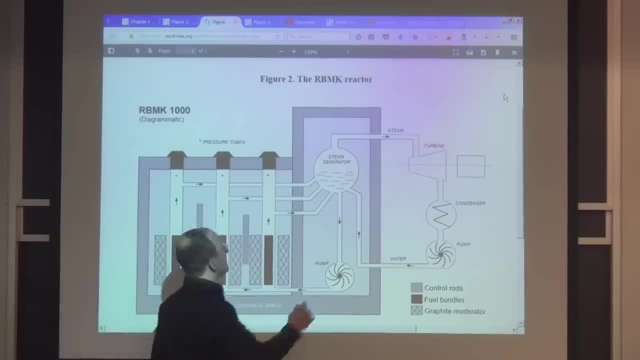 goes into a steam separator, better known as a big heat exchanger, and the steam drives a turbine which produces energy, And then this coolant pump keeps it going, and then the water circulates. What makes it different, though, is that each of these fuel rods was inside its own pressure tube. 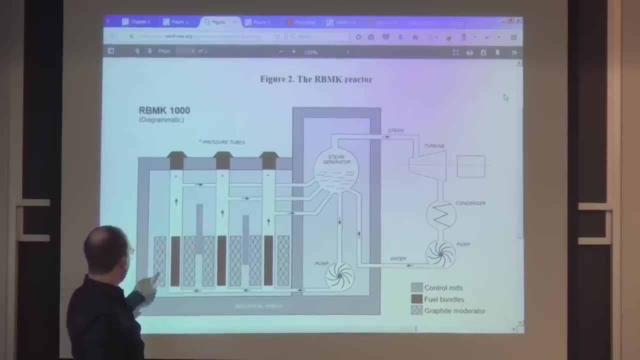 So the coolant was pressurized and out here this stuff, right here. This is a moderator composed of graphite. Unlike light-water reactors in the US, the coolant was not the only moderator in the reactor: Graphite also existed, which meant 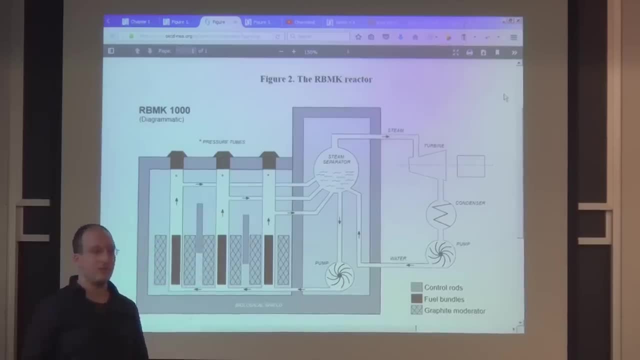 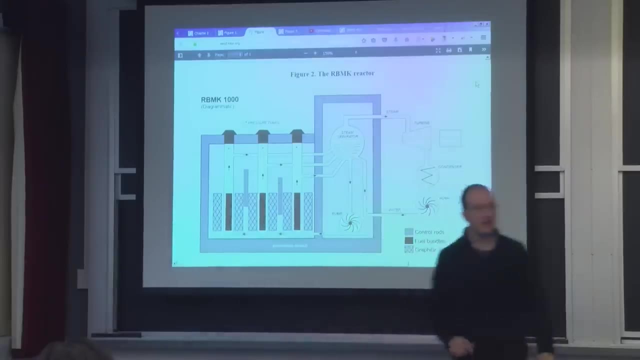 that if the water went away, which would normally shut down a light-water reactor from lack of moderation, graphite was still there to slow the neutrons down into the high fission cross-section area. And I'd like to pull up Janus and show you. 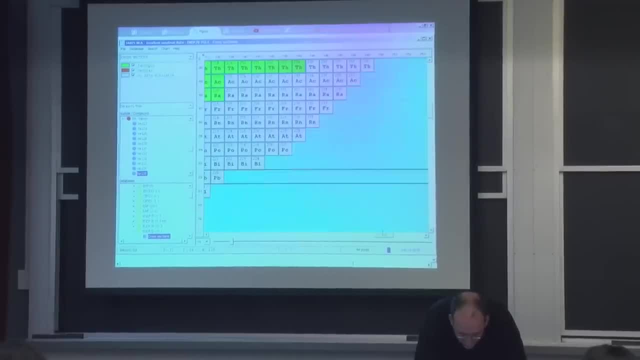 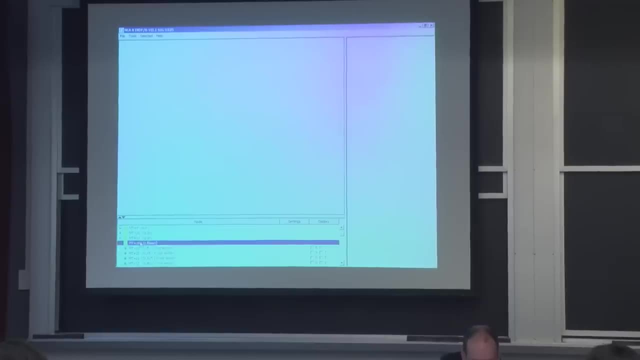 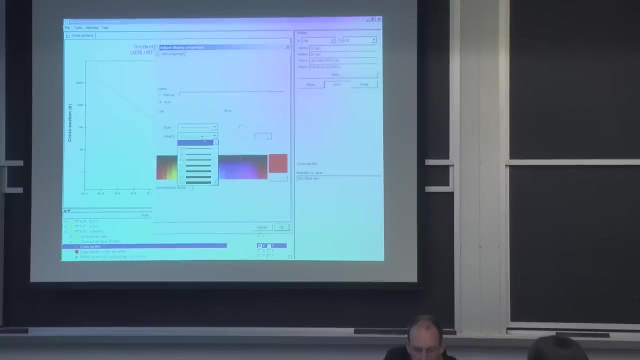 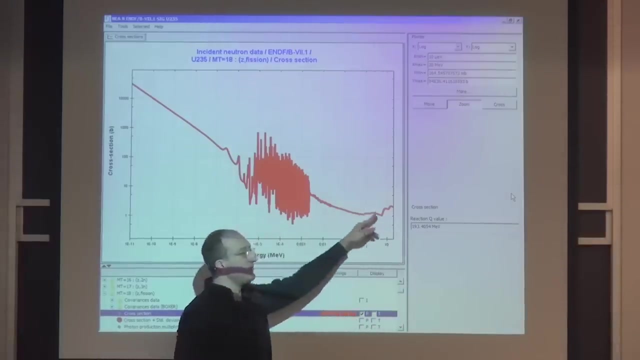 what I mean with the uranium cross-section. So let's go again to uranium-235 and pull up its fission cross-section. z fission Can make it a little thicker too. So again, the goal of the moderator is to take neutrons from high energies like 1 to 10 MeV. 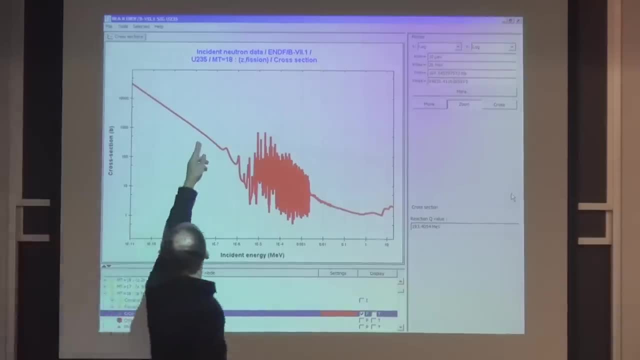 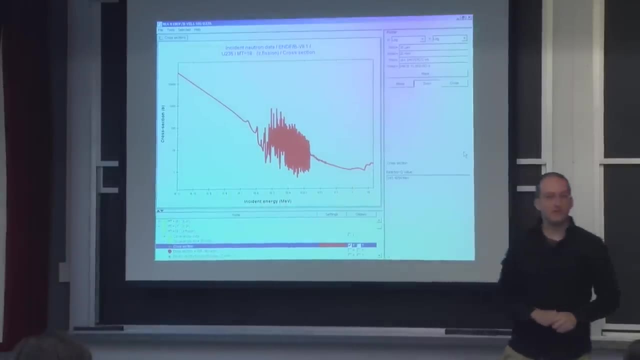 where the fission cross-section is relatively low, and slow them down into this region where fission is, let's say, 1,000 times times more likely, And in a light water reactor in the US if the coolant goes away. 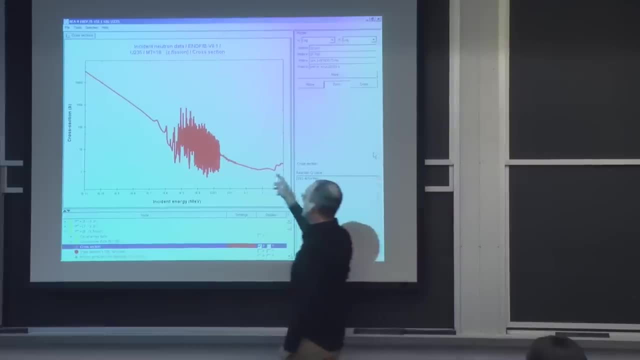 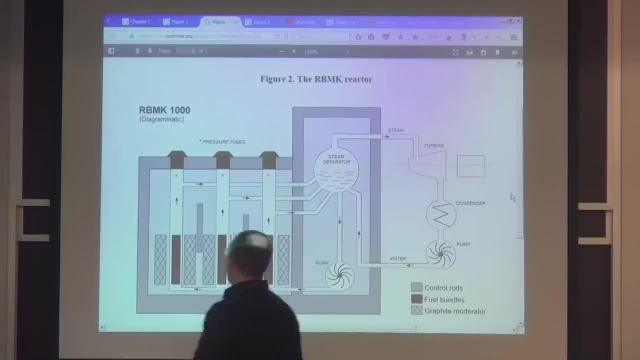 so does the moderation, And there's nothing left to slow those neutrons down to make fission more likely. In the RBMK that's not the case. The graphite's still there. The graphite is cooled by a helium-nitrogen mixture. 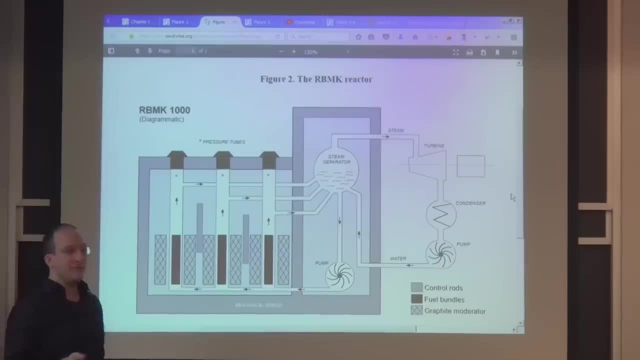 because the neutron interactions in the graphite. that's slowing down. We've always talked about what happens from the point of view of the neutron, But what about the point of view of the other material? Any energy lost by the neutrons is gained by the moderating material. 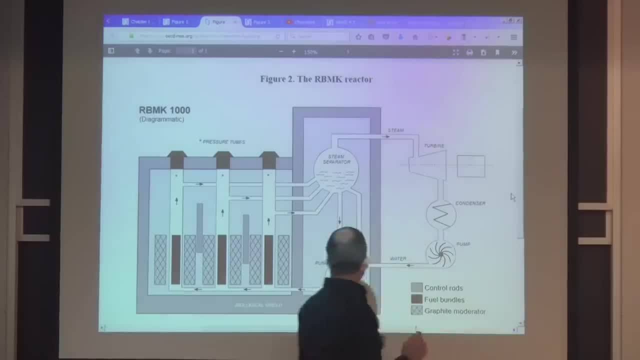 So the graphite gets really hot And you have to flow some non-oxygen-containing gas mixture like helium and nitrogen, which is pretty inert, to keep that graphite cool. And in between the graphite moderator were control rods, about 200 of them or so. 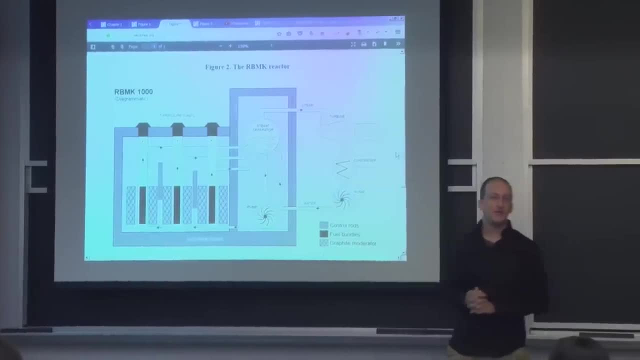 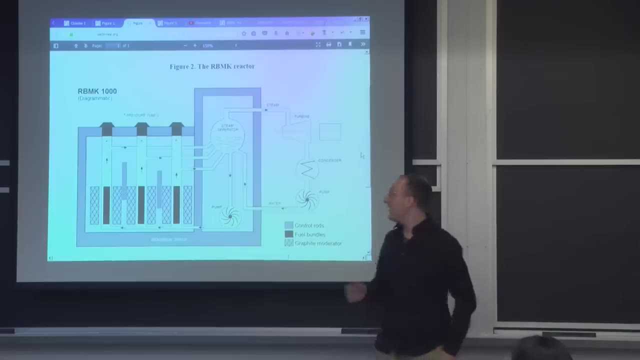 30 of which were required to be down in the reactor at any given time in order to control power, And that was a design rule that was broken during the actual experiment. And then, on top of here, on top of this biological shield, you could walk on top of it. 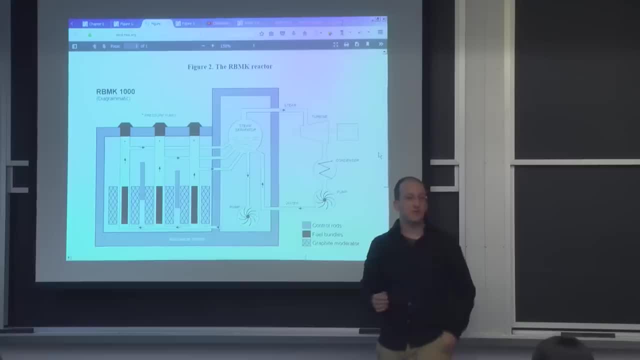 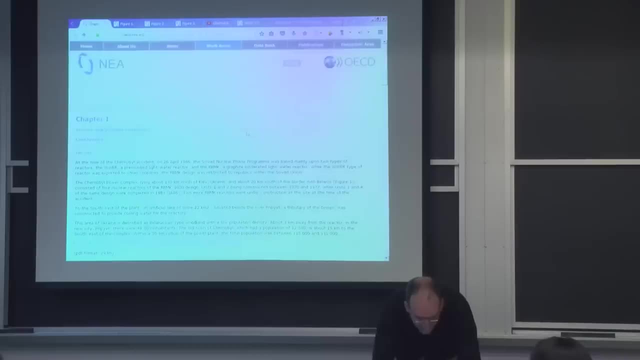 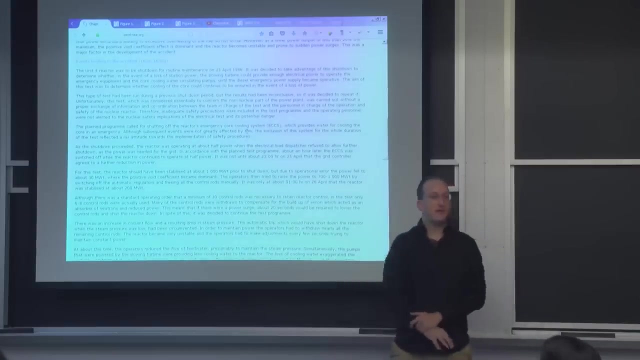 So the tops of those pressure tubes. despite being about 350 kilo chunks of concrete, you could walk on top of them. It's pretty cool. Kind of scary too. So what happened, in chronological order, was: around midnight, the decision was made to undergo this test and start. spinning down the turbine. But the grid operator came back and said: no, you can't just cut the reactor power to nothing, You have to maintain it at a rather high power for a while. about 500 megawatts electric, or half the rated power. 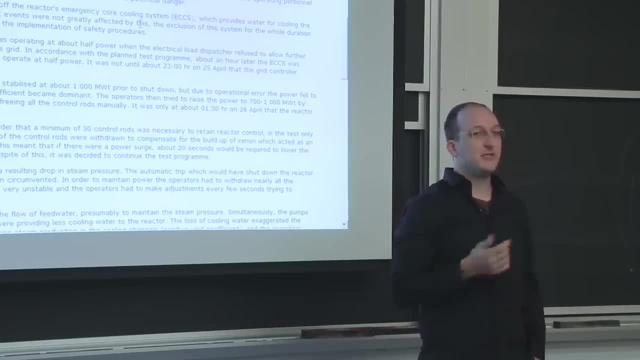 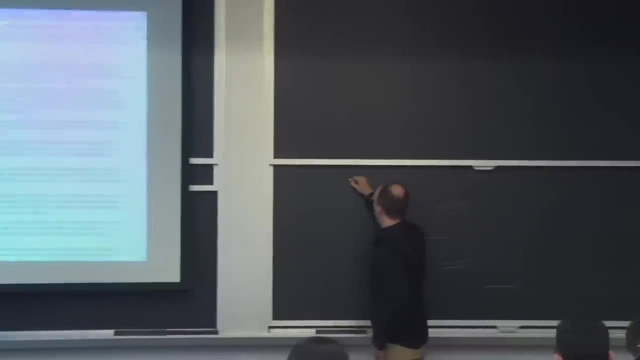 of the reactor, And what that had the effect of doing is continuing to create fission products, including xenon-135.. We haven't mentioned this one yet. You'll talk about it quite a lot in 2205, in neutron physics. 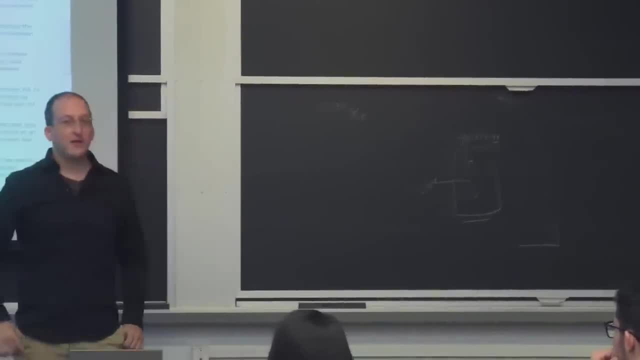 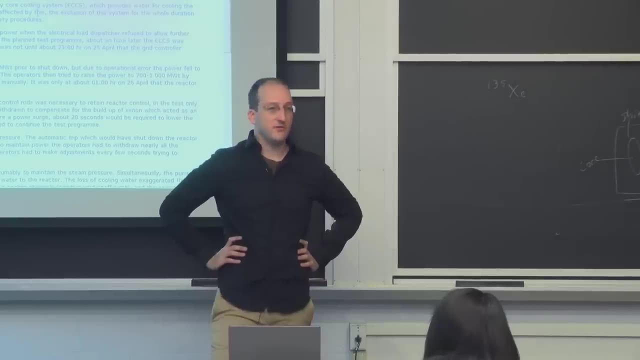 This black shirt really shows chalk. well OK, What xenon-135 does is it just sits there. It's a noble gas. It has a half-life of a few days, so it decays on the slow side as fission products go. 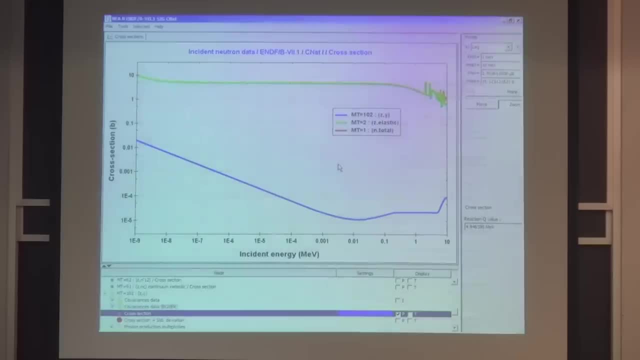 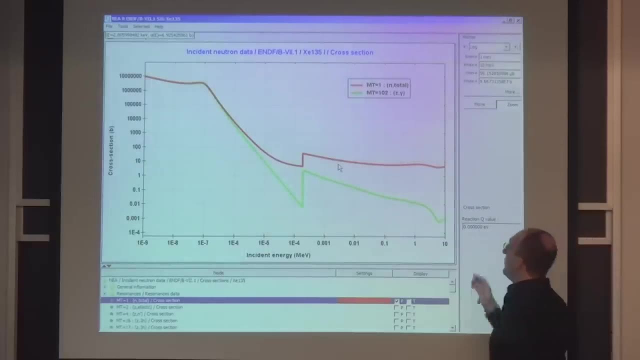 But it also absorbs lots and lots and lots of neutrons. Let's see if I can find which one is the xenon one. There we go. So here I've plotted the total cross section for xenon-135 and the absorption cross section. And notice how, for low energies, pretty much the entire cross section of xenon is made up of absorption. Did you guys in your homework see anything that reached about 10 million barns? No, Xenon-135 is one of the best neutron absorbers there is. 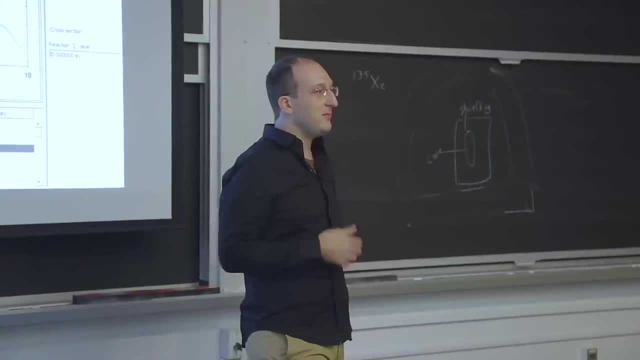 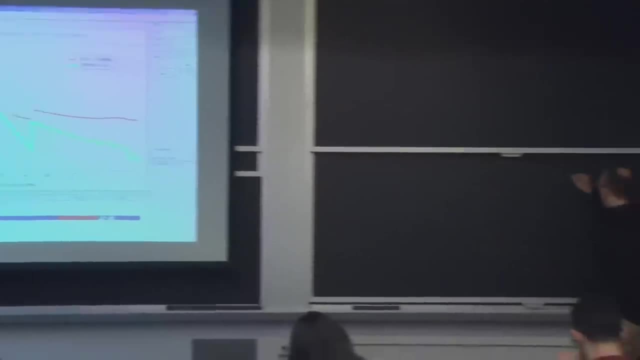 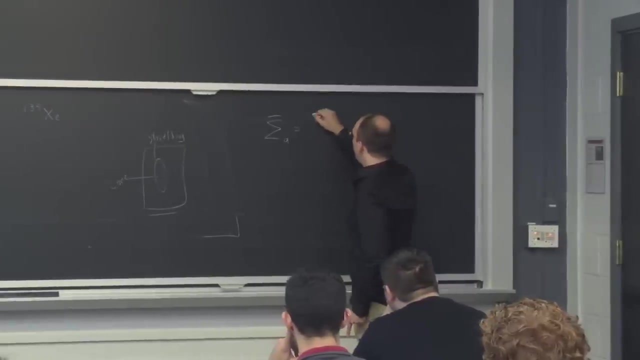 and reactors produce it constantly. So, as they're operating, you build up xenon-135 that you have to account for in your sigma absorption cross section Because, like you guys saw in the homework, if you want to write what's the sigma absorption cross section of the reactor, 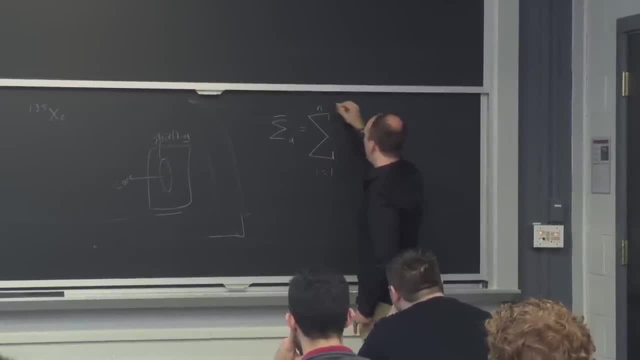 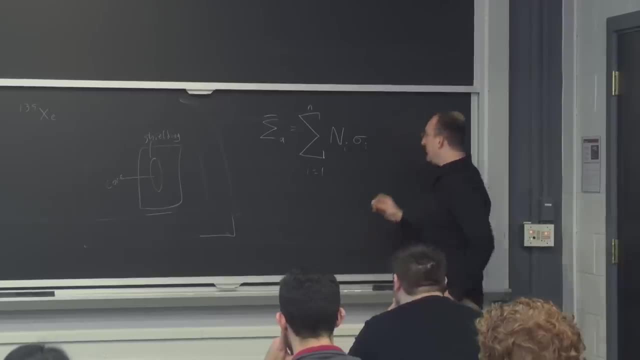 It's the sum of every single isotope in the reactor, of its number density times its absorption cross section, And so that would include everything for water and, let's say, the uranium and the xenon that you're building up When the reactor starts up. the number density of xenon is 0,. because you don't have anything to have produced it. When you start operating, you'll reach the xenon equilibrium level, where it will build to a certain level that will counteract the reactivity of the reactor And, in your K-effective expression, 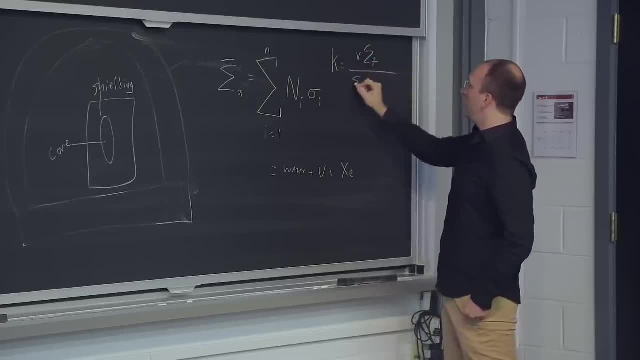 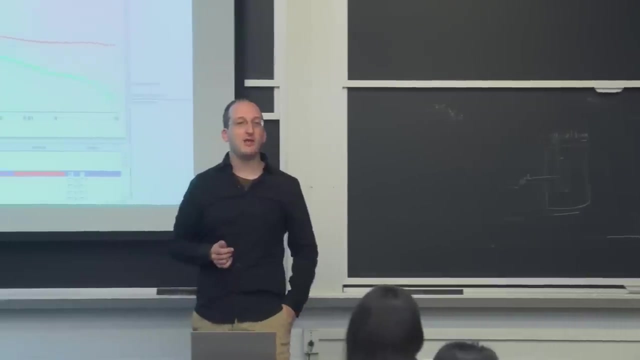 where it's sources over absorption plus leakage. this has the effect of raising sigma absorption and lowering K-effective. The trick is it doesn't last for very long. It both decays. It starts with a half-life of about five days And when you try and raise the reactor power. 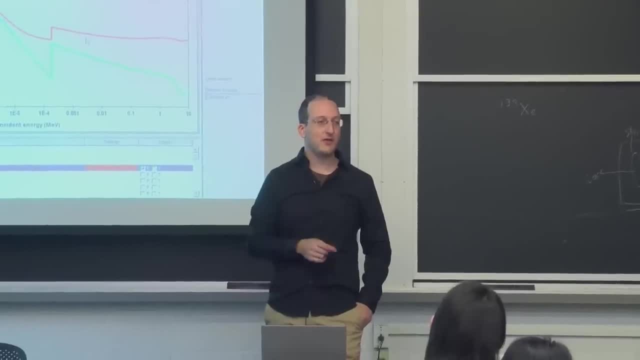 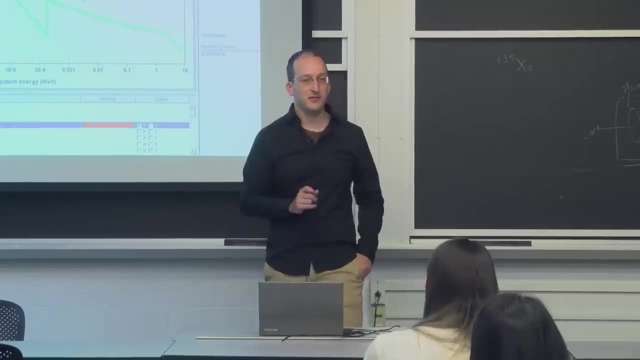 you will also start to burn it out. So if you're operating at a fairly low power level, you'll both be decaying and burning xenon without really knowing what's going on. And that's exactly what happened here. So an hour or so later, let me pull up the chronology again. 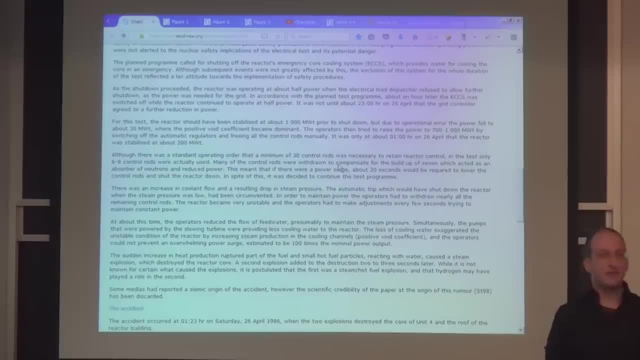 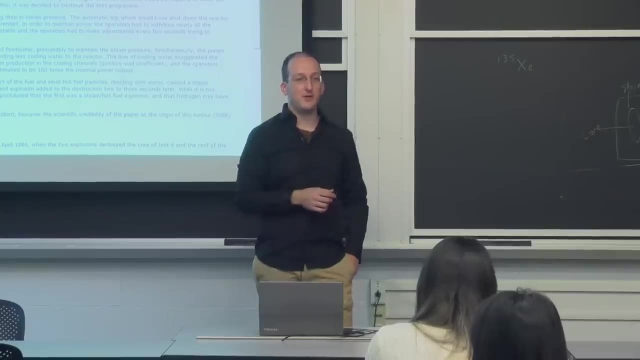 A little more than an hour later. so the reactor power stabilized at something like 30 megawatts And they were like: what is going on? Why is the reactor power so low? We need to increase it. We need to increase the reactor power. So what did they do? A couple of things. One was remove all but six or seven of the control rods, going way outside the spec of the design, because 30 were needed to actually maintain the reactor at a stable power, All the while the xenon that had been building up. 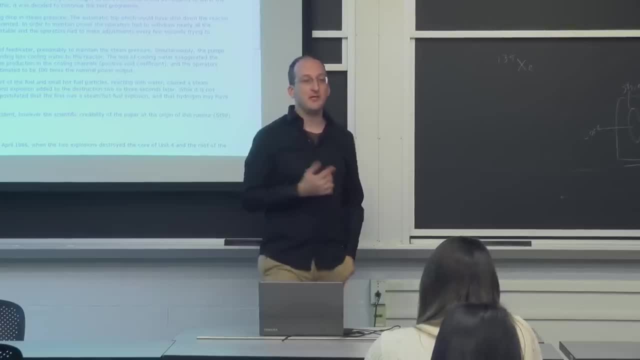 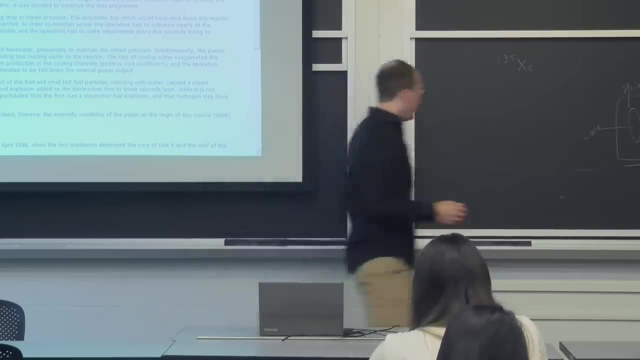 is still there, keeping the reactor from going critical. It's what was the main reason that the reactor didn't even have very much power, But it was also burning out at the same time, And so we were able to show a graph of two things. 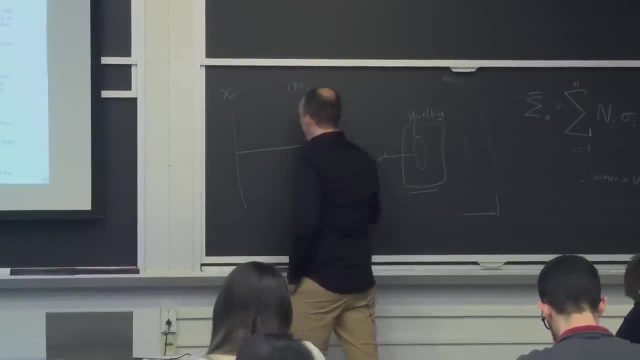 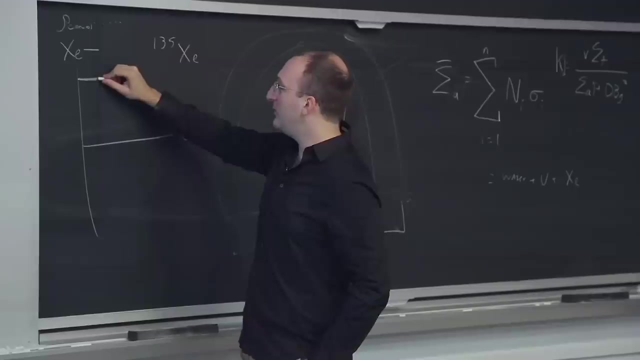 Time, xenon inventory and as a solid line and, let's say, control rod worth. as a dotted line, The xenon inventory at full power would have been at some level And then it would start to decay and burn out. Well, at the same time, the control rod worth. 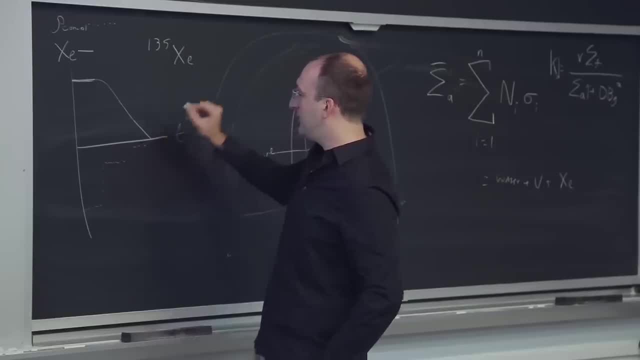 as you remove control rods from the reactor, it would start to decay. So this is the graph, This is the graph. This is the reactor. Every time you remove one, you lose some. control rod worth would continue to diminish, leading to the point: 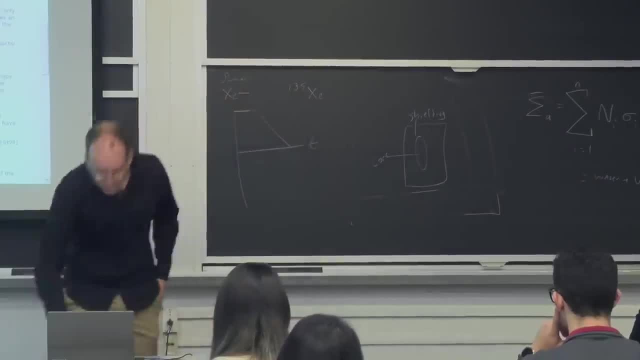 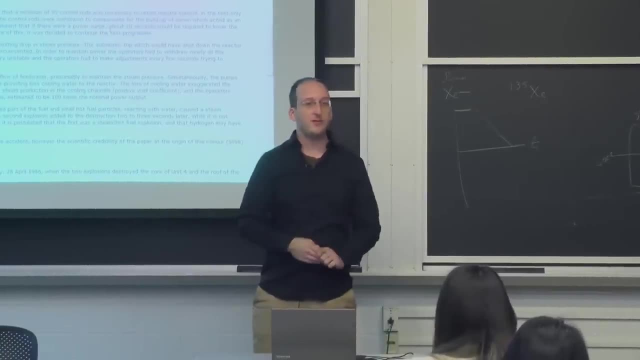 where bad stuff was going to happen. Let me make sure I didn't lose my place. So, at any rate, as they started pulling the control rods out, a couple of interesting quirks happened in terms of feedback. So let's look back at this design. 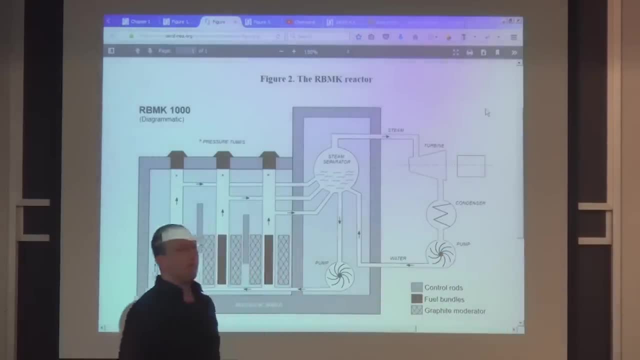 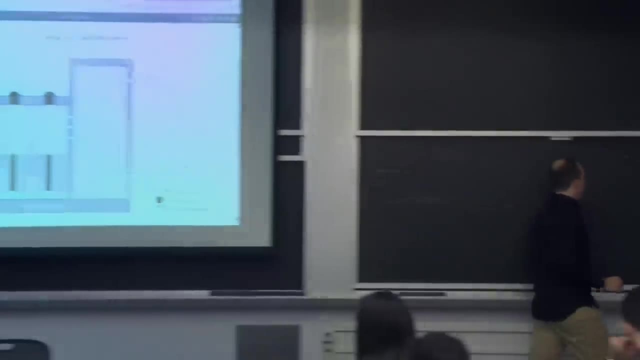 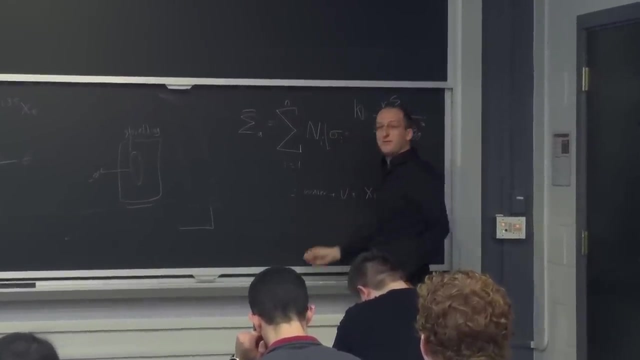 Like any reactor, this reactor had what's called a negative fuel temperature coefficient. What that means It's that when you heat up the fuel, two things happen. One, the cross-section for anything- absorption or fission- would go up, but the number density would also go down. 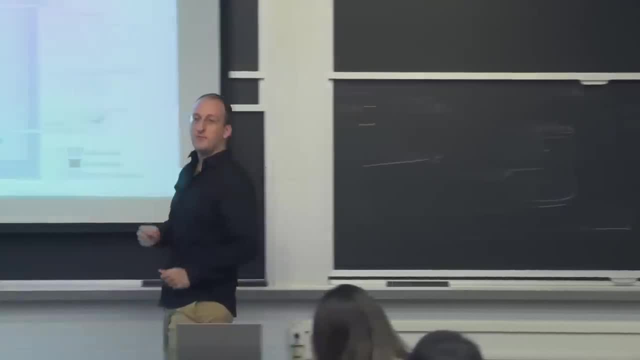 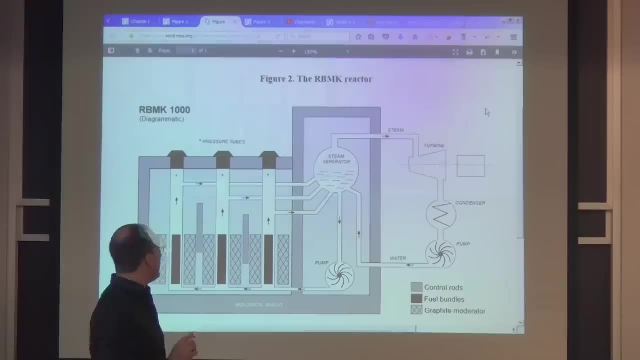 As the atoms physically spaced out in the fuel, their number density would go down, lowering the macroscopic cross-section for fission, And that's arguably a good thing. The problem is, at below about 20% power, the reactor had what's called a positive void coefficient, which 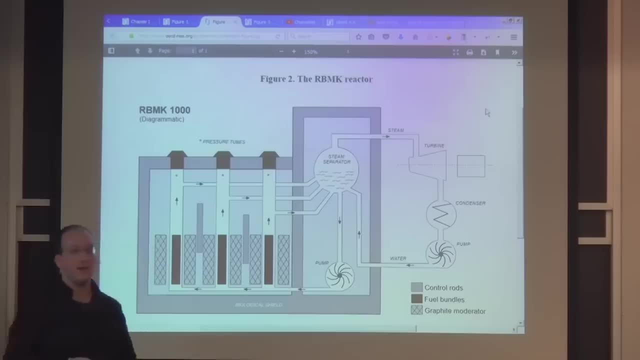 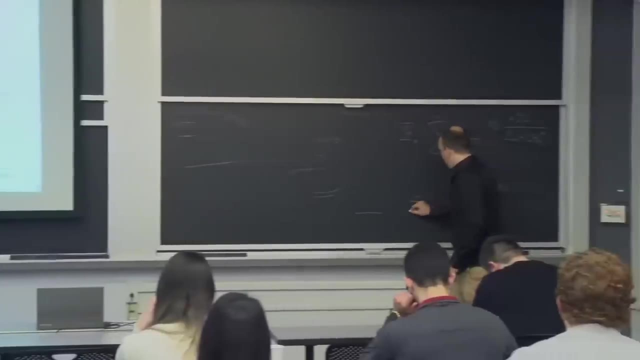 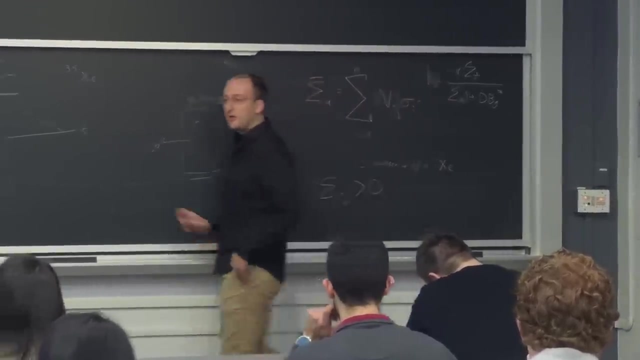 meant that If you boil the coolant, you increase the reactor power. Because the other thing that I think- I mentioned this once and you calculate it in the homework- the absorption cross-section of hydrogen is not zero. It's small but fairly significant. 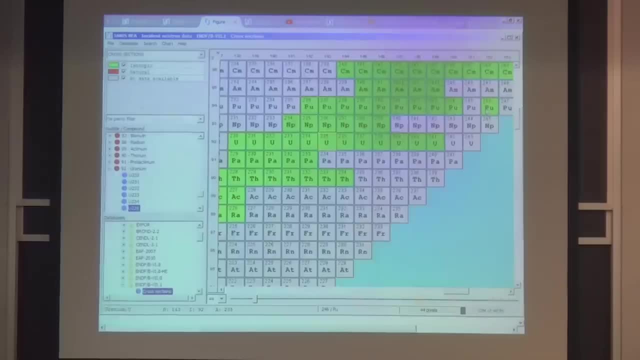 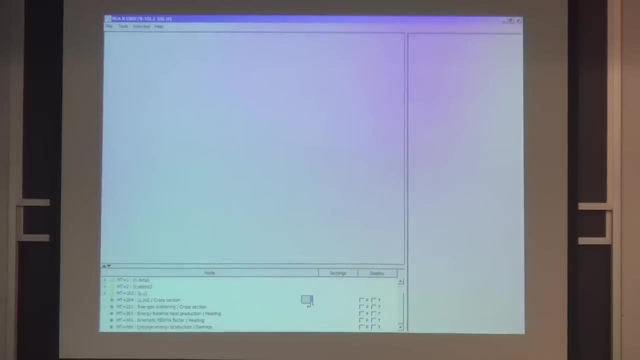 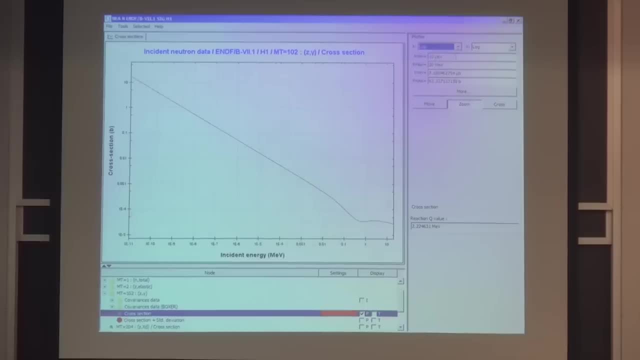 And of course it started us with a linear scale. Let's go logarithmic, Ah OK, So at low energies, 10 to the minus 8 to 10 to the minus 7, it's around a barn, Not super high but absolutely not negligible. 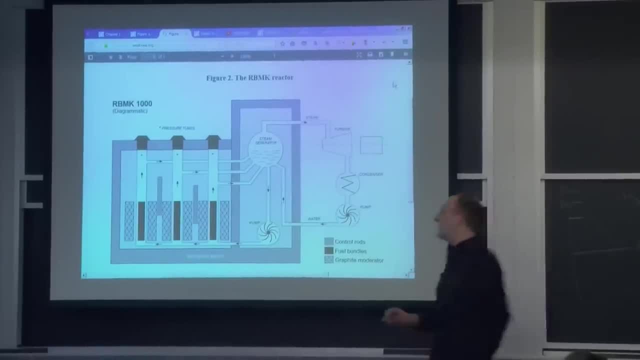 which meant that part of the normal functionality of the RBMK depended on the absorption of the water to help absorb some of those neutrons. With those neutrons gone, I'm sorry. with that water gone there was less absorption But there was still a ton of moderation. 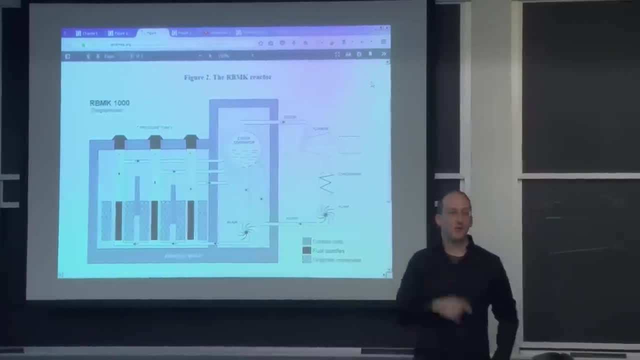 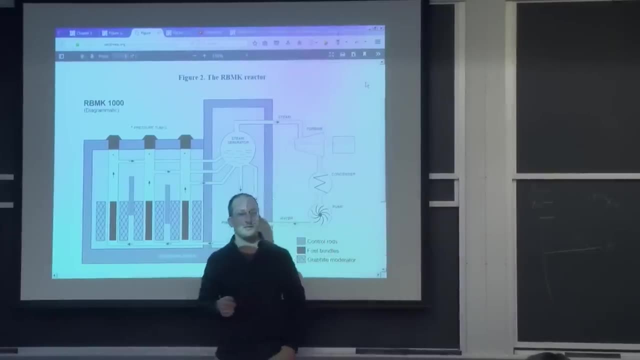 in this graphite moderator, So they still could get slow, but then there'd be more of them And that would cause the power to increase, And then that caused more of the water, the coolant to boil, which would cause less absorption, which 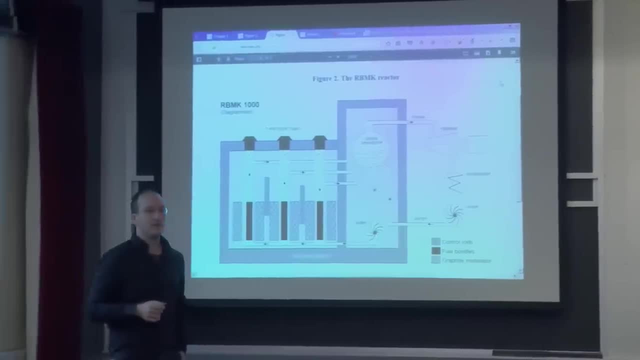 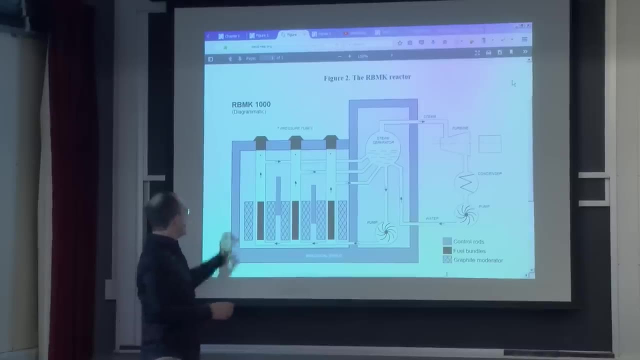 would cause the power to increase. Yeah, Charlie, So did they remove the water from the reactor? They did not remove the water from the reactor. However, as the power started to rise, the power started to rise. Some of the water started to boil. 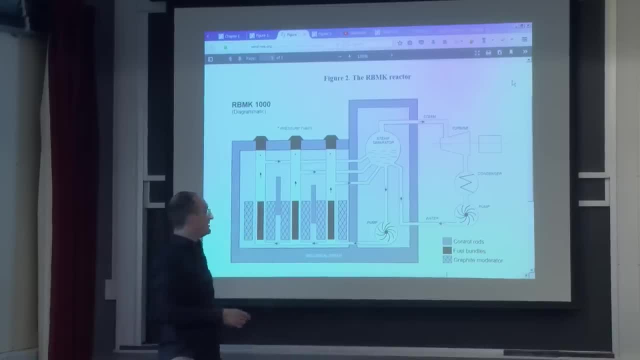 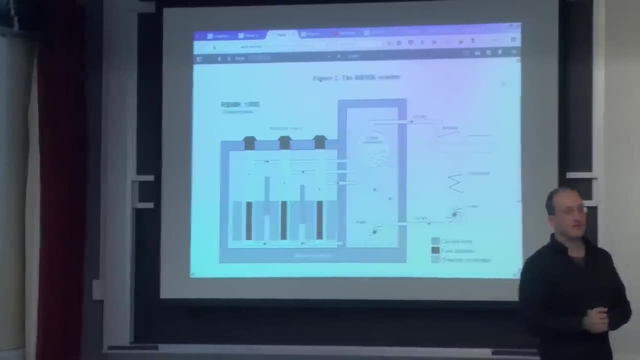 And so you can still have, let's say, steam flowing through and still remove some of the heat. However, you don't have that denser water to act as an absorber, And that's what really undid this reactor. In addition, they decided to disable the ECCS. 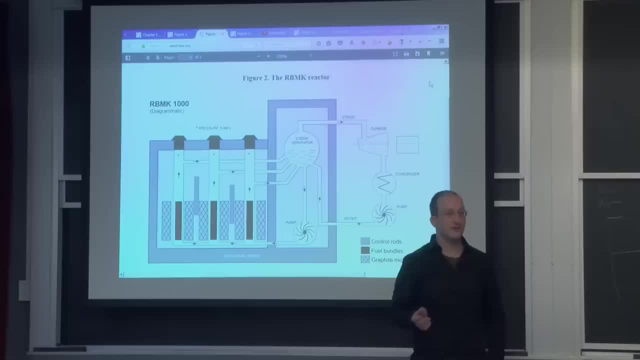 or the emergency core cooling system, which you're just not supposed to do. So they shut down a bunch of these systems to see if you could power the other ones from the spinning down turbine. And then, as they noticed that the power was going down, 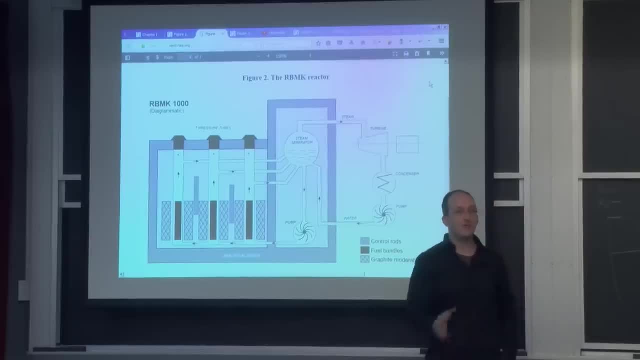 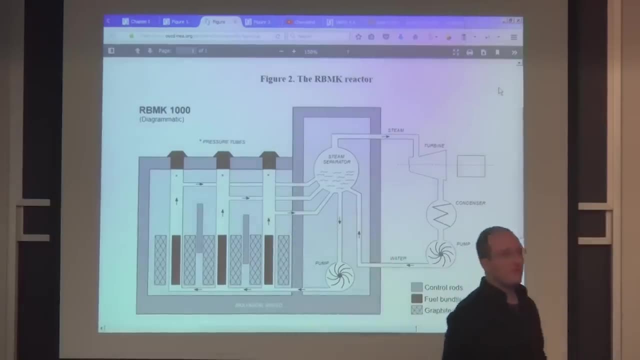 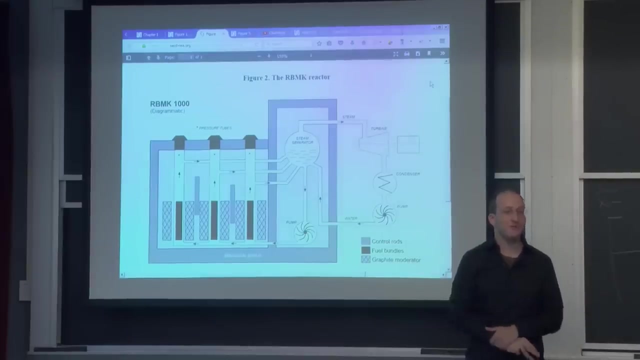 as they noticed that the reactor was getting less and less stable, they had almost all the rods out. some of these pressure tubes started to bump and jump. These 350 kilogram pressure tube caps were just rattling. I mean, imagine something that weighs, you know, 900 pounds. or so rattling around, and there's a few hundred of them. So there was someone in the control room that said the caps are rattling, What the heck? Didn't quite make it down the spiral staircase because about 10 seconds later everything went wrong. 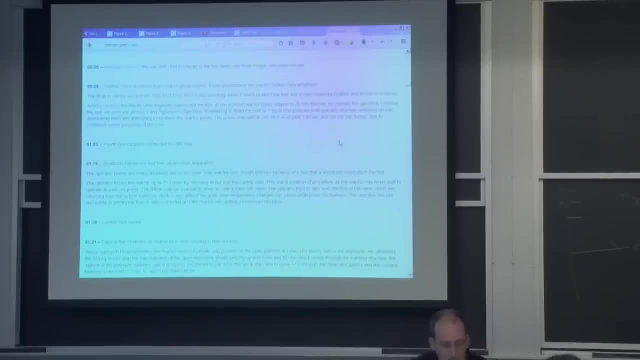 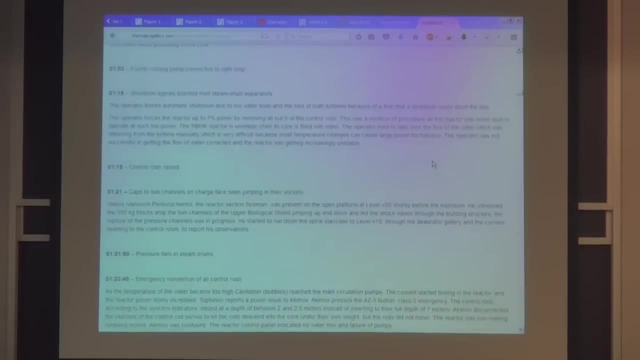 And so I want to pull up this actual timeline so you can see it splits from minutes to seconds, because the speed at which this stuff started to go wrong was pretty striking. So, for example, the control rods raised at 119 in the morning. 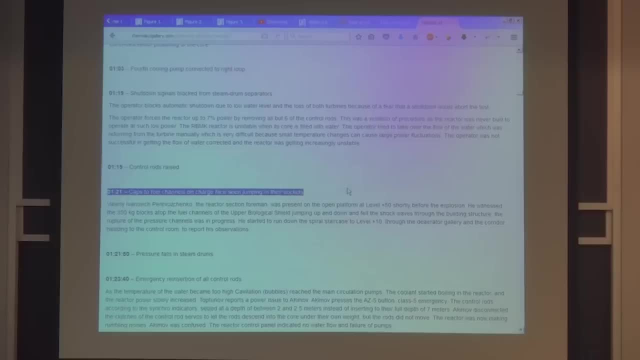 Two minutes later, when the power starts to become unstable, the caps on the fuel channels, which again are like 350 kilogram blocks, start jumping, Jumping in their sockets, And a lot of that was. we go back to the RBMK reactor. 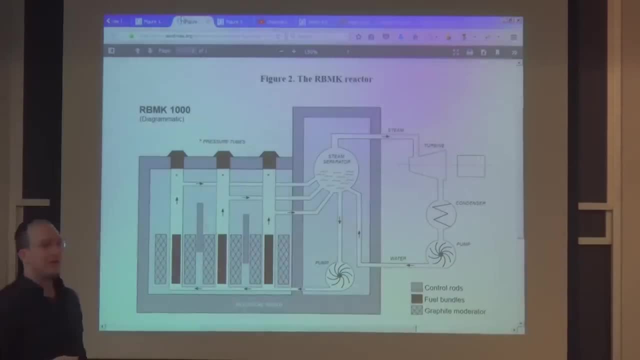 as the coolant started to boil here. well, that boiling force actually creates huge pressure instabilities, which would cause the pressure tubes to jump up and down, eventually rupturing almost every single one of them with enough force to shoot these 350 kilo caps. 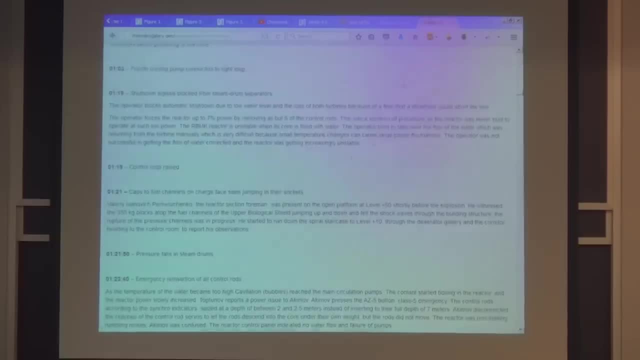 And what did they say? I like the language that they used: Jumping in their sockets. So yeah, Yeah, Yeah, Yeah, Yeah, Yeah. 50 seconds later, pressure fails in the steam drums, which means there's been some sort of containment leak. 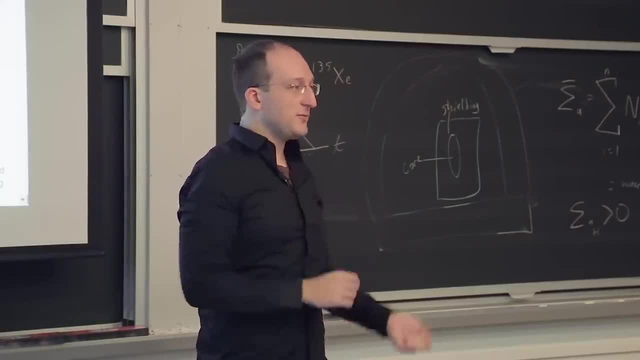 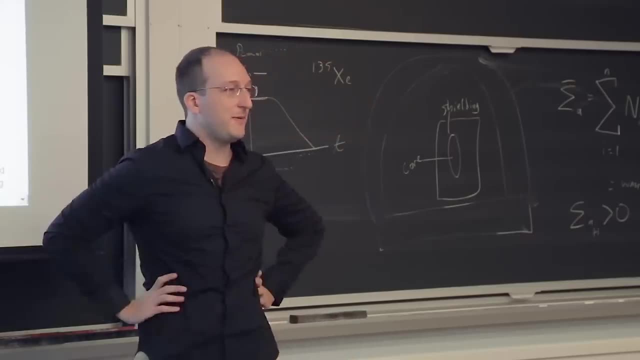 So all the while the coolant was boiling, the absorption was going down, the power was going up, repeat, repeat, repeat and the power jumped to about 100 times the rated power in something like 4 seconds. So it was normally 1,000 megawatt electric reactor. which was about 3200 megawatts thermal. It was producing nearly half a terawatt of thermal power for a very short amount of time until it exploded. Now it's interesting: a lot of folks called Chernobyl a nuclear explosion. That's actually a misnomer. A nuclear explosion would be a nuclear weapon, something set off by an enormous chain reaction, principally heated by fission or fusion. That's not actually what happened at Chernobyl, nor at Fukushima, nor was that the worry. at Three Mile Island. Not to say it wasn't a horrible thing, but it wasn't an actual nuclear explosion At first. what happened was a pressure explosion, So there was an enormous release of steam as the power built up to 100 times normal operating power. 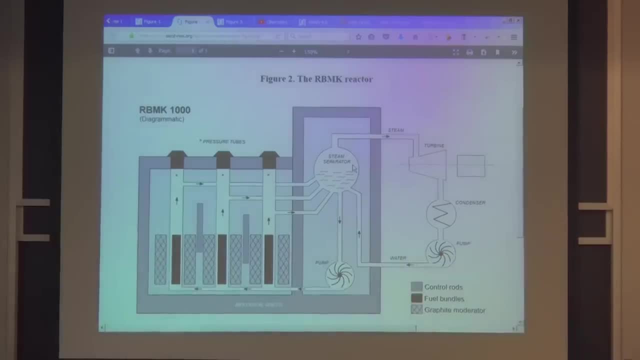 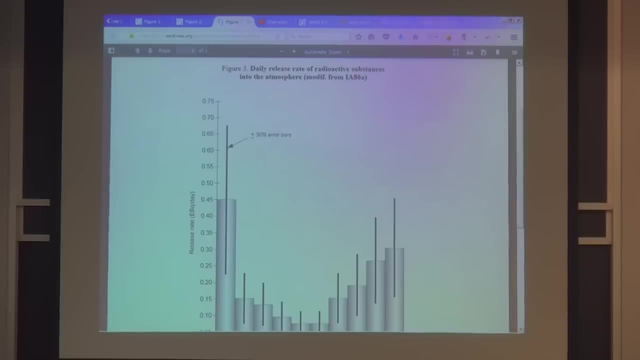 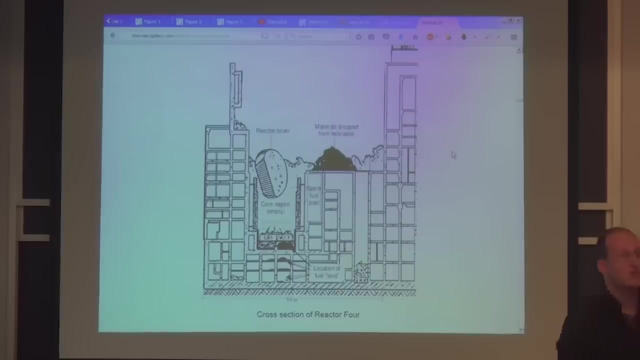 The steam force was so large that it actually blew the reactor lid up off of the thing, And I think I have a picture of that somewhere here too. It should be further down. yeah, To give you a little sense of scale. the reactor cover. which weighed about 1,000 tons, launched into the air and landed above the reactor, sending most of the reactor components up to a kilometer up in the air. Four seconds later, that was followed by a hydrogen explosion. Let me get back down to that chronology. 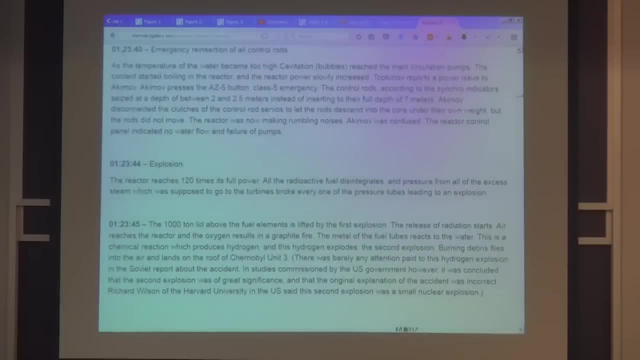 So yeah, at 1.23 and 40 seconds in the morning, oh yeah. so I should mention why this happened: Emergency insertion of all the control rods. The last part that this diagram doesn't mention is these control rods, and I'll draw this up here. 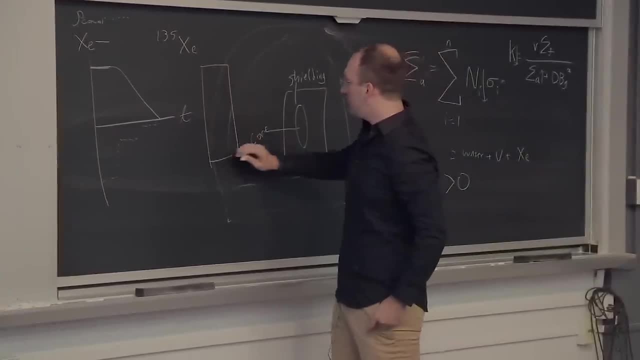 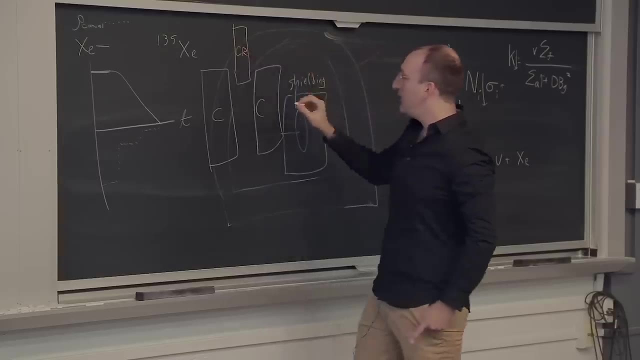 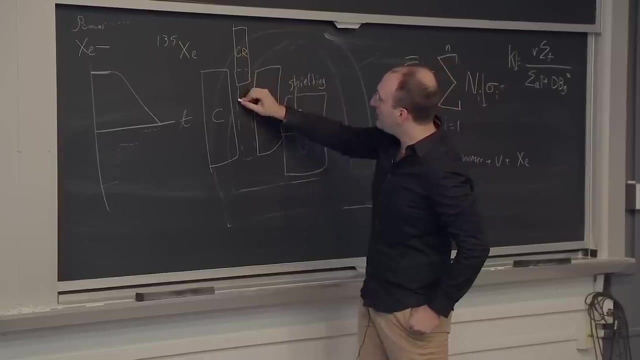 were tipped with about six inches of graphite. So if these were two graphite channels, let's say these are carbon and this is your control rod. the goal was to get this control rod all the way into the reactor. One part they didn't mention was they were tipped. 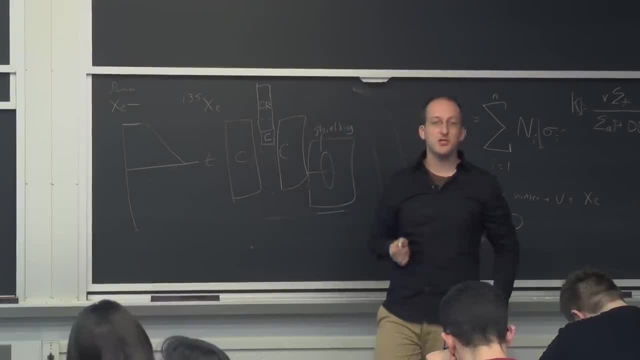 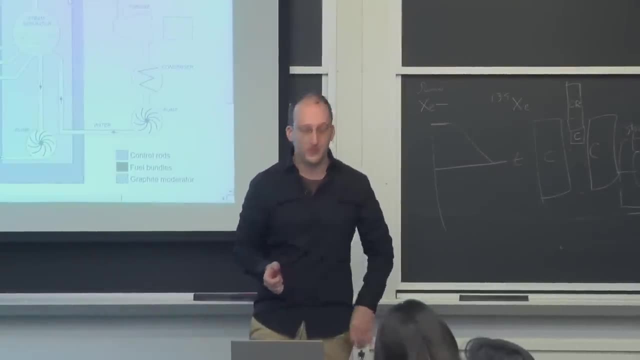 with about six inches of graphite, which only functions as additional moderator. Graphite is one of the lowest absorbers, so it's absorbing materials in the periodic table second, I think, only to oxygen, And if we pull up graphite's cross sections, 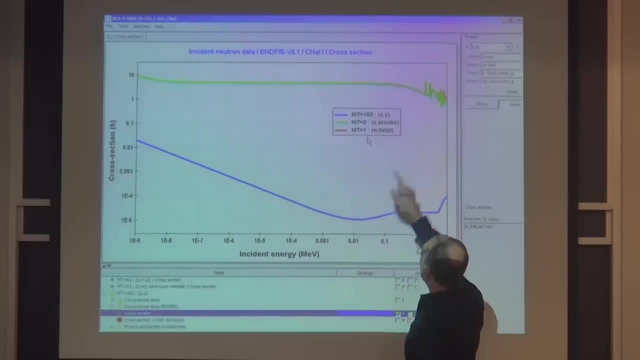 I've plotted here the total cross section, the elastic scattering cross section, and down here in the 0.001 barn level is the absorption cross section about 1,000 times lower than water. So you're shoving more material in the reactor. that slows down. 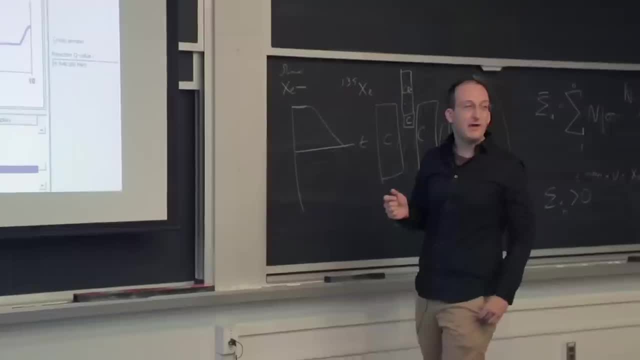 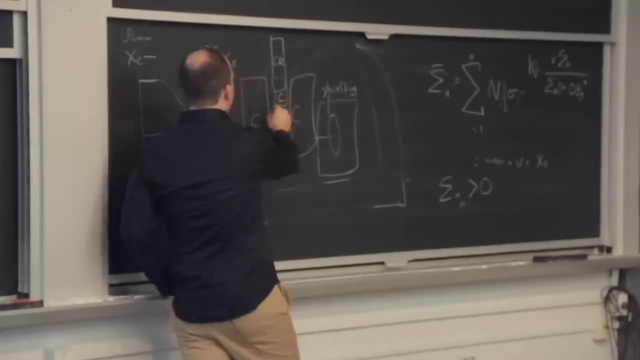 neutrons even more, bringing them into the high fission region without absorbing anything. And they jammed about halfway down, about two and a half feet down, leaving the extra graphite right in the center of the core, where it could do the most damage. And it didn't take that much time. Yeah, So my understanding is that also, one of the designs was that the control rods didn't immediately drop down, but they were slowly lowered. Yep, they took seven to 10 seconds. Okay, if they had a system where they did drop. 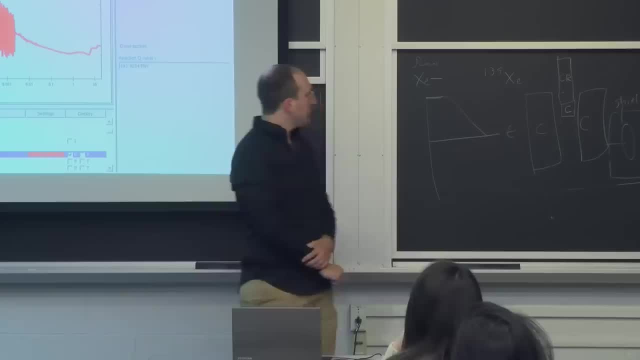 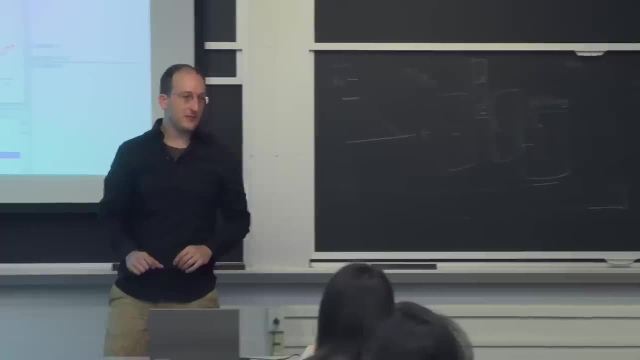 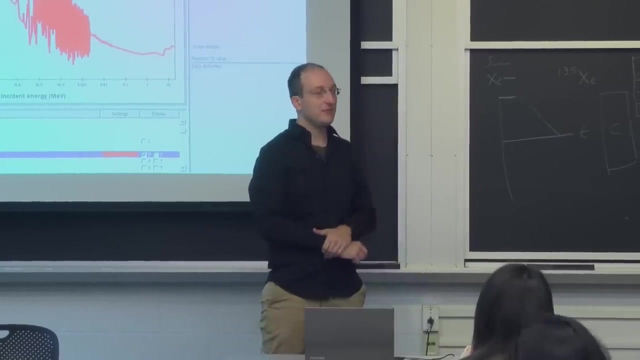 would that have possibly actually shut the system down? I'm not sure. I don't know whether lowering control rods into something that was undergoing steam explosions would have actually helped To me. by this point it was all over, So the extra moderator that was dumped in. 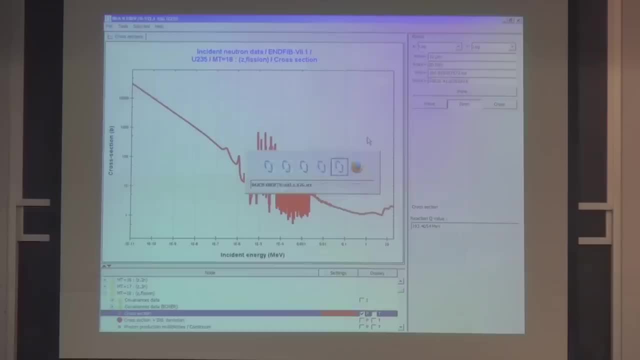 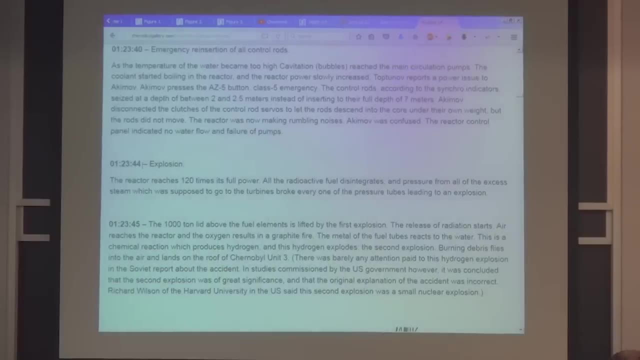 was the last kick in the pants. this thing needed to go absolutely insane. And if we go back to the timeline on the second level, control rods inserted at 1.23 and 40 seconds. explosion four seconds later, ah, to 120 times full power. 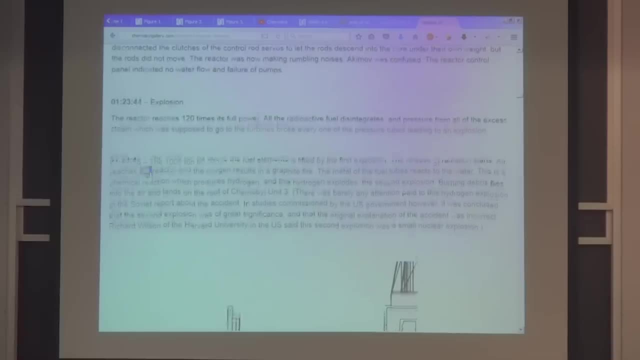 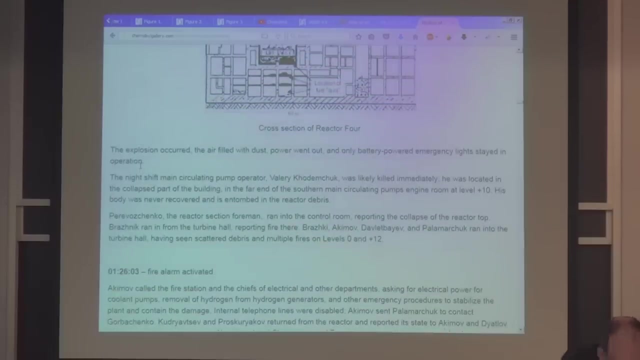 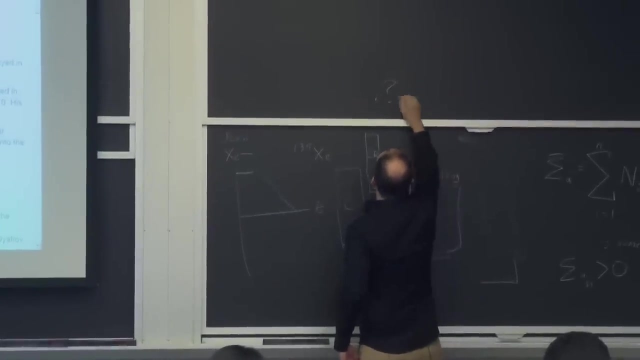 getting towards a terawatt or so. One second later, the 1,000-ton lid launches off from the first explosion Very shortly after that second explosion. And that happened because of this reaction- Well, just about anything corroding with water. will make pretty much anything: oxide plus hydrogen, The same chemical explosion that was the undoing of Fukushima and was the worry at Three Mile Island that there was a hydrogen bubble building because of corrosion reactions with whatever happened to be in the core. This happens with zirconium pretty vigorously. 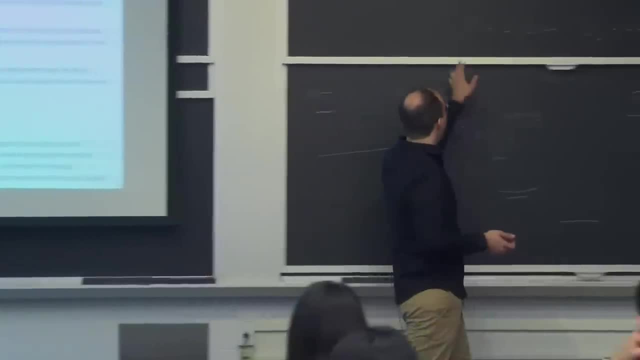 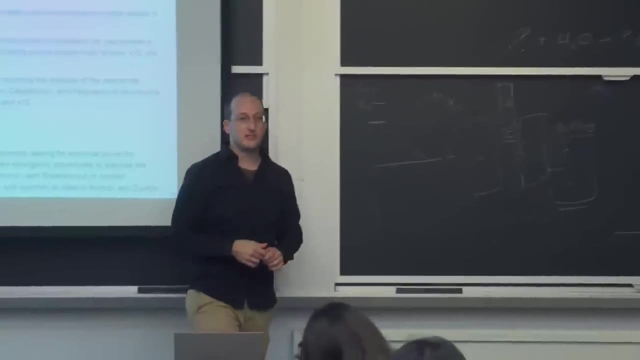 but it happens with other materials too. If you oxidize something with water, you leave behind the hydrogen, And the hydrogen in a very wide range of concentrations in the air is explosive. We're actually not allowed to use hydrogen at above 4%. 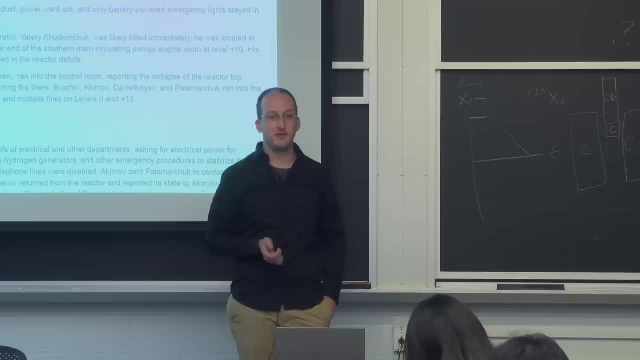 in any of the labs here because that reaches the flammability or explosive limit. OK, So we were doing some for my PhD. we were doing these experiments corroding materials in liquid lead And we wanted to dump in pure hydrogen to see what happens when there's no oxygen. 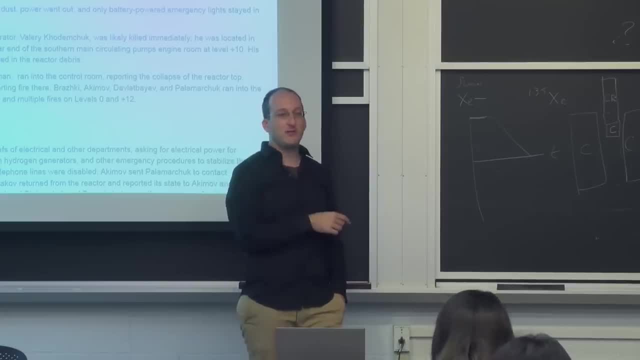 We were told absolutely not. We had to drill a hole in the side of the wall so that the hydrogen would vent outside and do some calculations to show if the entire bottle of hydrogen emptied into the lab at once, which it could do if the cap of the bottle breaks off. 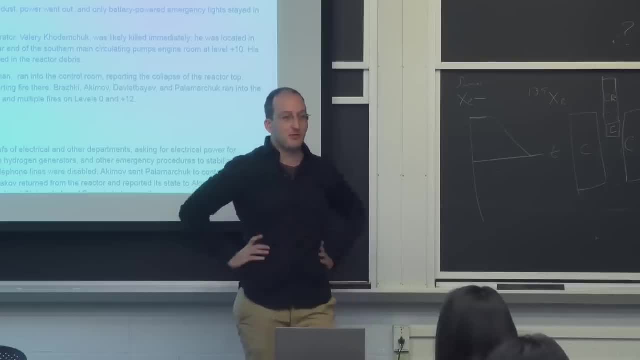 it would not reach 4% concentration. So hydrogen explosions are pretty powerful things. Have you guys ever seen people making water from scratch? Mix hydrogen and oxygen in a bottle and light a match. We've got a video of it circulating somewhere around here. because for RTC, for the reactor technology course, 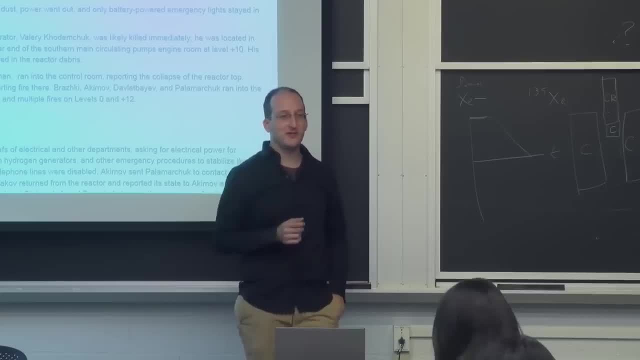 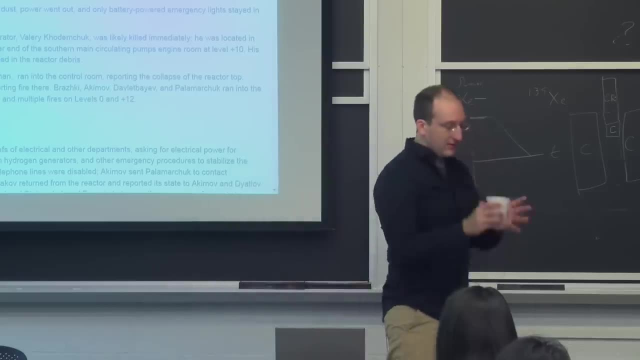 I do this in front of a bunch of CEOs. Watch them jump out of their chairs to teach basic chemical reactions. But it's pretty loud About enough hydrogen and oxygen to just fill this cup or fill a half liter water bottle. makes a bang that gets your ears ringing- not quite bleeding. but close enough. Close enough. So that's what happened here, except on a much more massive scale. So there was a steam explosion, followed seconds later by a hydrogen explosion from hydrogen liberated from the corrosion reaction of everything with the water that was already there. 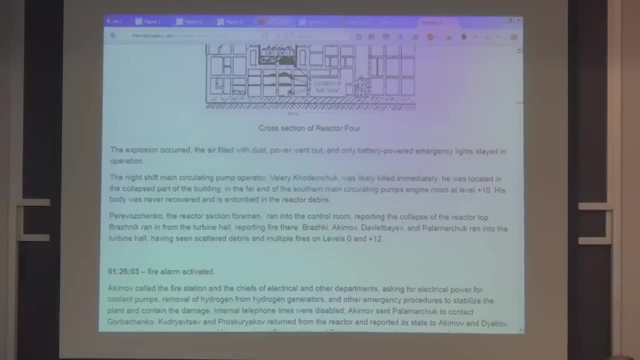 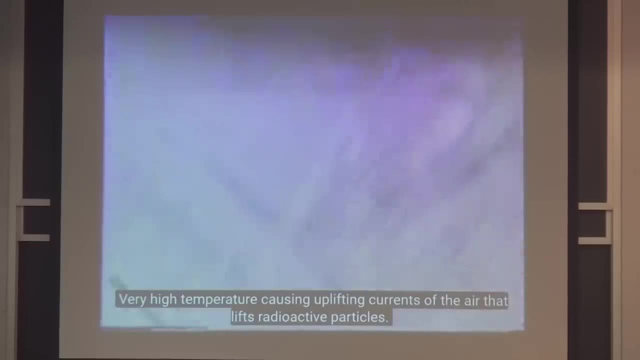 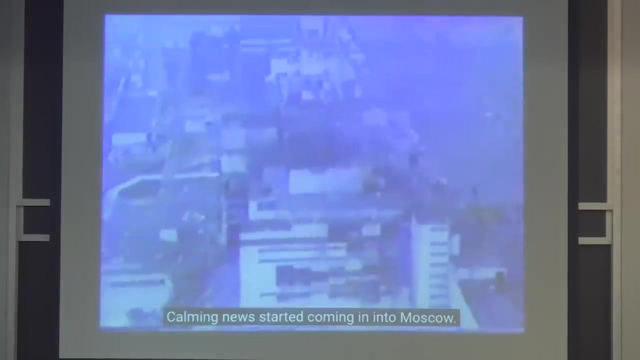 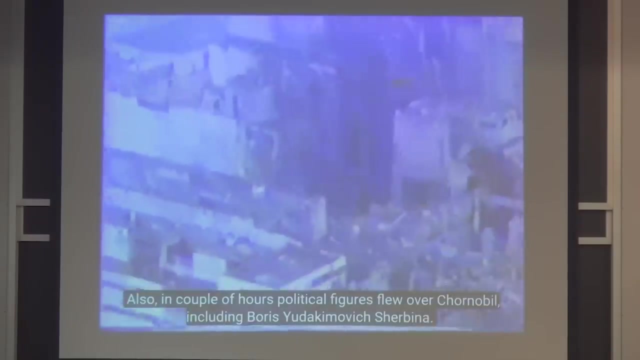 And that's when this happened. So that smoke right there it's from a graphite fire, not normal smoke. 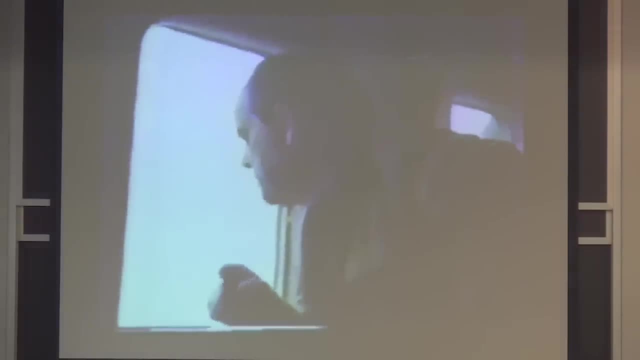 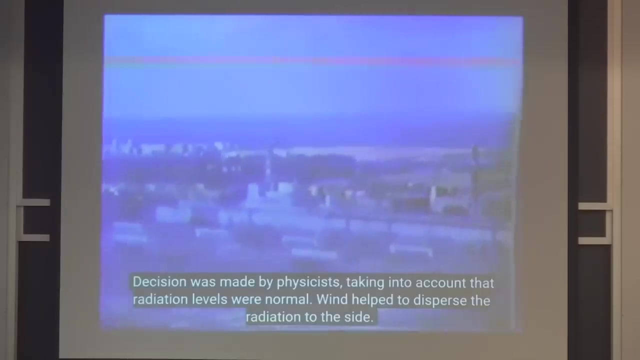 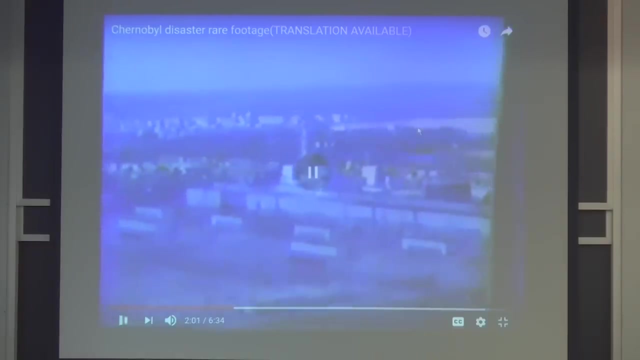 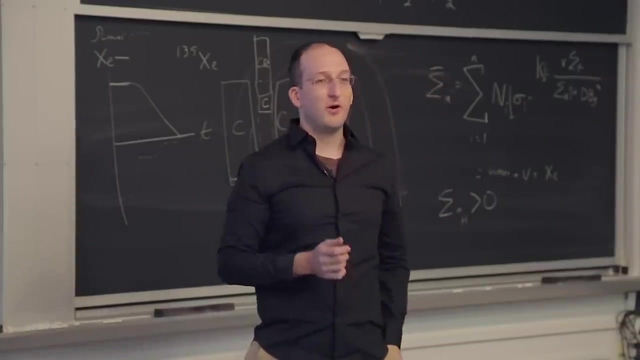 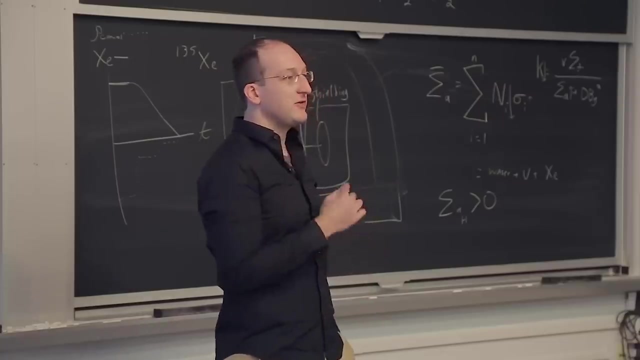 feedback and criticality, you can start to understand why Chernobyl was flawed. 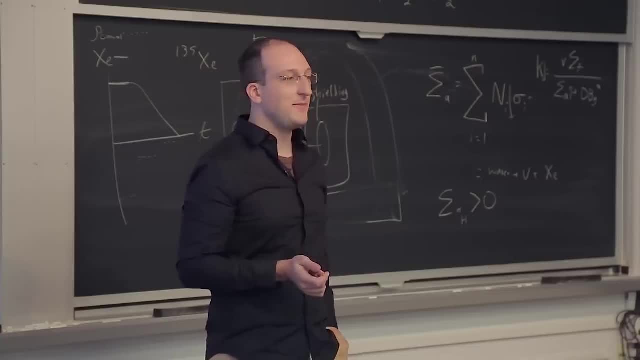 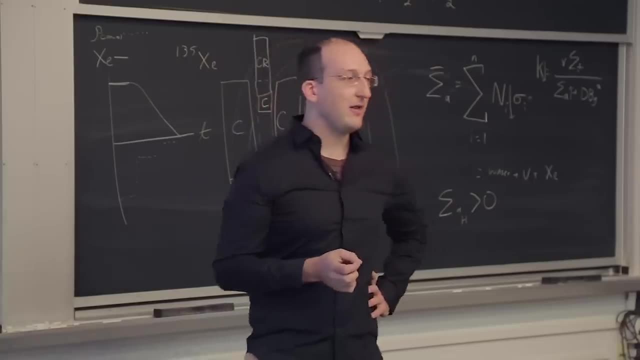 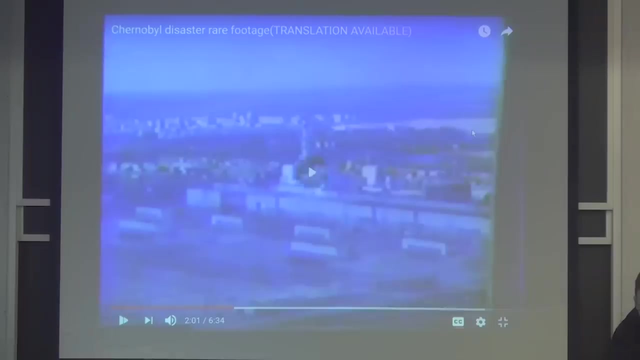 in this design and what we're going to teach you in the rest of the course is what happens next, what happens when radionuclides are absorbed by animals of the human body and what was the main fallout, let's say in the in the colloquial sense and the actual sense- from the Chernobyl reactor. let's look a. 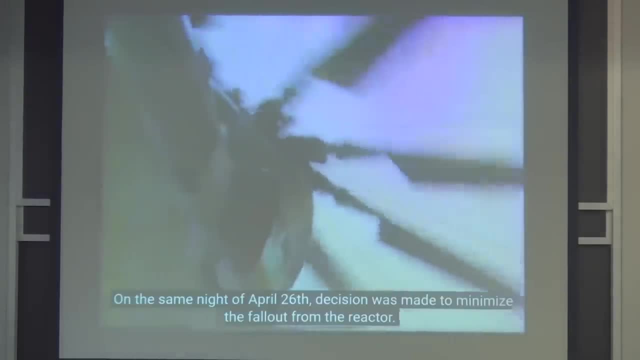 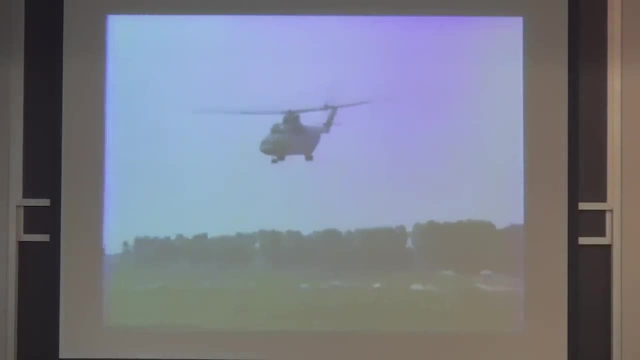 bit. what they did next, though? all this was on the reactor's burning gas: 22 flights and 30 tons of cargo per day for each. the highest skill was required, not only for the cargo to reach the target of the burning graphite. every extra minute in the area of the 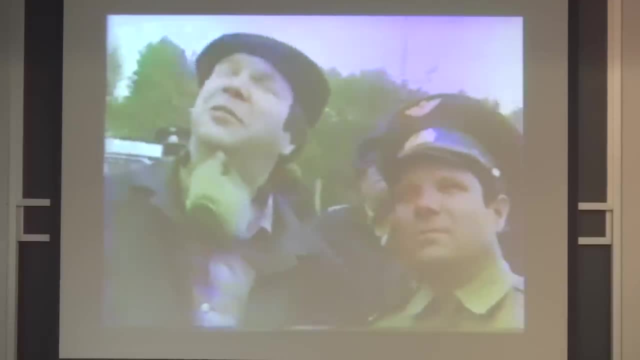 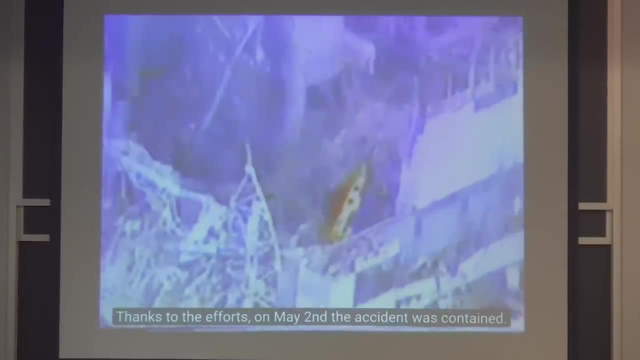 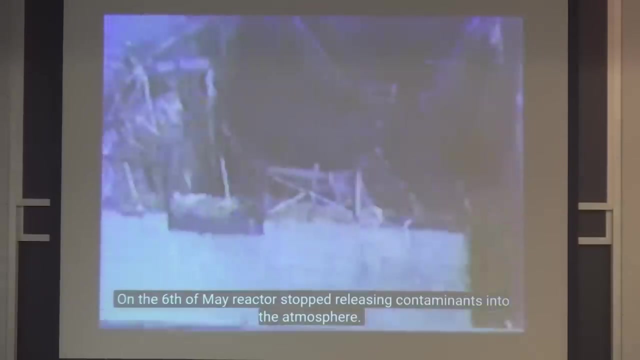 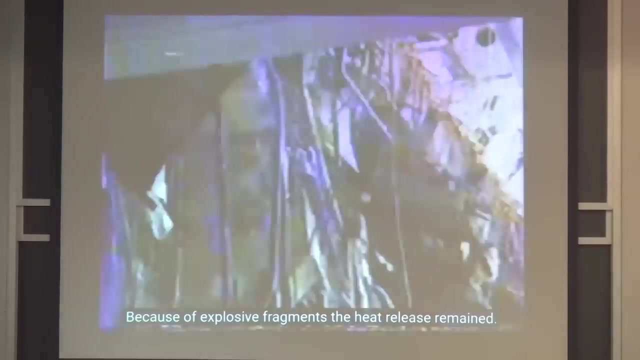 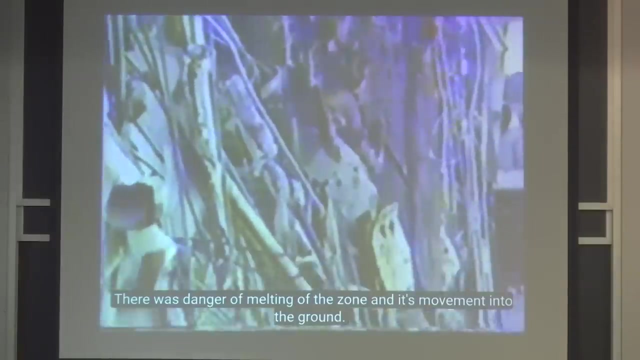 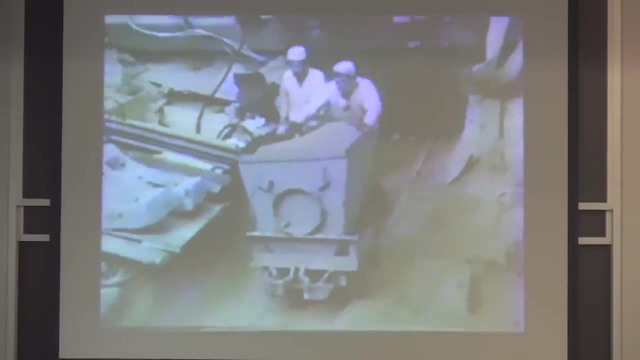 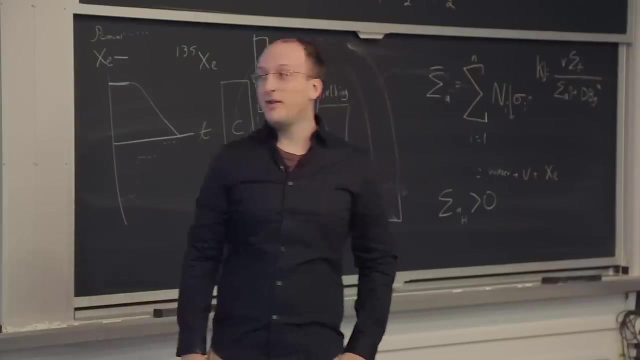 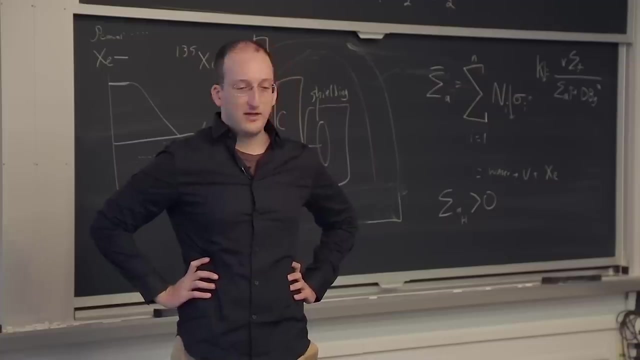 primordial and active fire threatened health thanks to this action already on May 2. that's not quite true. you'll see why that actually did happen- makes no sense. I think that pretty much summarizes the state of things now. the yā: they built a sarcophagus around this reactor, a gigantic tomb which, according to some, 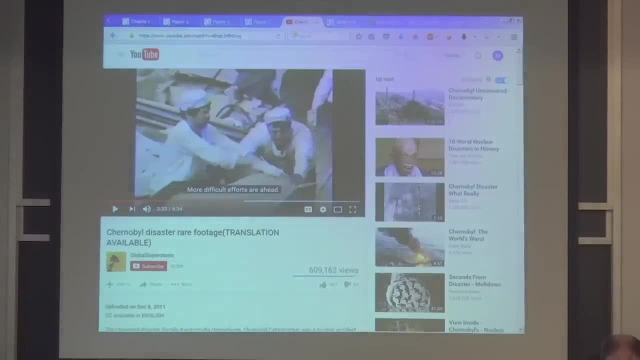 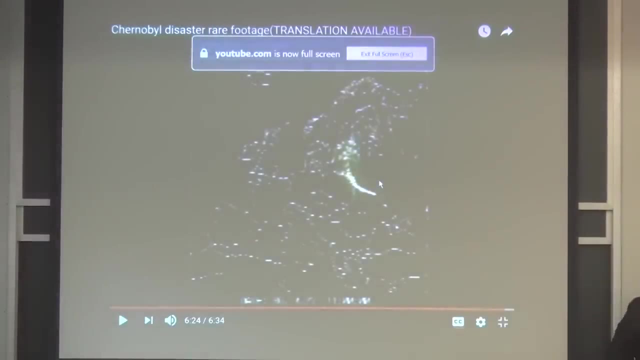 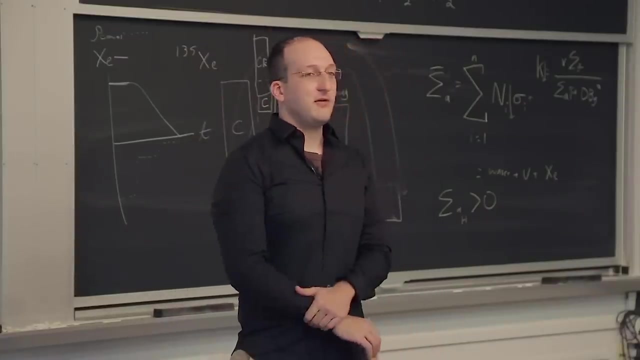 reports, is not that structurally sound and is in danger of partial collapse. so, yeah, more difficult efforts are ahead, but let's now talk about what happened next to not so close by Sweden. So it was noticed that folks entering a reactor in Sweden had contaminants on them which they thought was coming from their own reactor. good first assumption. When it was determined that nothing was amiss at the reactor in Sweden, folks started to analyze wind patterns and find out what happened. And then it was clear that the USSR had tried to cover up the Chernobyl accident. But you can't cover up fallout And it eventually spread pretty wide, covering most of Europe and Russia and, surprisingly, not Spain, Lucky them for the wind patterns that day or those few days. So what happened is a few days after the actual accident. 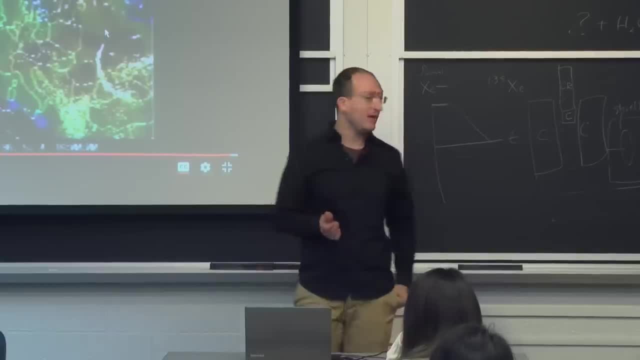 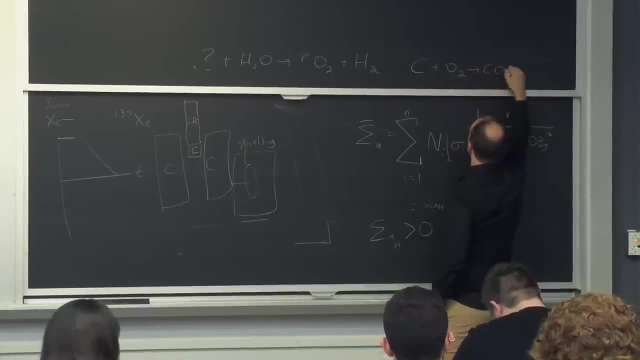 a graphite fire started to break out Because graphite, when exposed to air, well you can do the chemistry. Add graphite plus oxygen, you start making carbon dioxide. So graphite burns when it's hot And, as you could see from the video, 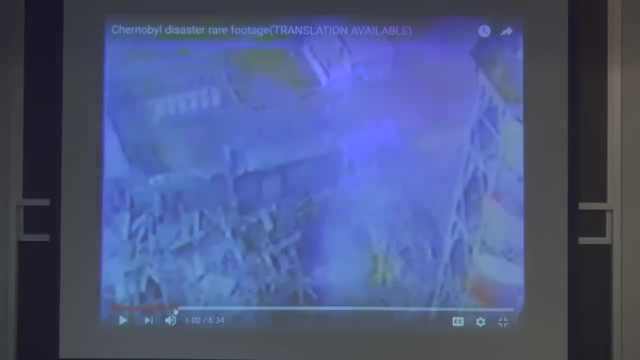 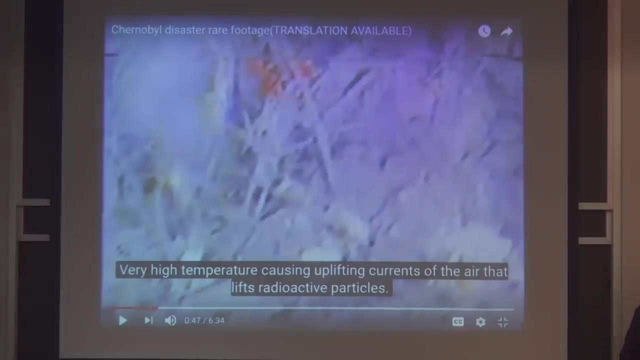 graphite burns when it's hot. So graphite burns when it's hot. Where is that nice still of burning graphite? Yeah, that graphite was pretty hot, So a lot of that smoke included burning graphite and a lot of the materials from the reactor itself. Now, when you build up fission products in a reactor and they get volatilized like this, the ones that tend to get out first would be things like the noble gases. So the whole xenon inventory of the reactor was released. It's estimated about 100%. 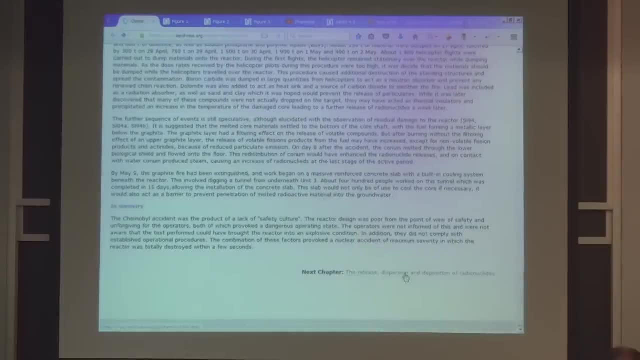 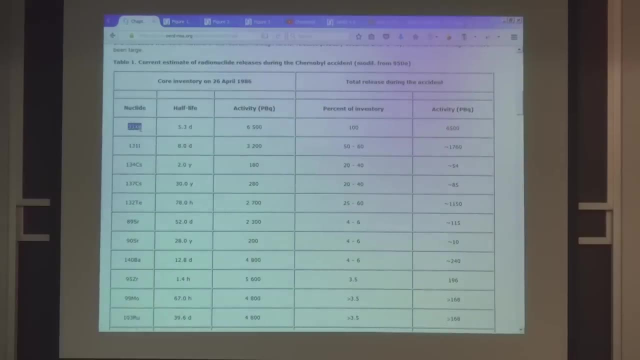 And I can actually pull this. I can actually pull up those figures- And we talk about how much of which radionuclide was released. That's also a typo. If somebody wants to call in, there's no 33 isotope of xenon. 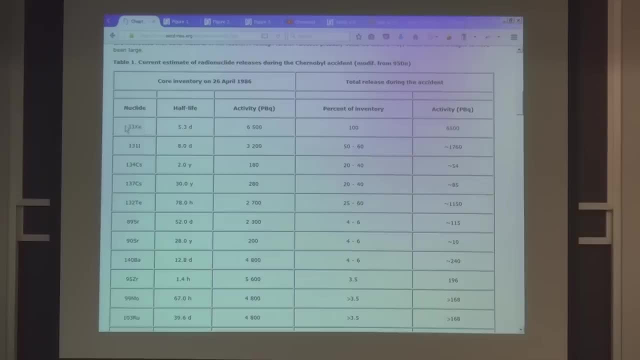 It's supposed to be 133.. That would be interesting if someone wants to call in and say the NEA has got a mistake. So 100% of the inventory released. That should be pretty obvious, because it's a noble gas and it just kind of floats away. 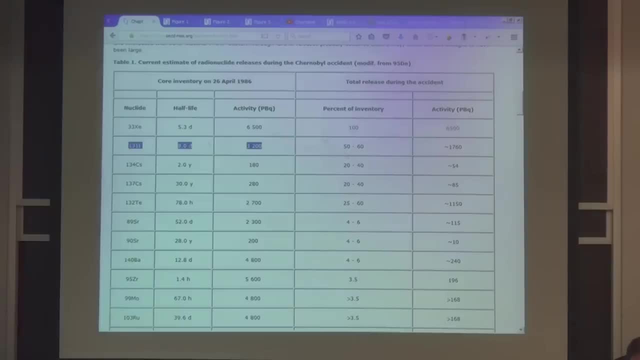 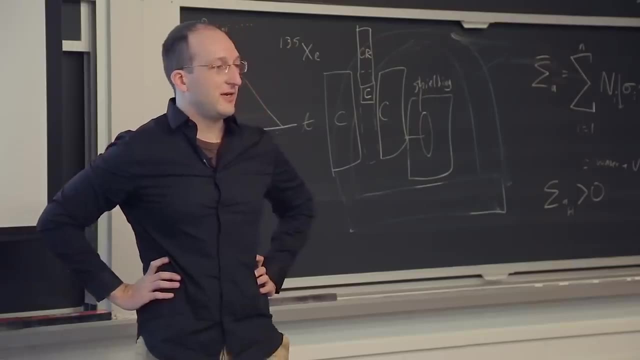 The real dangers, though, came from iodine-131.. About 50% of a 3-hexabacryl activity, So we're talking like mega curies. It might be giga. I can't do that math in my head. 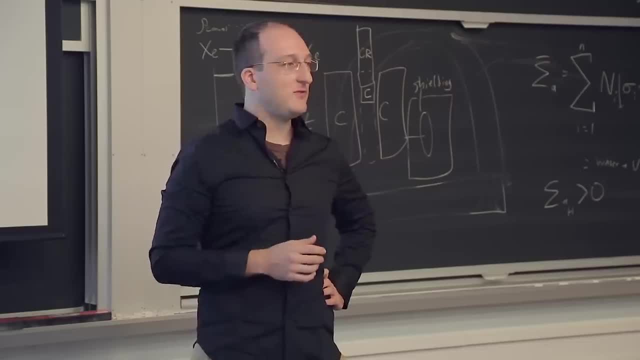 Lot, a lot of radiation, And the problem with that is iodine behaves just like any other halogen. It forms salts. It's rather volatile. Have any of you guys played with iodine before? No one does? Oh, you have. 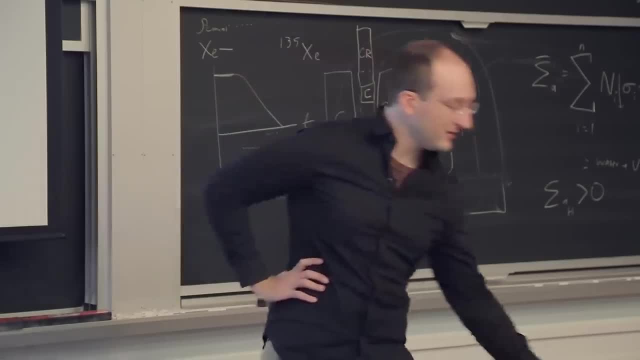 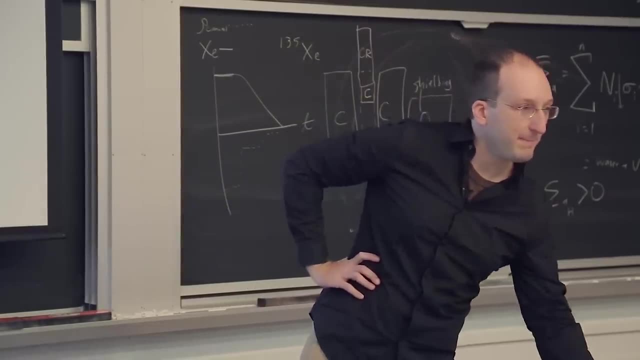 OK, What happens with it? Play with it. I mean, it just throws some stuff, Like hmm, It turns everything yellow And it just reacts with like acids and stuff. But I don't play with it, very much with it. 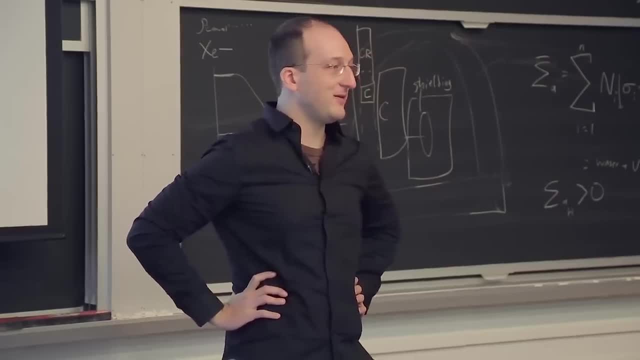 OK, I happen to have extensive practice playing with iodine in my home because I did all the stuff you're not supposed to do as a kid, Kind of build your own chemistry stuff and things that somehow leak out of your local high school somehow. 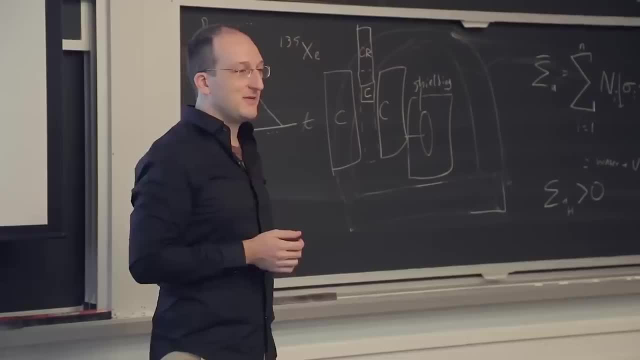 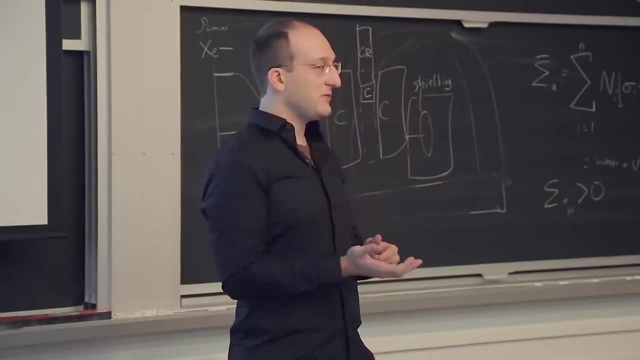 Iodine's pretty neat. How does it feel? Yeah, it happens sometimes. If you put iodine in your hand, it actually sublimes. The heat from your hand is enough to directly go from solid to vapor, And so the iodine was also quite volatile. 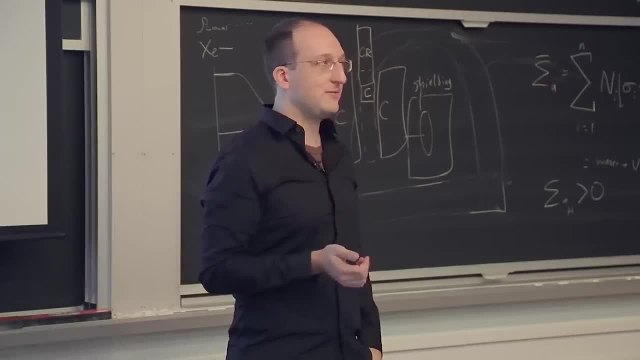 Some of it may have been in the form of other compounds. Some of it may have been elemental. Probably not likely, But there was certainly some iodine vapor, And about half of that was released. The problem is then it condenses out and falls. 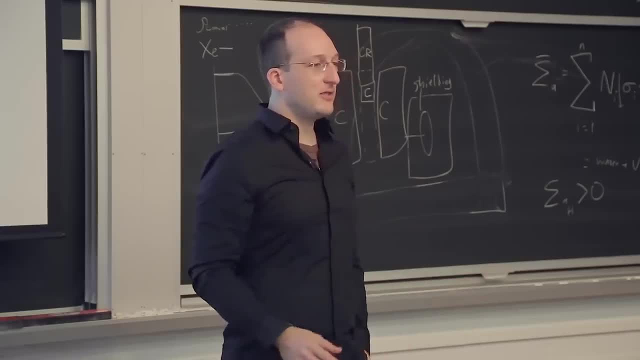 on anything green, anything with surface area. So the biggest danger to the folks living nearby was from eating leafy vegetables, because the leaves got lots of surface area And that's why it's so important to have iodine deposits on them, And it's intensely radioactive for a month or so. 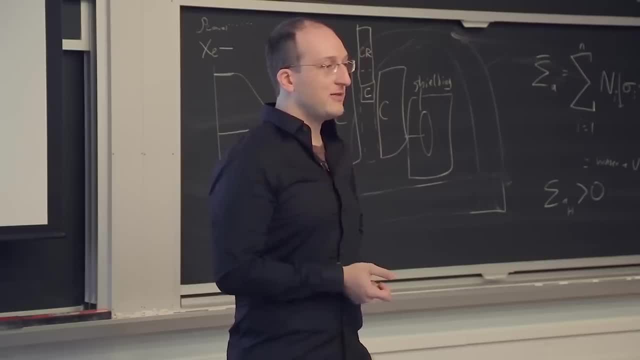 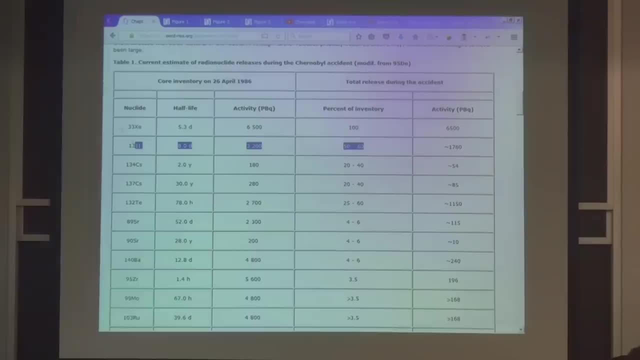 Or depositing on the grass that cows eat, which led to the problem of radioactive milk, And so that's why milk in the Soviet Union was banned for such a long time, because this was one of the major sources of iodine contamination, The other one which we're worrying about now. 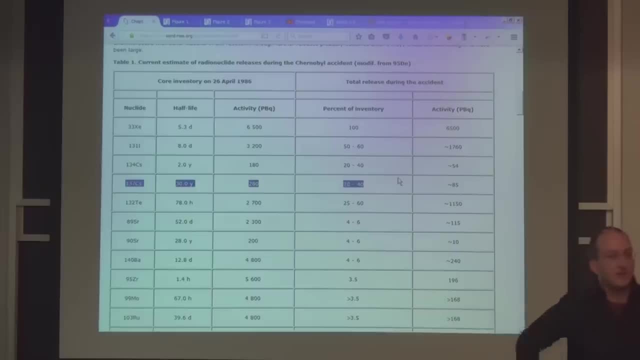 from Fukushima as well is cesium, which has similar chemistry to sodium and potassium, Again a rather salty compound, Or a rather salty element, But it's got a half-life of 30 years And if we look it up in the table of nuclides, 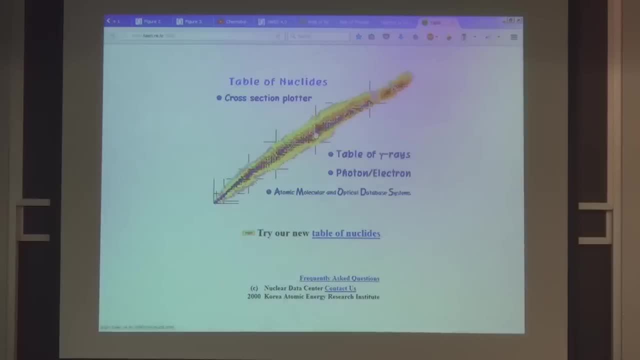 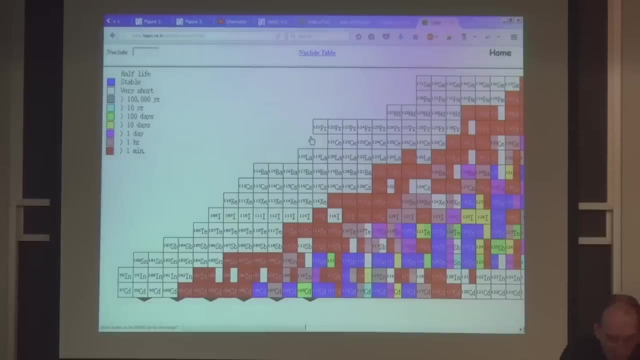 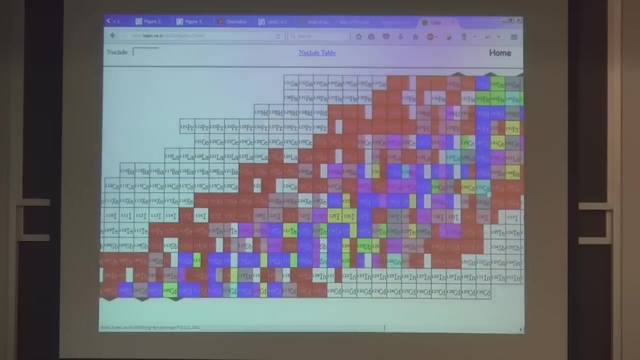 we'll see what it actually releases. Oh good, It's back online. Anyone else notice this? broken a couple of days ago. Yeah Well, luckily Brookhaven National Lab has a good version up too. Let's grab cesium. 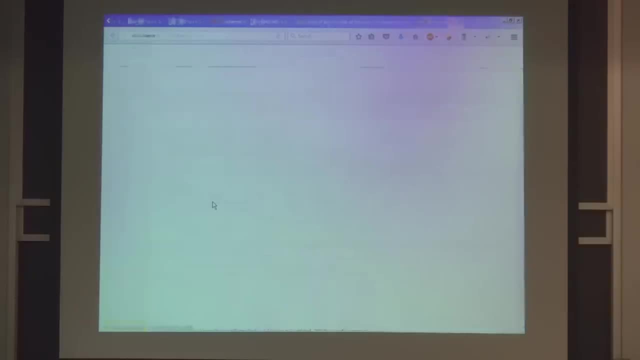 Yeah, there's plenty out there: Cesium-137, beta decays to barium but also gives off gamma rays And most of the decays end up giving off one of those gamma rays. Let's say a 660 KeV gamma ray. 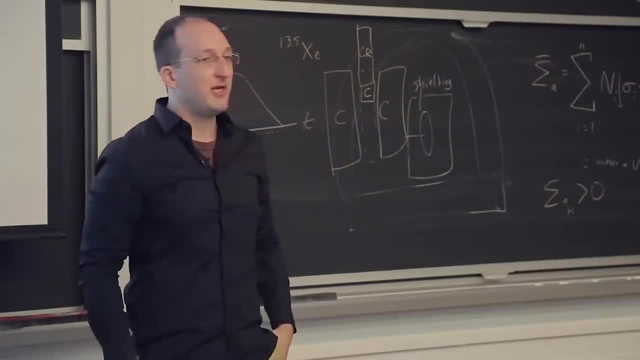 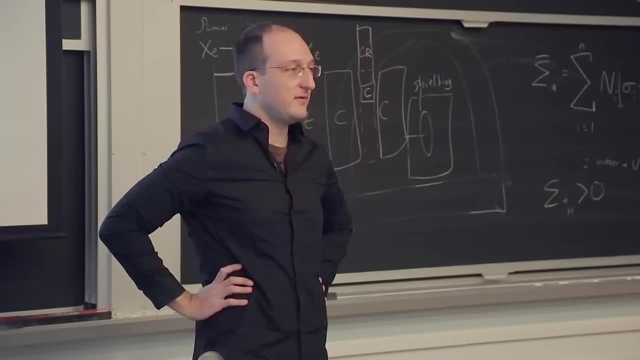 So it's both a beta and a gamma emitter. Now which of those types of radiation do you think is more damaging to biological organisms, The beta or the gamma? You say the gamma. Why do you say so? Doesn't beta get stopped by skin clothing? 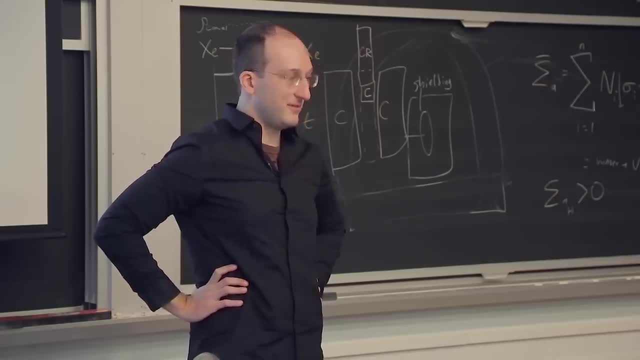 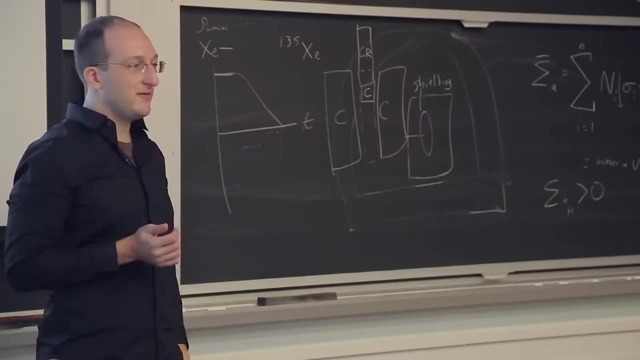 It does. But if cesium is better known as, Yes, That's right. So did I get to tell you guys this question? the four cookies question: Yeah, You eat the gamma cookie, because most gammas that are emitted by the cookie simply leave you. 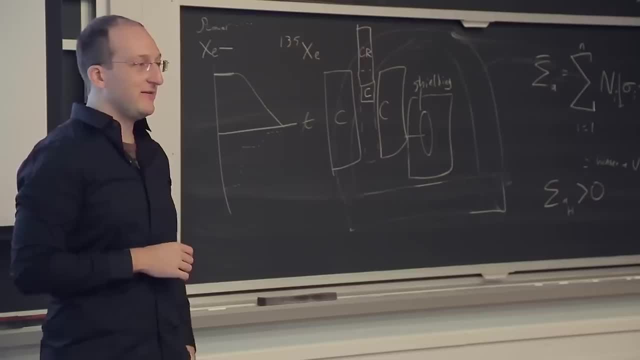 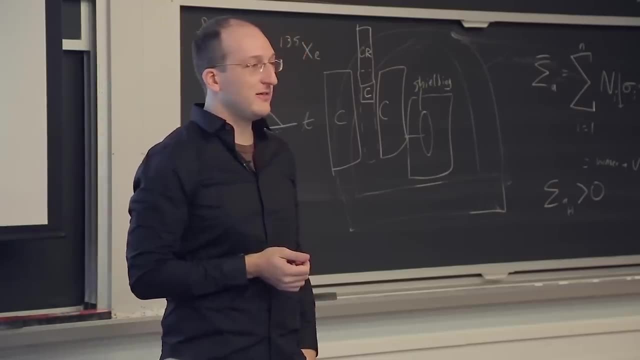 and irradiate your friend, which is going to be the topic of p set number eight. You'll see, That's why you guys are getting your whole body counts. Speaking of, who's gotten their whole body counts at EHS- Awesome. 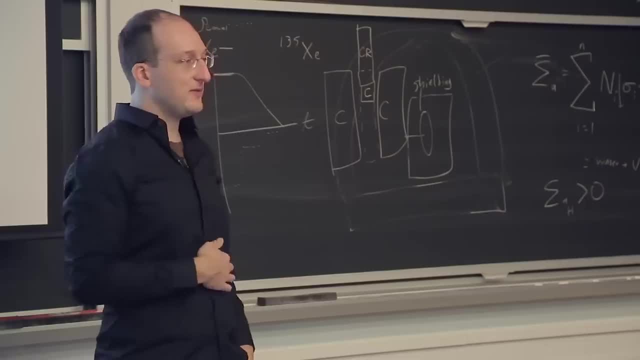 So that's almost everybody. You will need that data for problem set eight, So do schedule it soon, preferably before Thanksgiving, so that you'll be able to take a look at it. Has anyone found anything interesting in your spectra? Good, Glad to hear that. 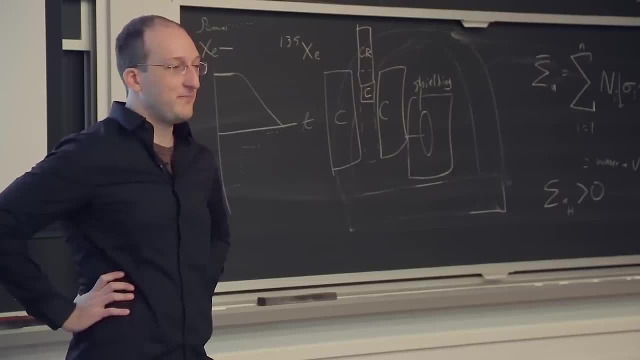 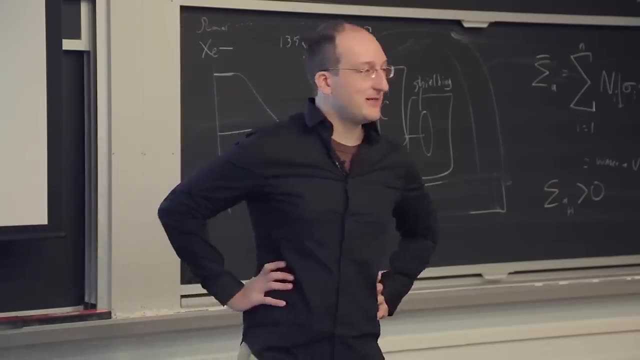 But you do see a potassium peak that you can probably integrate and do some problems with, right, Yeah, because you will. OK. Anyway, yeah, it's the betas that's the real killer. The gammas are going to leave the cesium enter your body. 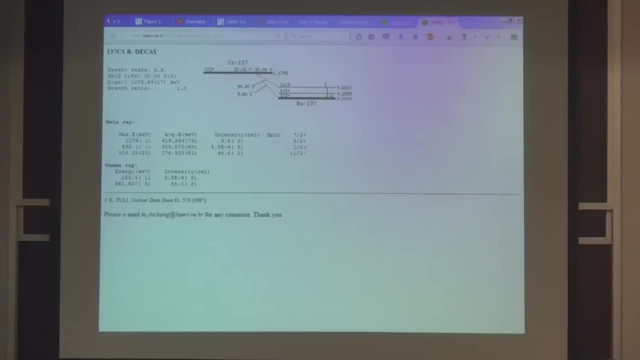 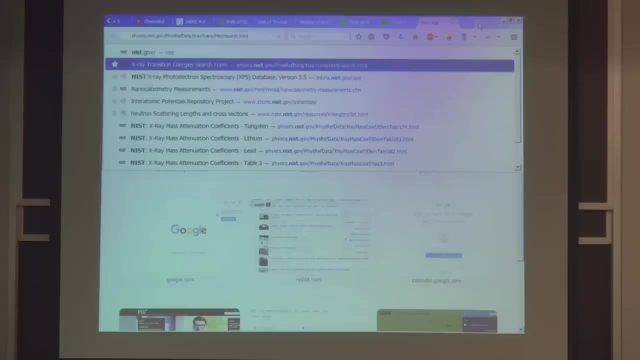 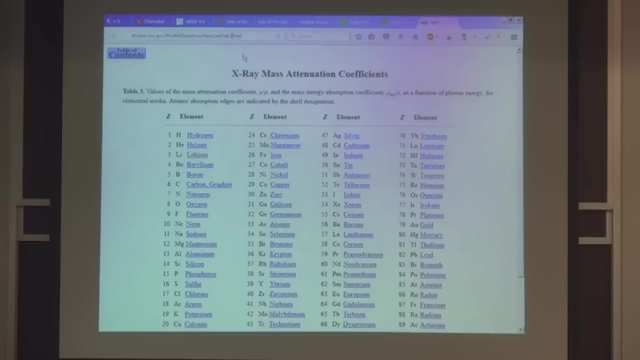 and most likely come out the other side, Because the mass attenuation coefficient of 6,. what is it? water for 660 keV gammas. let's find that table three. Let's say you're made mostly of water, Water liquid. 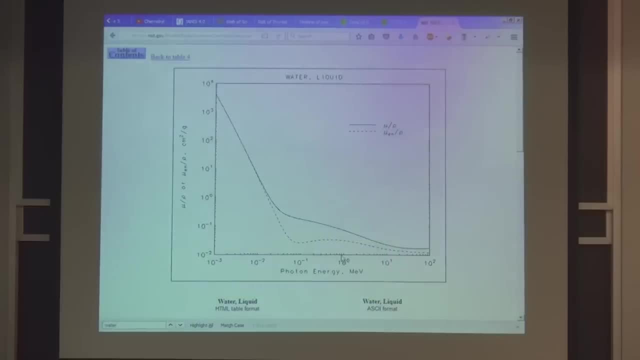 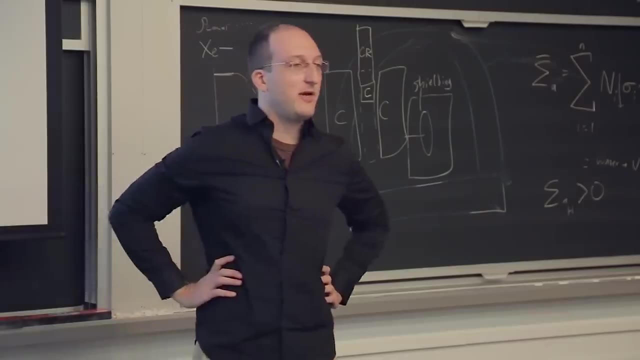 That's pretty much humans. 660 keV is right about here, leading to about 0.1 centimeters squared per gram, And with a density of 1 gram that's a pretty low attenuation of gammas. So this chart actually shows why most of the cesium gammas that 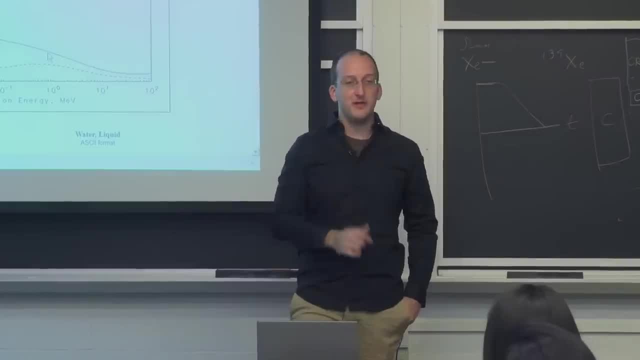 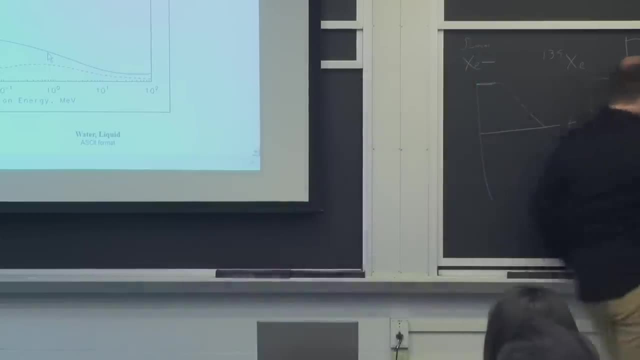 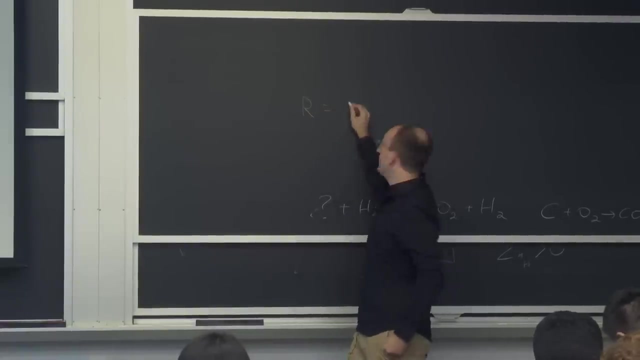 would be produced from ingestion, just get right out. But it's the betas that have an awfully short range. Anyone remember the formula for range in general, Because it's going to come back up in our discussion of dose and biological effects, The integral of 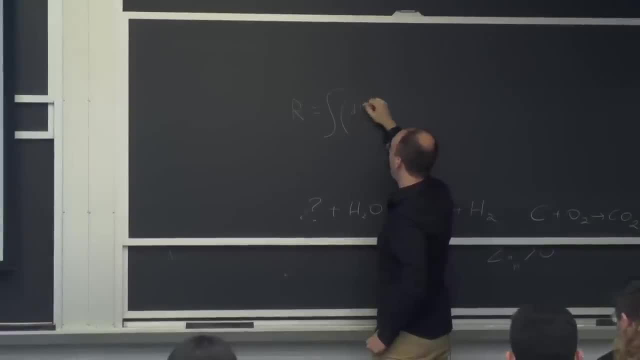 MICHAEL SHORTENBERGER- Integral of The negative of 1.. MICHAEL SHORTENBERGER- Yep Of stopping. MICHAEL SHORTENBERGER- Stopping power to the negative 1. And that stopping power is this simple formula. 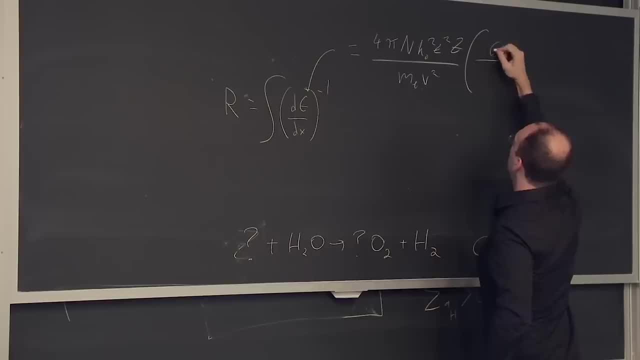 Let's see. What did that come out? as? Log minus theta squared. That simple little formula, which I'm not going to expect you guys to do, MICHAEL SHORTENBERGER- Yeah, I'm not going to ask you guys to memorize. 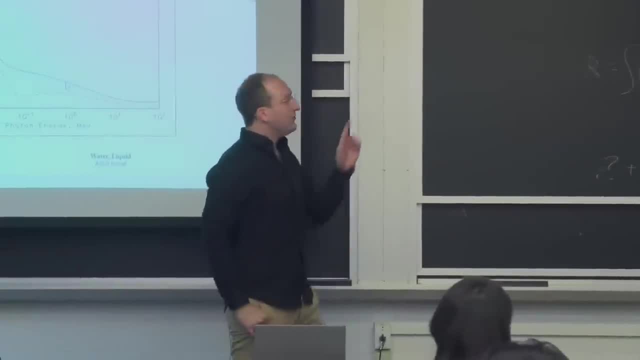 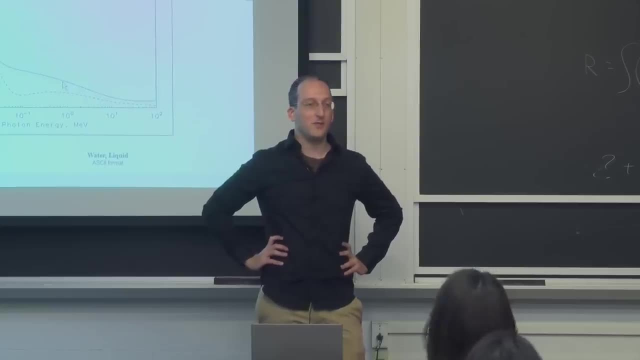 so don't worry about it. But if you integrate this, you find out that the range of electrons- even 1 MeV electrons- in water, is not very high, So most of them are stopped near or by the cells that absorb them, doing quite a bit of damage. 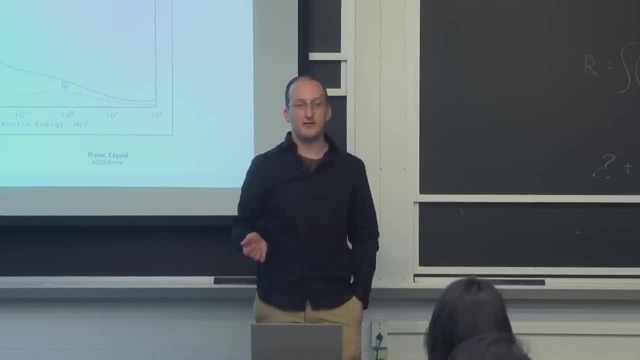 to the DNA, which is eventually what causes mutagenic effects, cancer, cell death, what we're going to talk about for the whole third part of the course. There's also a worry about which organs actually absorb these radionuclides. 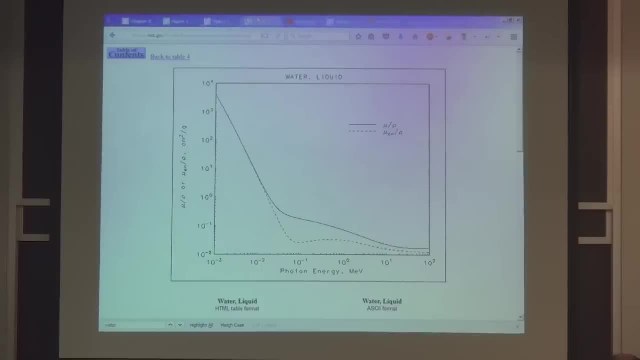 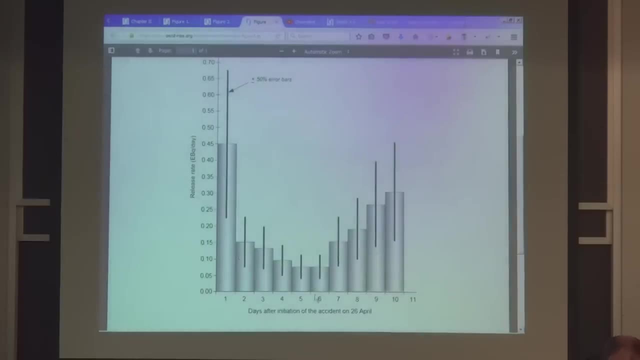 And iodine in particular, is preferentially absorbed by the thyroid. So when we started looking at the amount of radioactive substances released, remember they said OK, at around 26th of April or the 2nd of May or so the release was stopped. 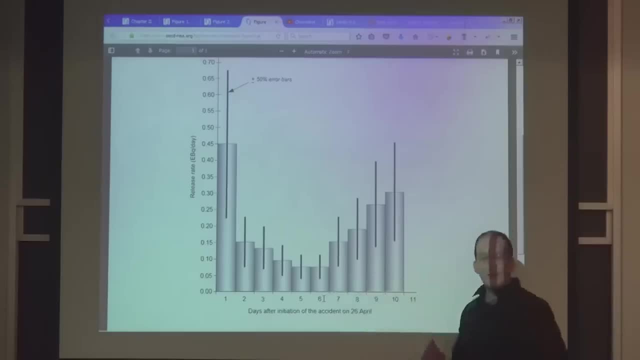 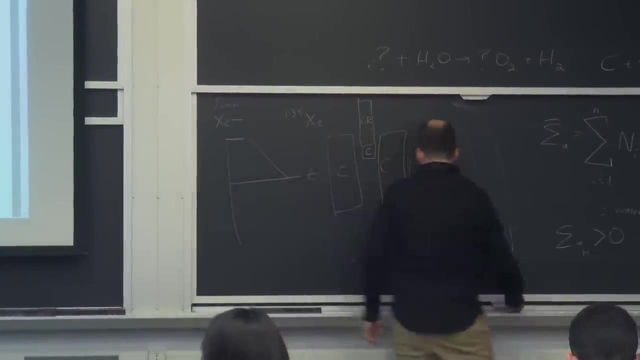 Not. according to our data, That's when the graphite fire picked up again. In addition, the core of Chernobyl, which had undergone a mostly total meltdown, was sitting in a pool. It was a pool on top of this concrete pad. 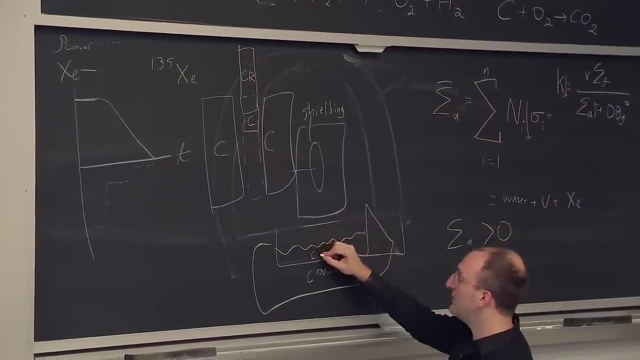 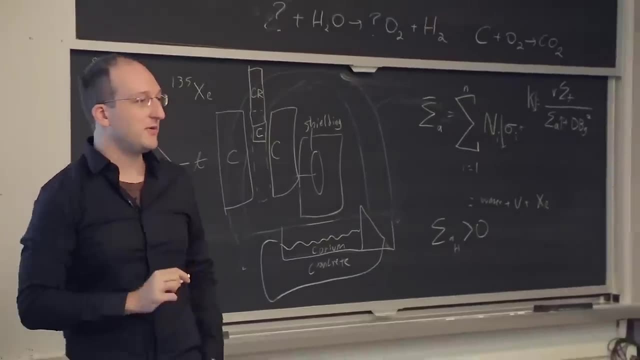 So let's just call this liquid stuff. The actual word that we use in pyrolytes is called corium. It's our tongue-in-cheek word for every element mixed together in a hot radioactive soup. First of all, it started to redistribute. 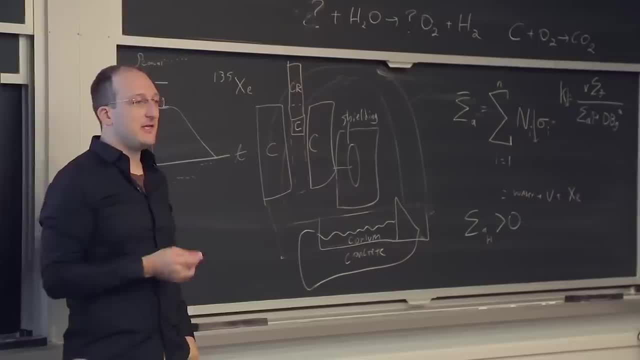 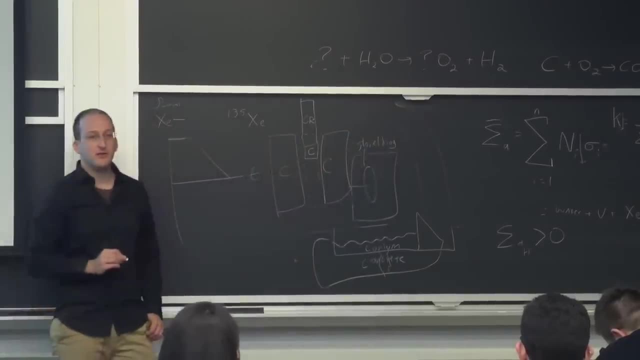 reacting with any water that was present, flashing it to steam, And the steam caused additional dispersion of radionuclides And eventually it borrowed its way through and into the ground, Releasing more. It's the worst nuclear thing, that's. 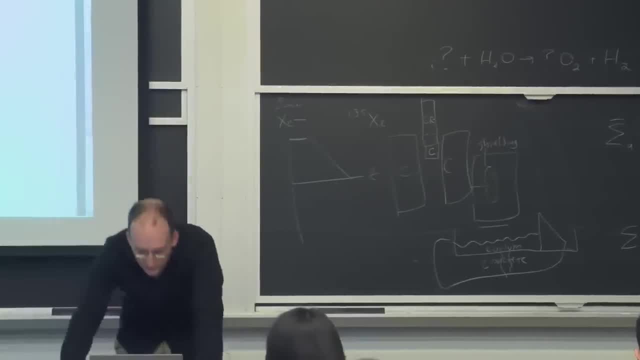 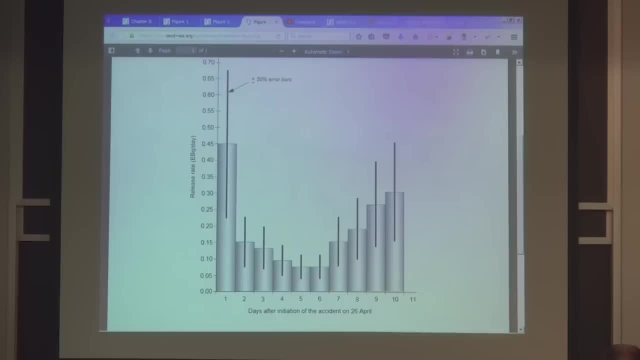 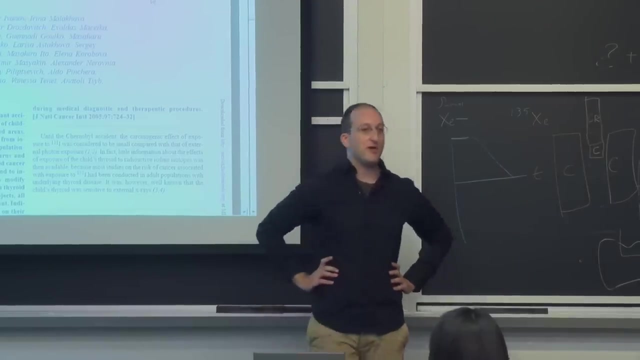 ever happened in the history of nuclear things. Quite a mess, And luckily it did sort of taper off after this. But let's now look into what happens next, And this is the nice intro to the third part of the course. Iodine is preferentially uptaken by the thyroid gland. 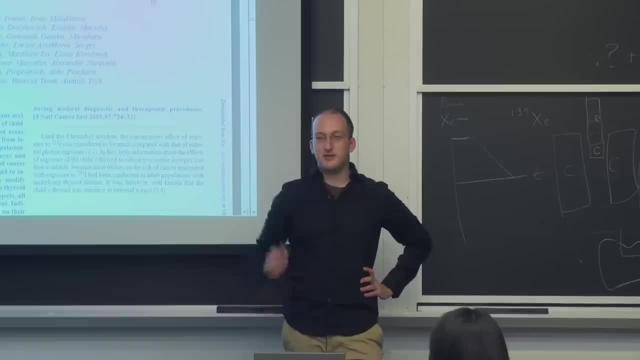 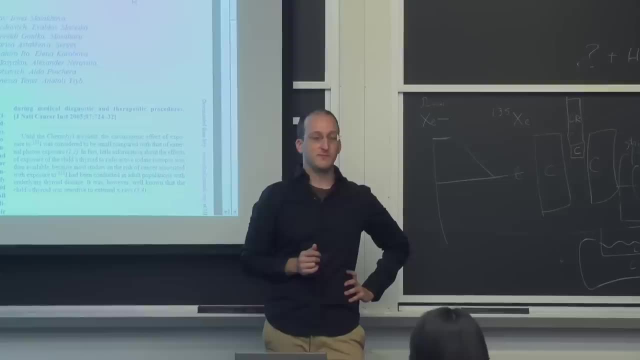 somewhere right about here? So has anyone ever heard of the idea of taking iodine tablets In the case, In the case of a nuclear disaster? Anyone have any idea why? If you saturate your thyroid with iodine, then if you ingest radioactive iodine, 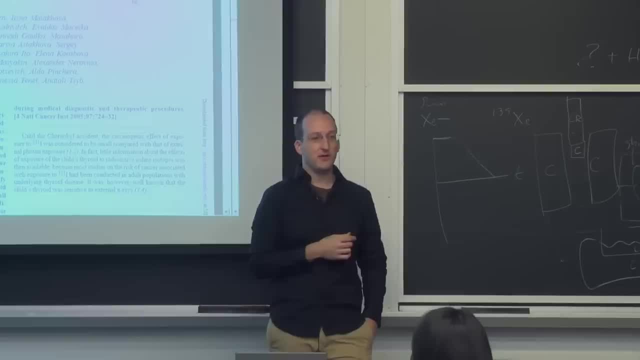 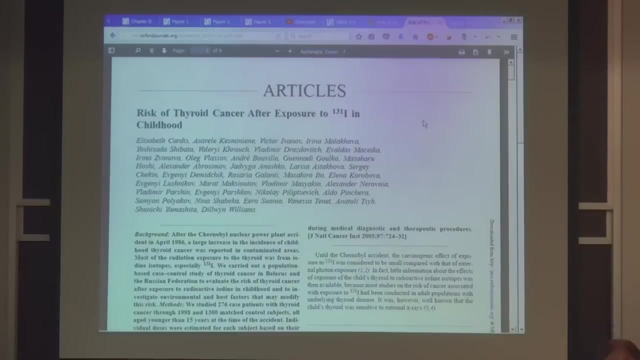 it's less likely to be permanently uptaken by the thyroid. So this actually provided some statistics on the probability of getting thyroid cancer from radioactive iodine ingestion. Luckily the statistics were quite poor, which means that not many people were exposed. It was somewhere. 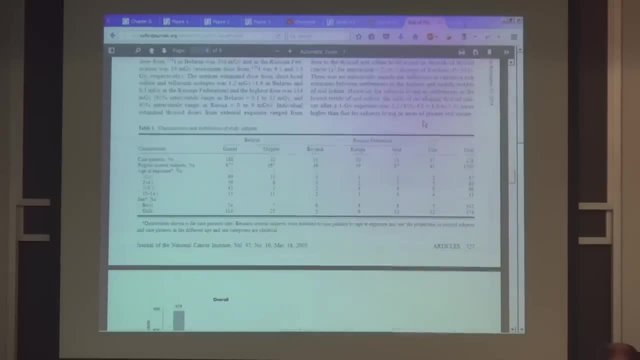 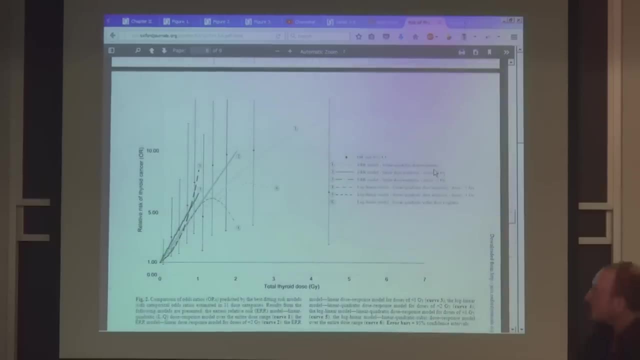 Around 1,300 or so, Not like millions. Yeah, 1,300 people total. But what I want to jump to is the dose versus risk curve, And this is going to belie all of our discussion about the biological long-term effects of radioactivity. 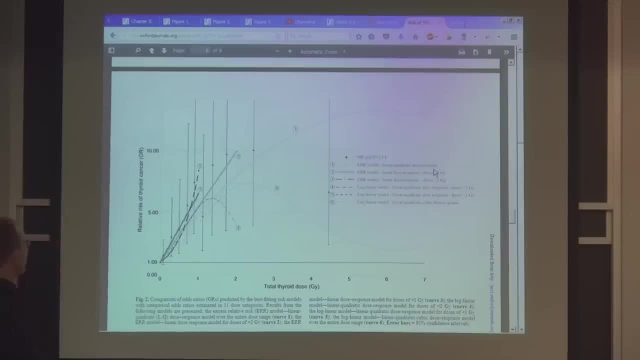 What's the most striking thing you see as part of this curve? Aerobatics. That's right. That's the first thing I saw. There are six different models For how dose and increased risk of cancer proceeds, And they all fall within almost all the error. 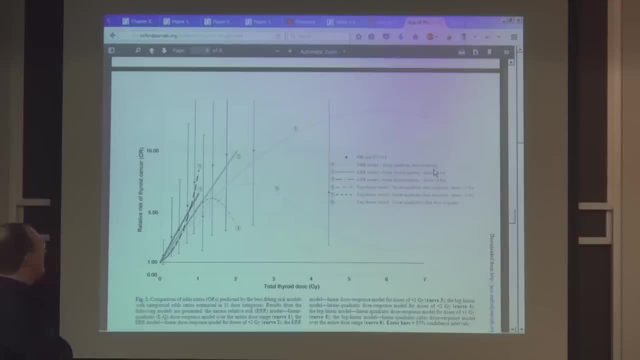 bars of these measurements. I say again: thank God that the error bars are so high, because that means that the sample size was so low. So when folks say we don't really know how much radioactivity causes how much cancer, they're right. 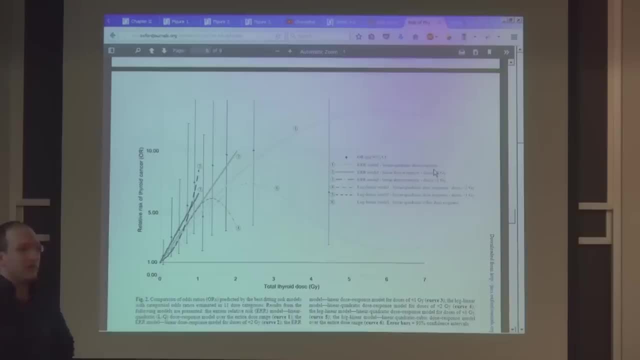 Because luckily we don't have enough data from people being exposed to know that really really well. So some folks say we should be cautious. I kind of agree with them. Some folks say the jury's still out. I also agree with them. 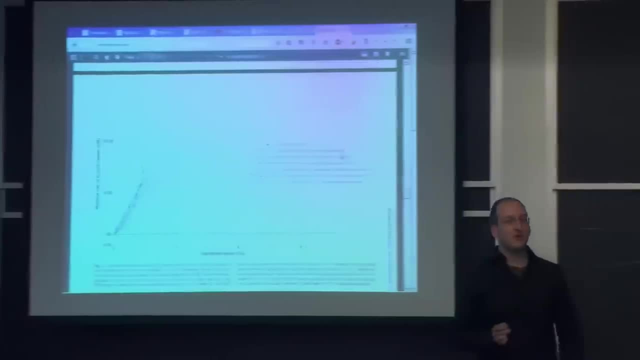 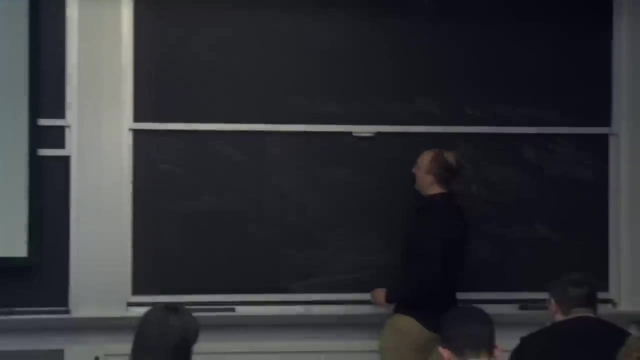 But you can start to estimate these sorts of things by knowing how much radiation energy was absorbed and to what organ. So I think the only technical thing I want to go over today is the different units of dose, Because as you start to read things in the reading- which I recommend you do if you haven't- 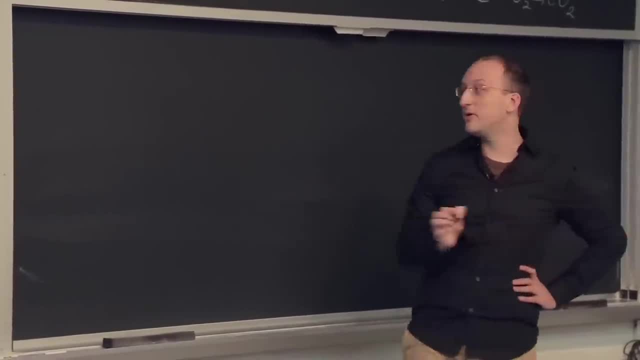 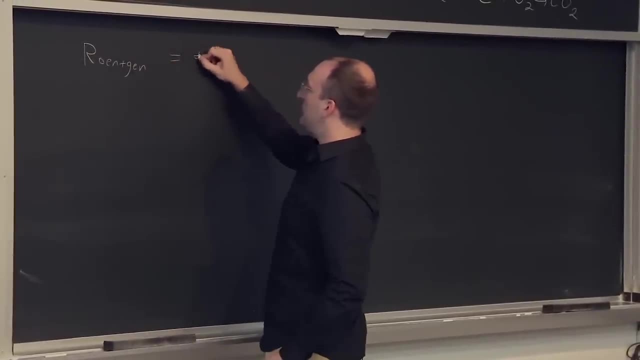 been doing. yet you're going to encounter a lot of different units of radiation dose, ranging from things like the rentgen, So a lot of the people who have been doing this are probably going to be interested in this. But if you're interested in the dosimeter, 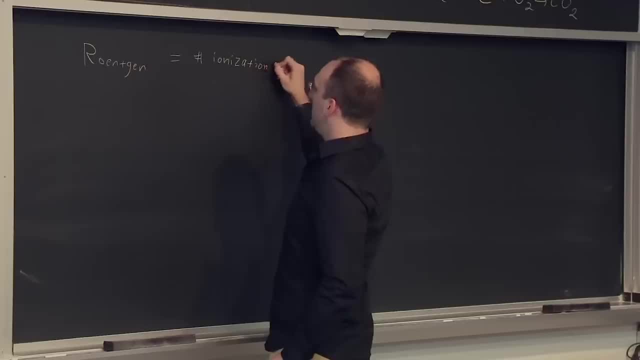 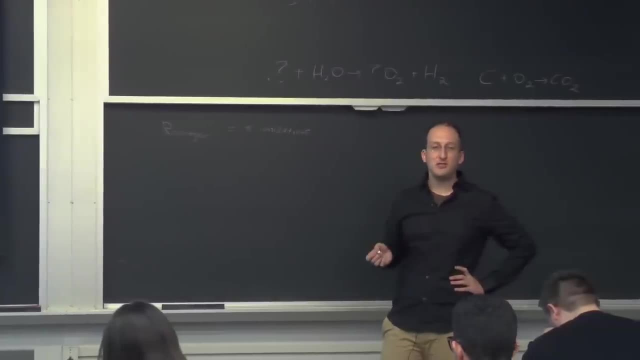 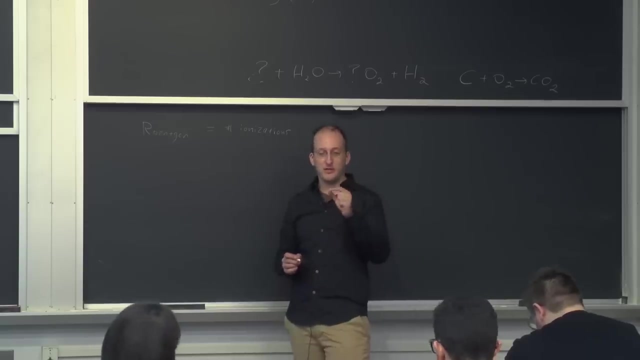 which responds to a number of ionizations. you won't usually see this one given in sort of biological parlance, Because it's the number of ionizations detected by some sort of gaseous ionization detector. So the dosimeters that you all put on, 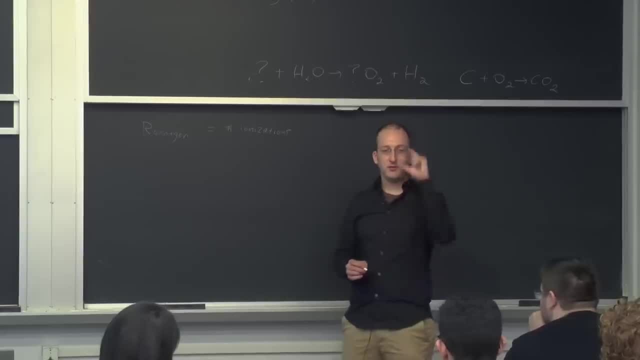 did you guys all bring these brass pen dosimeters into the reactor? It's going to be in Roentgens because that's directly correlatable to the number of ionizations that that dosimeter has experienced. You'll also see four dose units, two of which 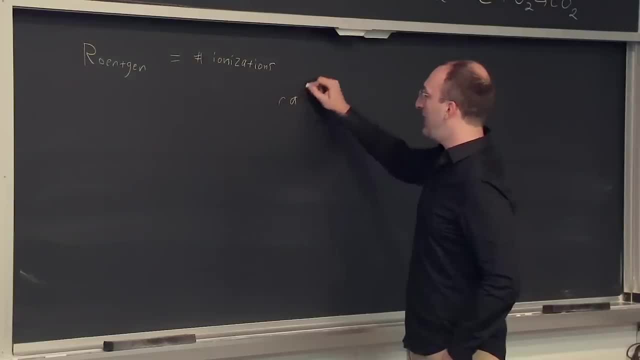 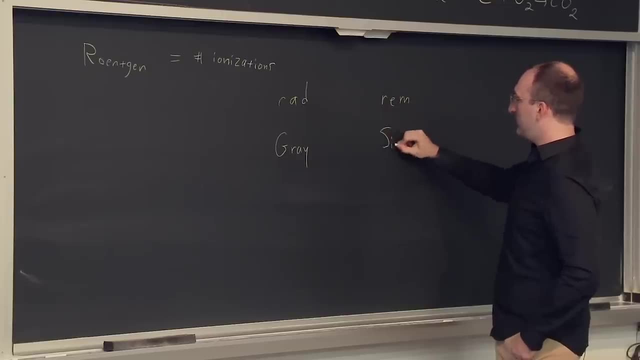 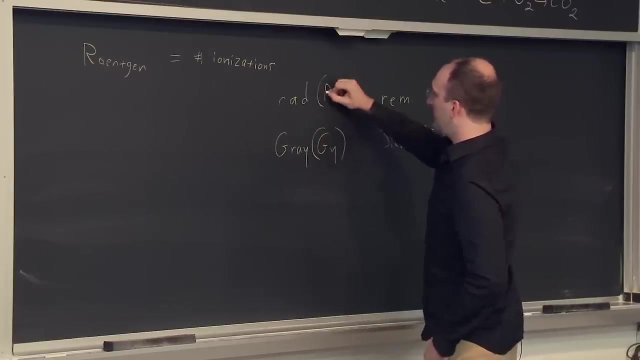 are just factors of 100 away from each other. There's what's called the rad and the gray And there's what's called the rem and the sievert. You'll see these approximated as gray. You'll see these as R, And these are just. 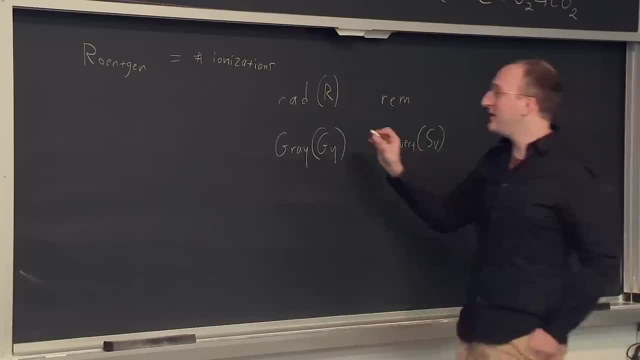 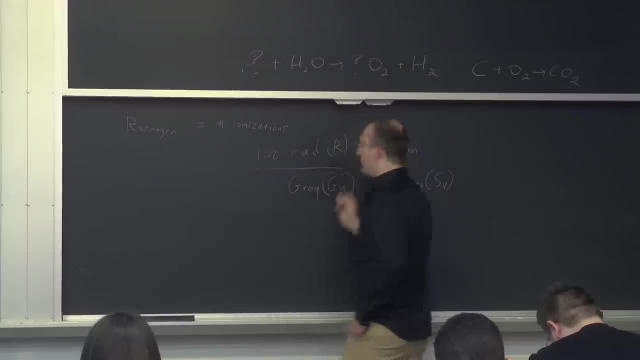 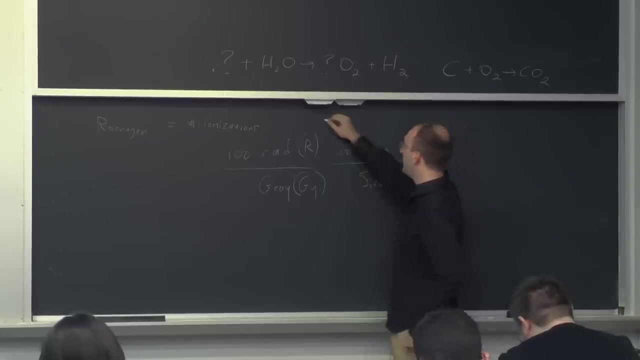 usually written as rem. So a rad is simple. Let's see: 100 rads is the same as one gray And 100 rem is the same as one sievert. And for gamma? for the case of gamma radiation, these units are actually equal. 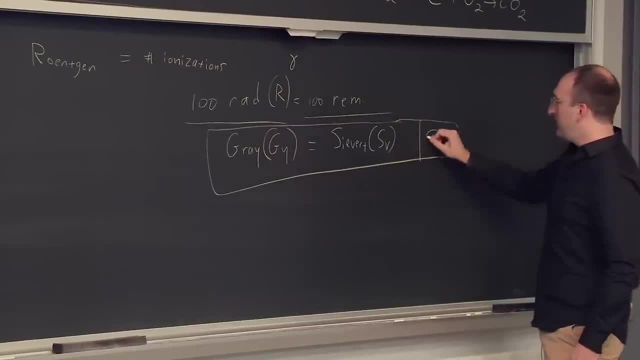 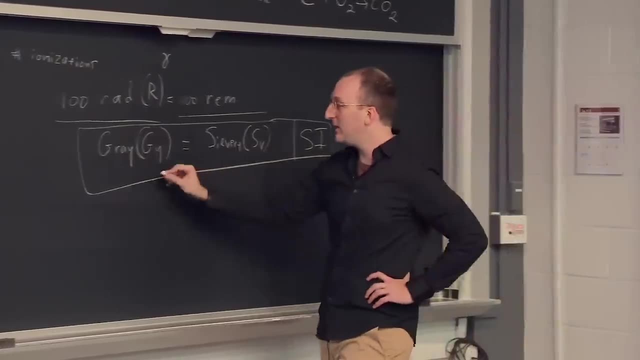 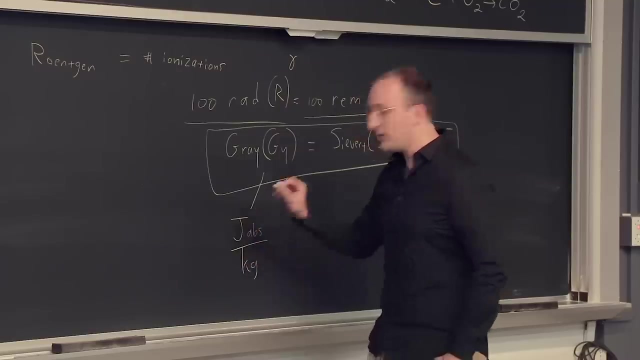 I particularly like this set of units because this is it. This is the kind of SI of radiation units, because it comes directly from measurable, calculatable quantities, Like the gray, for example. the actual unit of gray is joules absorbed per kilogram of absorber. 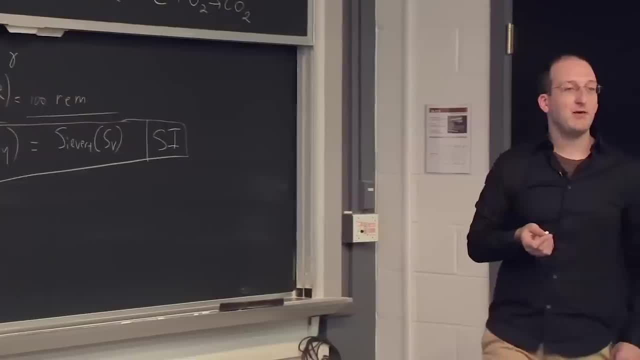 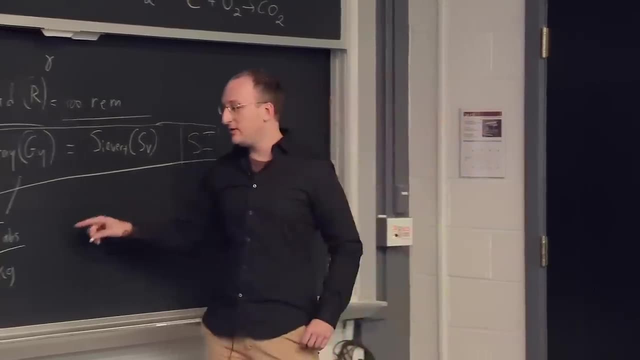 It's a pretty simple unit to understand. If you know how many radioactive particles or gammas or whatever that you have absorbed, you can multiply that number by their energy, divide by the mass of the organ absorbing them, and you get its dose in gray. 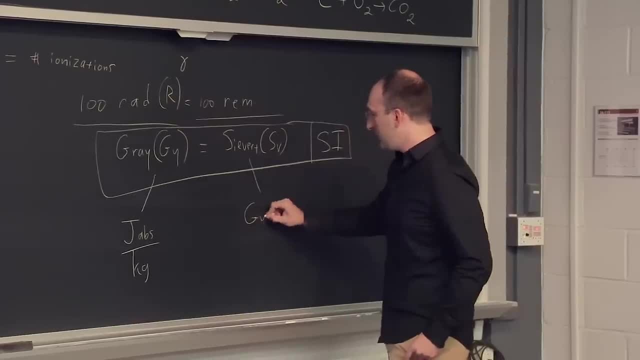 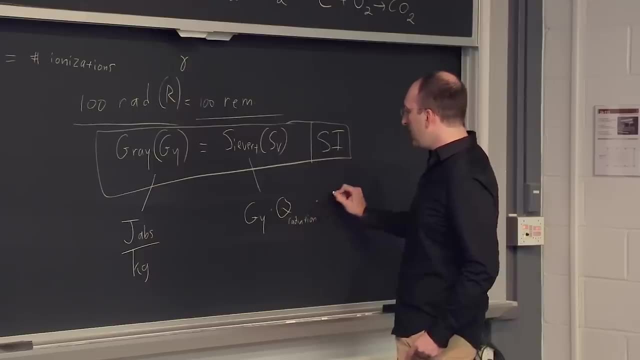 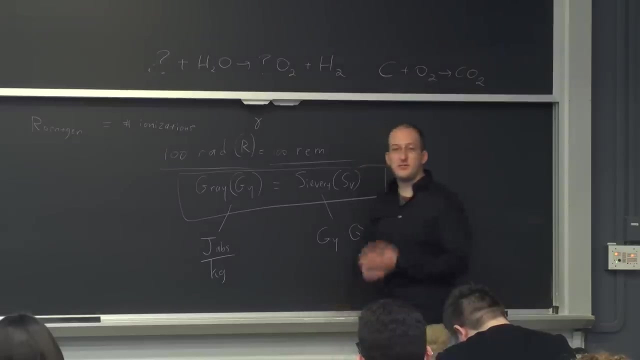 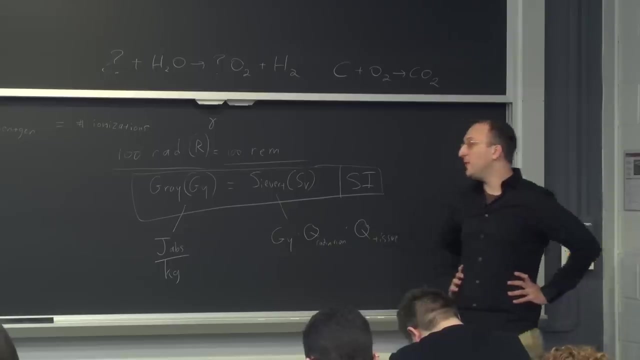 Sievert is gray times, some quality factor for the radiation times, some quality factor for the specific type of tissue. What this says is that some types of radiation are more effective at causing damage than others And some organs are more susceptible to radiation damage than others. 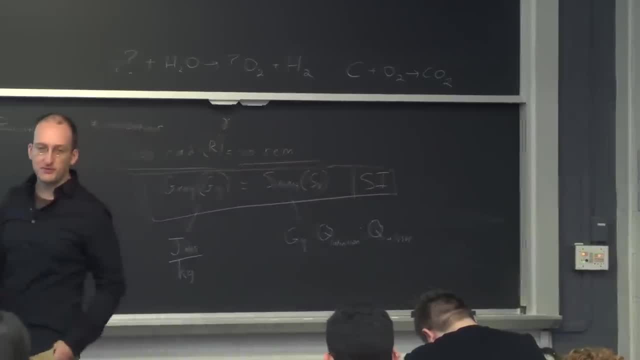 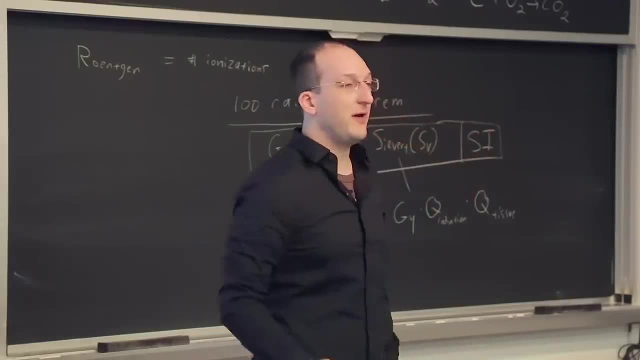 Does anyone happen to know some of the organs, organs that are most susceptible to radiation damage? Soft tissues- MICHAEL SHORTLAND- Soft tissues like what? Because there's lots of those. So like stomach lining, MICHAEL SHORTLAND- Stomach lining, yup. 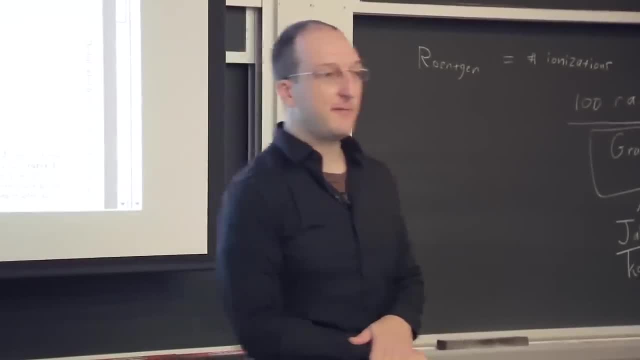 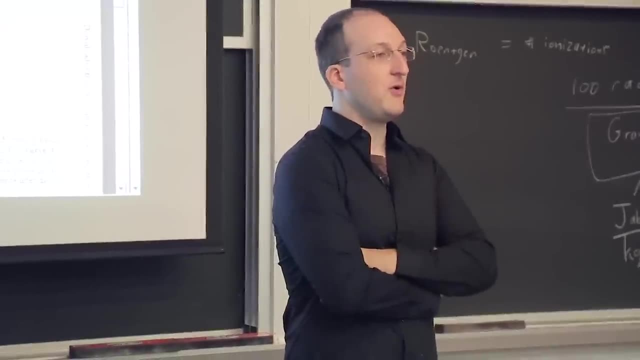 Yeah, Huh. Lungs- MICHAEL SHORTLAND- Lungs- yup, What else? Thyroid- MICHAEL SHORTLAND- Thyroid- Yup, there is definitely one for thyroid. Bone marrow- MICHAEL SHORTLAND- Bone marrow. 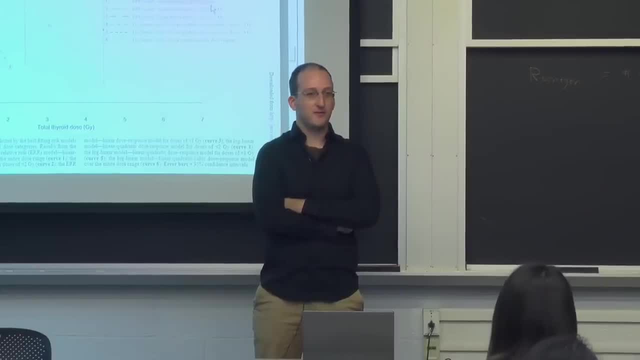 What other ones? MICHAEL SHORTLAND- Brain. MICHAEL SHORTLAND- Brain. actually, not so much Eyes. And where else do you find rapidly dividing cells in your body Skin? MICHAEL SHORTLAND- Skin. yup the dermis. 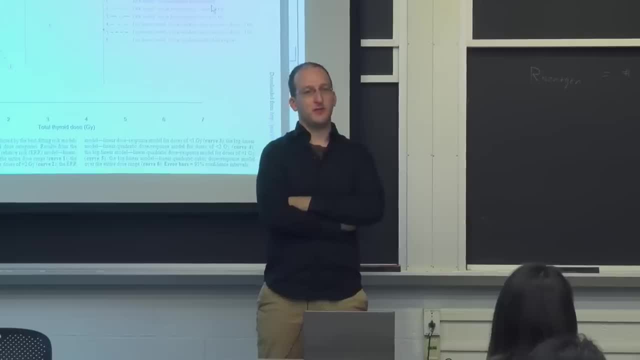 Liver. MICHAEL SHORTLAND- I don't know about the liver, I would assume. so Yeah, it's a pretty active organ. But when folks are worried about birth defects, reproductive organs, the link here that for some reason is not said in the reading and I've never figured out why. 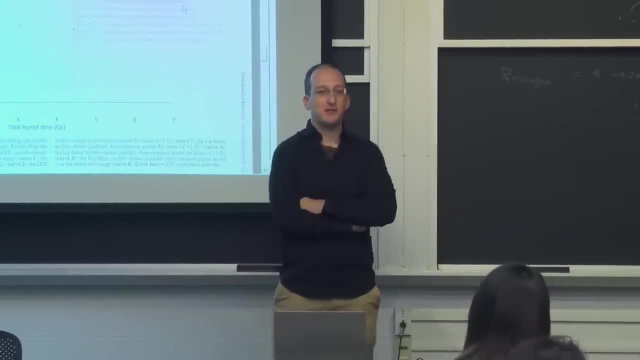 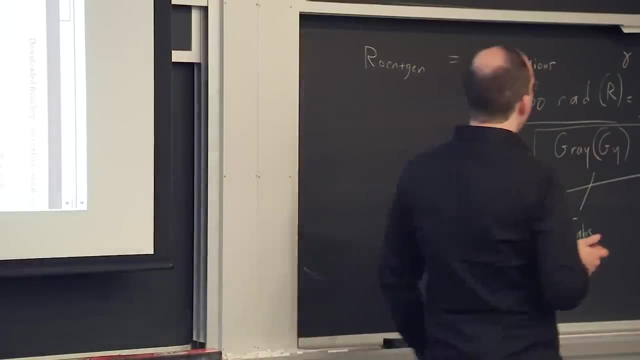 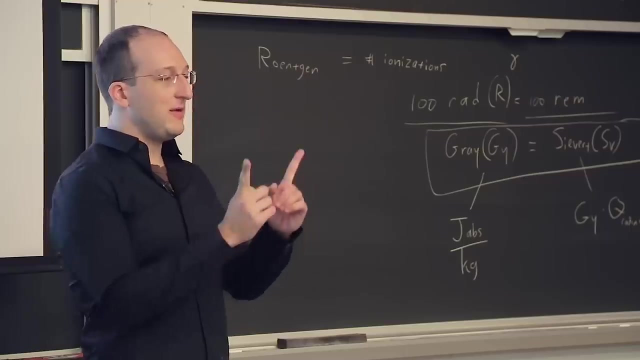 is, the more often a cell is dividing, the more susceptible it is to gaining cancer risk, Because every cell division is a copy of its DNA And any time that radiation goes in and damages or changes that DNA, by either causing what's called a thymine bridge, where two thymine bases get linked- together or damaging the structure in some other way. that gene is then replicated, And the faster they're replicating, the more likely cancer is going to become apparent. I guess This brings up a question: when does a rapidly dividing cell become cancer? 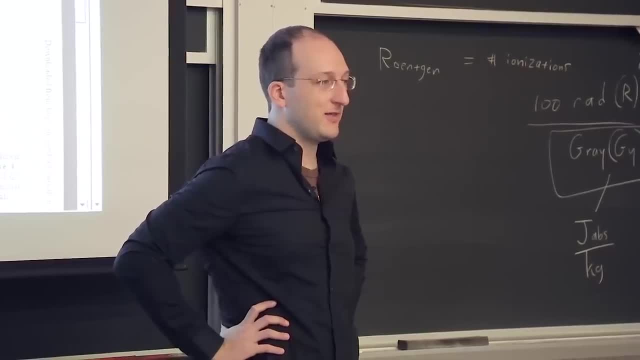 Is it division number one, or is it when you notice it? Guess I'll leave that question to the biologists. But if you notice, in the reading you'll see a bunch of different tissue equivalency factors And you'll just see them tabulated and say: 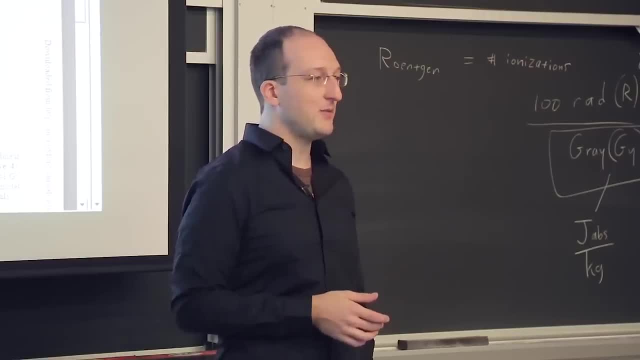 there they are, memorize them. I want you to try and think of the pattern between them. The tissues that basically don't matter, like the non-marrow part of the bone, dead skin cells, muscles- basically aren't listed that much. They're not dividing very fast, But anywhere where you find stem cells, the lining of your intestine, your lungs, which undergo a lot of environmental damage, need to be replenished: Gonads, skin, What was the other one that we said? 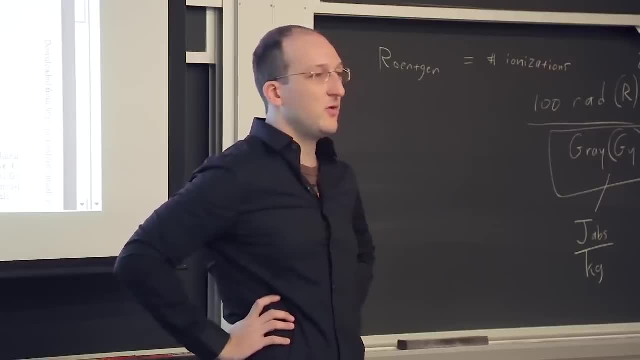 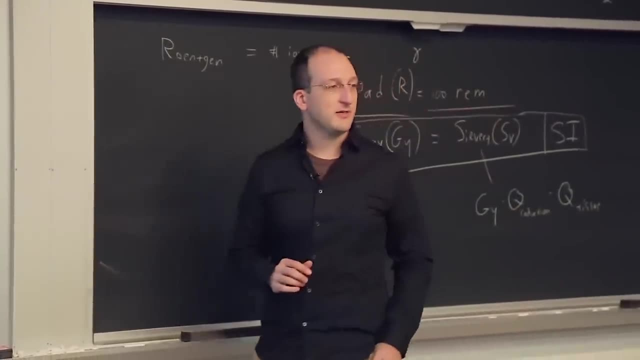 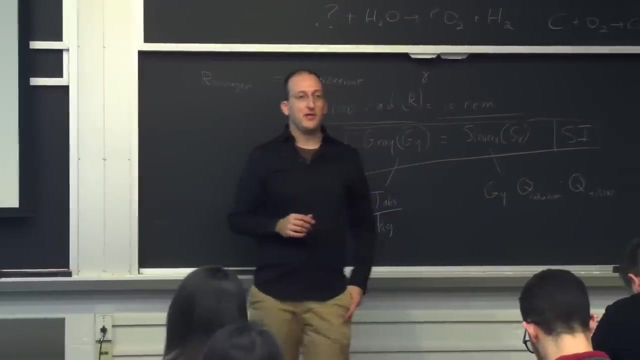 Eyes. These are places that are either sensitive tissues or they're rapidly dividing, And so the sievert is kind of a unit of increased equivalent risk, So that if you were to absorb one gray of gamma rays versus one gray of alphas, you'd be about 20 times more likely to incur cancer from the alphas than the gammas because of the amount of localized damage that they do to cells- And we'll be doing all this in detail pretty soon- And then for tissue equivalency factor. 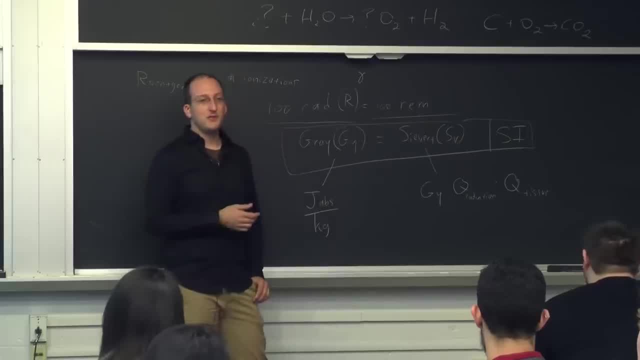 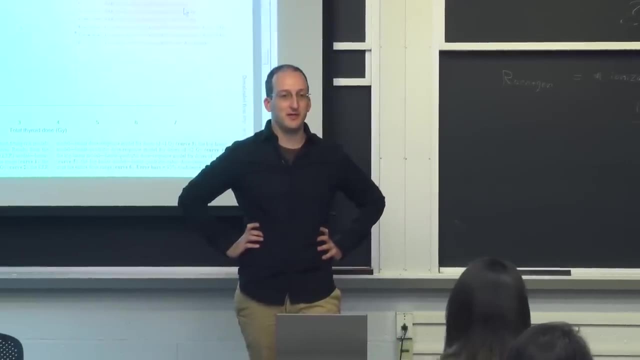 if you absorb one gray in your whole body, which means one joule per kilogram of average body mass, versus one gray directly to the lining of your intestine by, let's say, drinking polonium-laced tea, like happened to a poor- was it current or ex-KGB? guy? 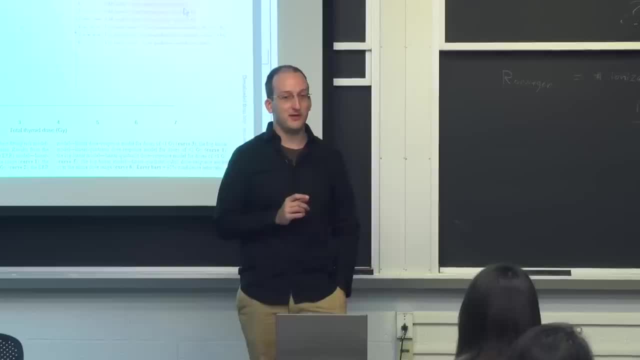 One of the Russian fellows. No, it's the KGB guys that poisoned him, right? Yeah, Do you guys remember? back in 2010 or so, there was a Russian? was he a journalist, Ex-KGB? So the current KGB somehow got into London. 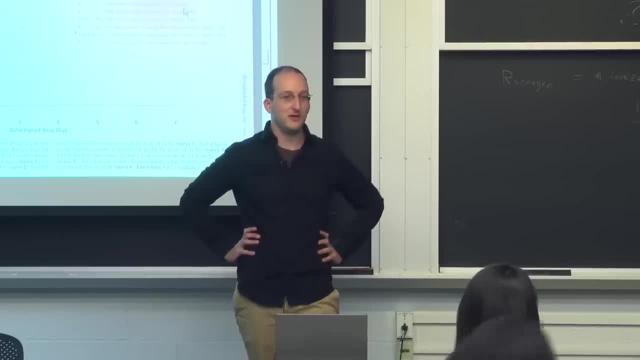 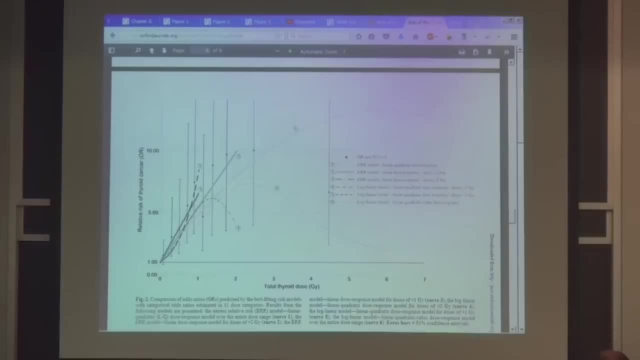 and slipped polonium into his tea at a Japanese restaurant. Just a drop or something. He moved back Really, I think. so right, He moved back. But it was a guy. He was like unsuccessful, What was his name? He died long term a couple years after. 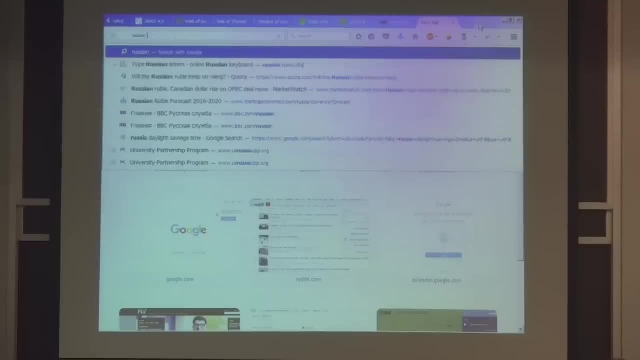 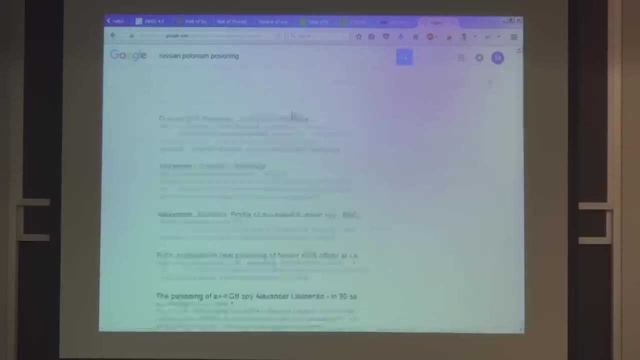 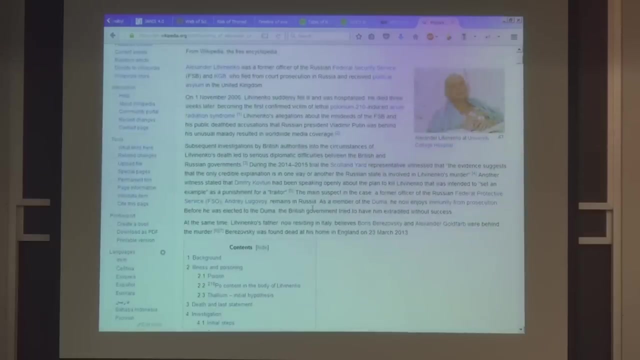 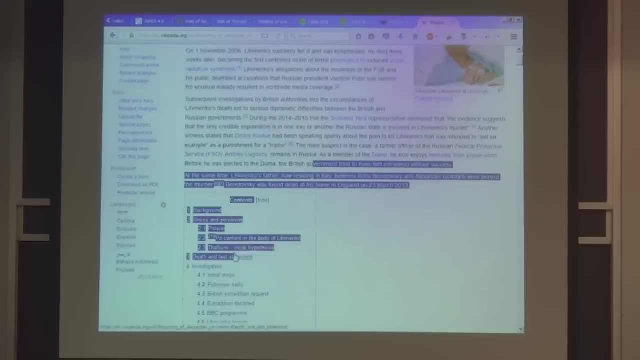 Let's see Polonium poisoning. Then polonium poisoning- Did he actually die? Poisoning of Alexander Litivenko: Yeah, that looks pretty close to dead. He's not doing too well. No Illness and poisoning, death. and last statement: 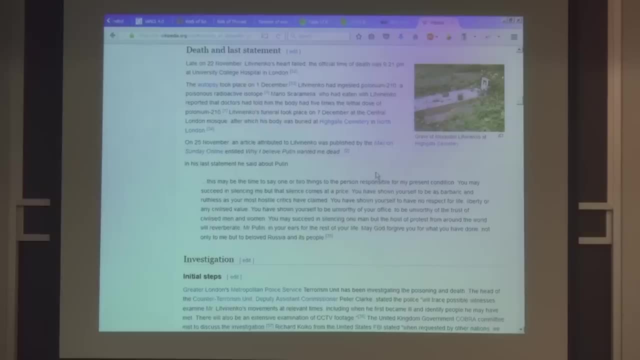 At the hospital in London. So, yeah, Well, he probably said something awesome. Well, what did he say? Well, interesting, That probably has something to do with it. Yeah, that's a really long class statement. Yeah, Well, we're not going to comment on the politics. 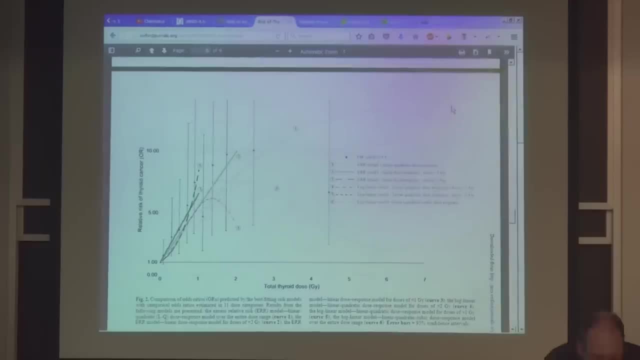 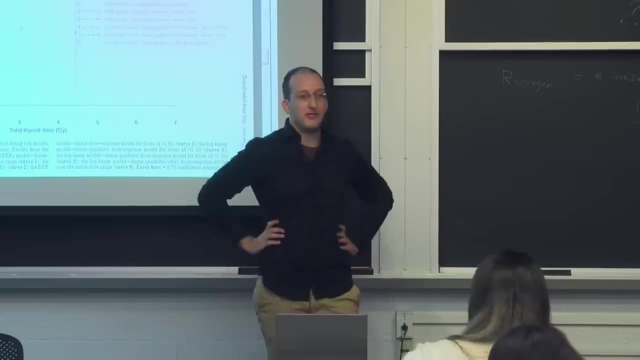 but the radiation effect worked clearly, unfortunately So. polonium is an alpha emitter and that caused a massive dose of alphas to his entire gastrointestinal tract And that caused a whole lot of damage to those cells. No time for cancer. It actually killed off a lot of those stem cells. And the way that radiation poisoning would work is that if you kill off the stem cells- the villi in your intestine die, which are responsible for absorbing nutrition, You can't uptake nutrition. You basically starve, Doesn't matter what you eat. 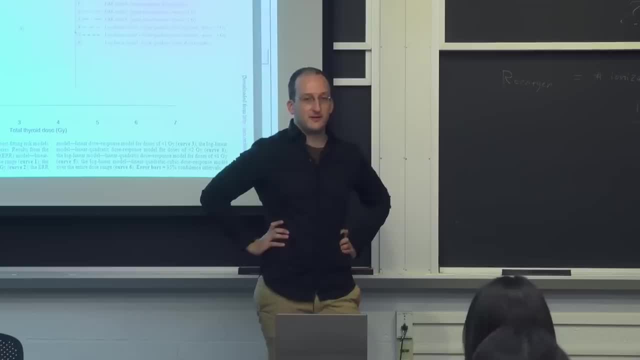 It's messed up. Yeah, That's a really bad way to go. It's called gastrointestinal syndrome And we'll be talking about the progressive. We'll be talking about some of the effects of acute radiation exposure, where you have immediate effects mostly. 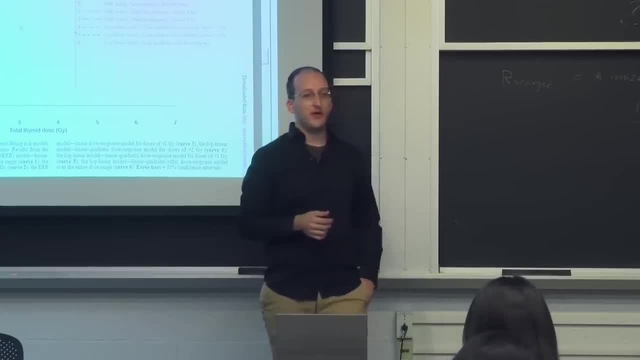 relating to the death of some organ that is responsible for either cell division to keep you alive or, in extreme cases, your neurological system And nerve function just stops at the highest levels of dose, And that corresponds to doses of around four to six gray. 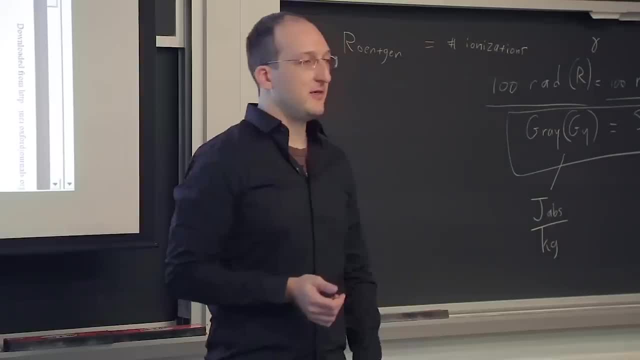 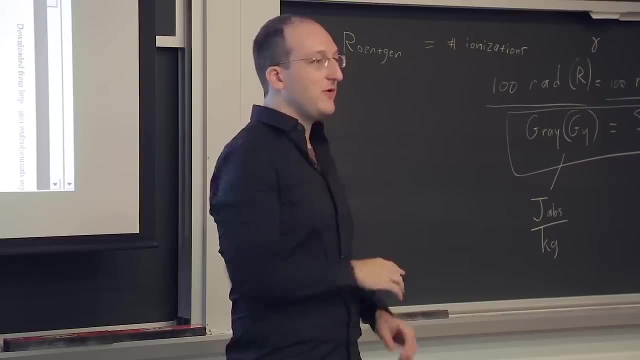 Four to six joules per kilogram of villi or body mass will kill you pretty quickly- Very little chance of survival, as what happened here, And so this was the problem with all the folks living around and near Chernobyl and Ukraine and Belarus. and everywhere was. the contamination was pretty extensive. About 4,000 people are estimated to have died or contracted cancer from this. I can't believe how low that number is, But it's still 4,000 people that it should never happen to. 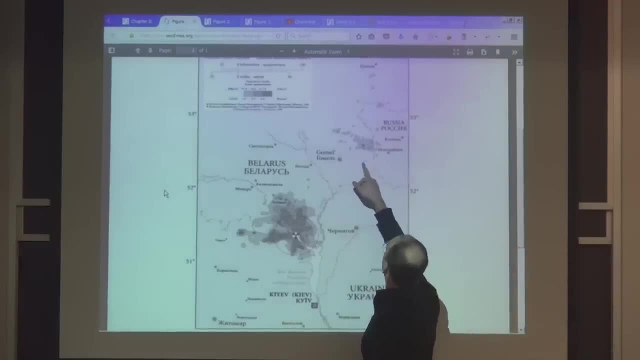 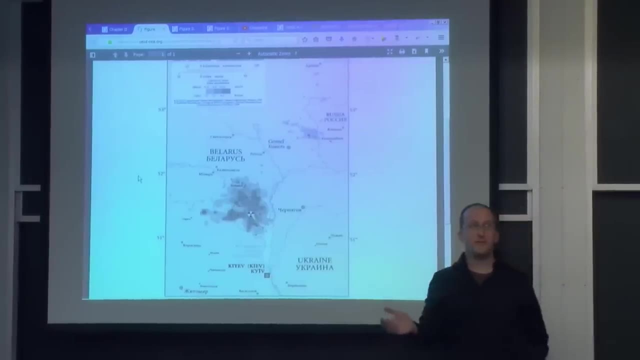 And effects were felt far away in towns like Gamal- And I can't read that one because there's not enough pixels, Because of the way that, let's say, rainwater whisked, or let's say, the vapor cloud from the reactor was whisked away. Rainwater caused it to fall on certain places which, still to this day, can have a really large contamination area. And this brings me a little bit into what should we be worried about from Fukushima? A whole lot less than Chernobyl. And the reason why is Fukushima did undergo a hydrogen explosion and did and still continues to release cesium-137 into the ocean. Luckily for us, the ocean is big And, except for fish caught right near around Fukushima, even though concentrations can be. measured at hundreds to thousands of times normal concentrations, they can still be hundreds to thousands of times lower than the safe consumption. So a lot of the problems you see in the news today. I'm not going to call them lies, but I'm going to call them half-truths. 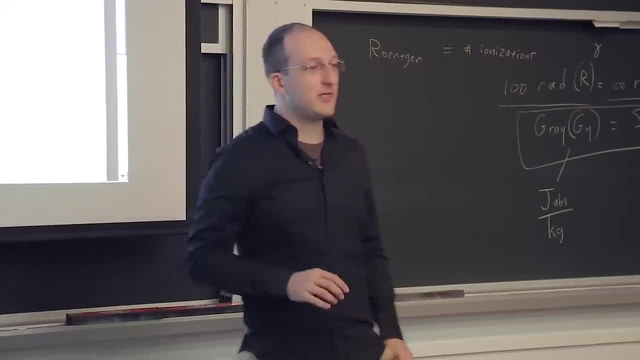 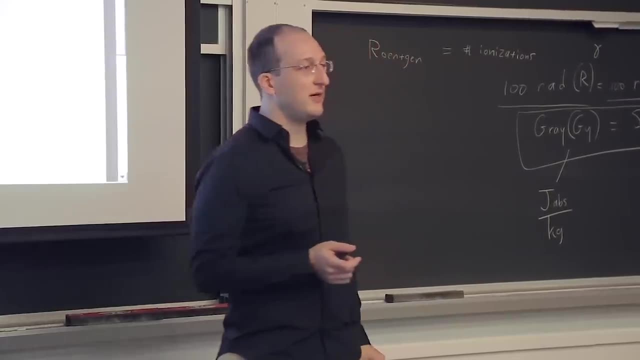 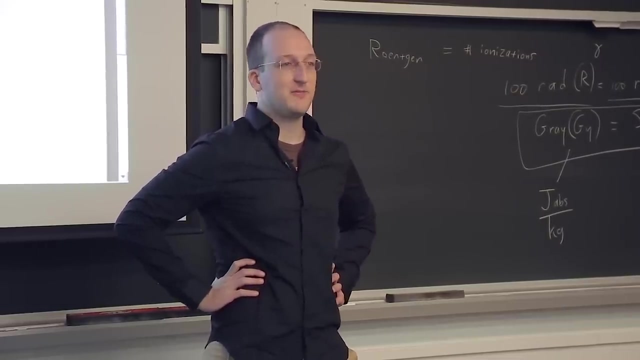 Folks will show the radiation plume of cesium-137 escaping from Fukushima, And that's true. There is radiation escaping. The question is: is it high enough to cause a noticeable increased risk of cancer? That's the question that reporters should be asking themselves when they only 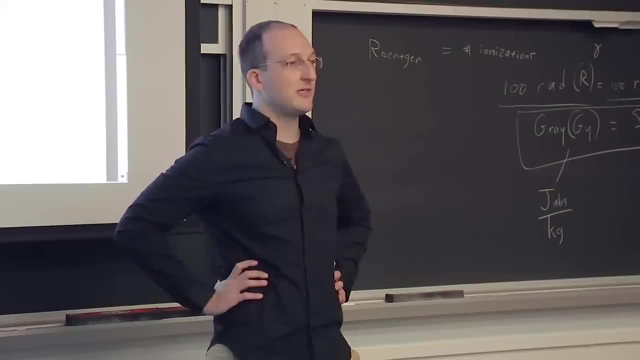 tell the half of the story. that gets them viewers, and they don't tell the half of the story. to complete the story and tell you should you be afraid or not, Because unfortunately, fear brings viewers. This is the problem, And I'm happy to go on camera saying this. 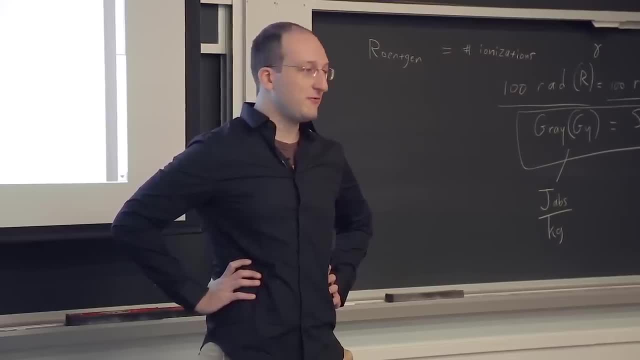 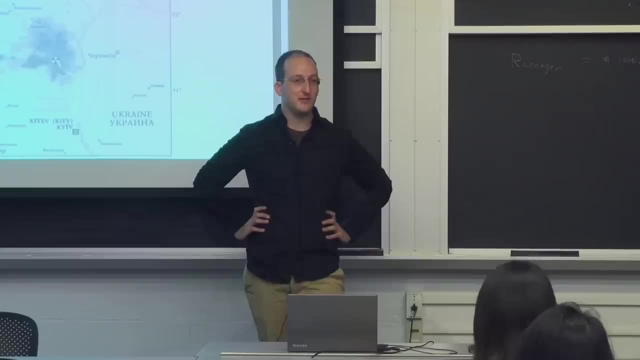 This is the problem with the media today is, with a half-truth and with a half-story, you can incite real panic over non-physical issues that may not actually exist, And so it's important that the media tell the whole story. 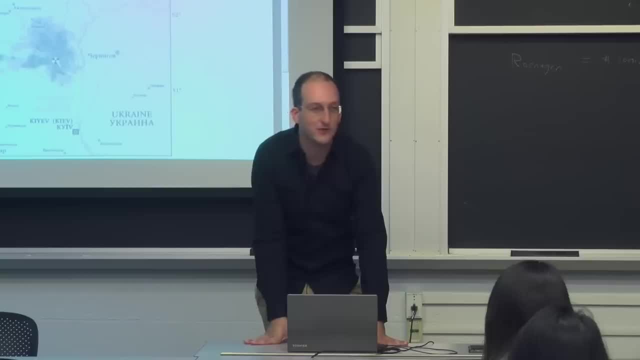 Yes, it's true that Fukushima is releasing cesium-137.. How much, though, is the question that people and the media should be asking themselves, And in the rest of this course, we're going to answer the question: how much is too much? 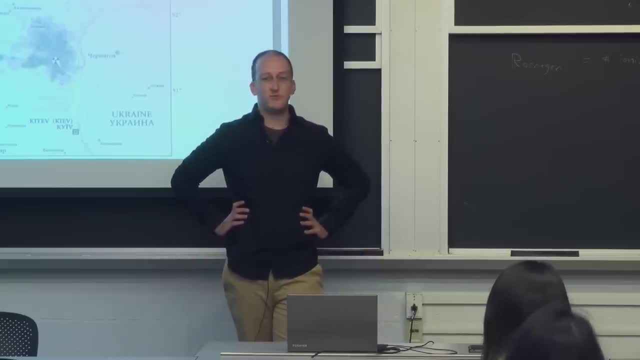 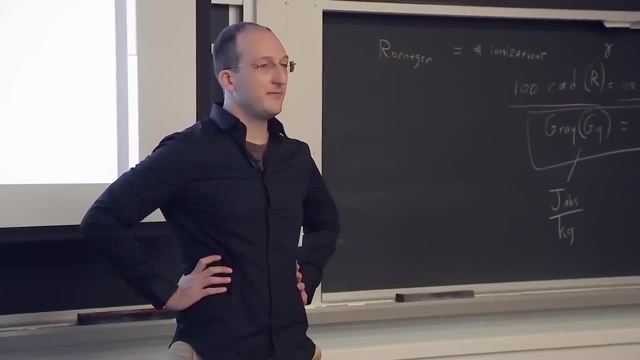 So I'm going to stop here, since it's two of five of, And I'll ask you guys if you have any questions on the whole second part of the course or what happened in Chernobyl. Yeah, Yeah, could you explain the quality factor term? 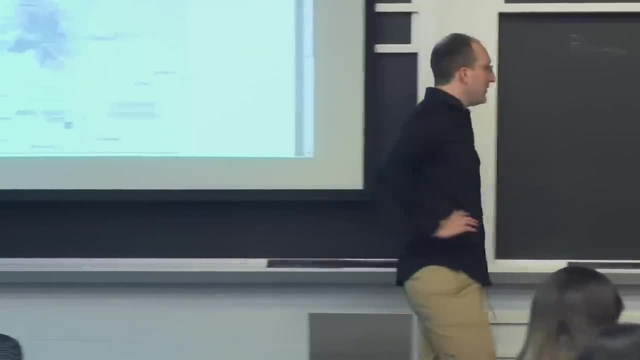 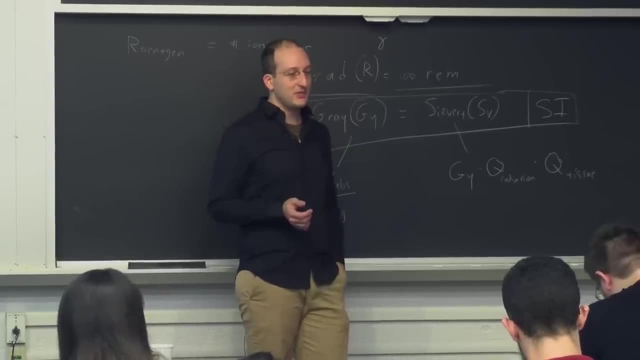 and how you find that, MICHAEL SHORTENBERG- Yep, Well, there's two quality factors. There is the quality factor for radiation, which will tell you how much, let's say how much more, cell damage a given type of radiation. 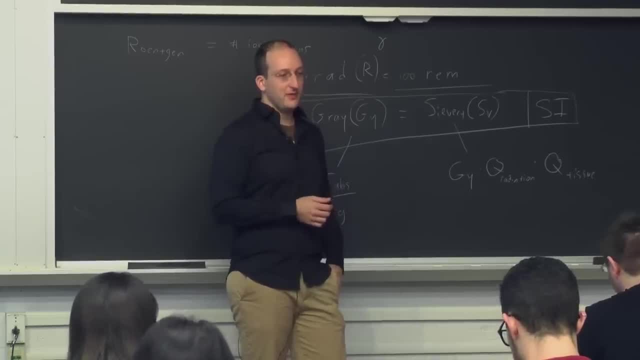 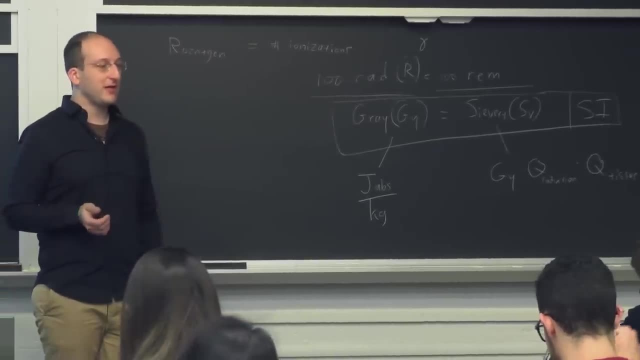 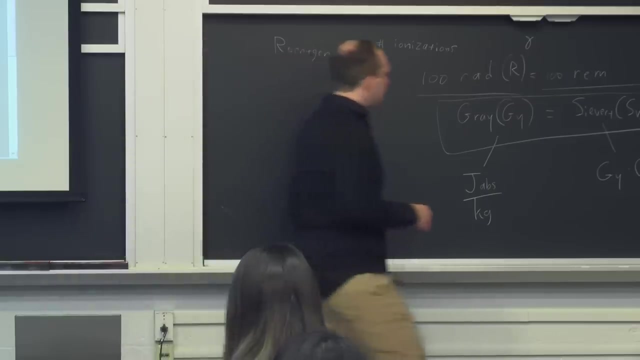 of the same energy will deposit into a cell And the tissue equivalency factor tells you well what's the added risk of some sort of defect leading to cell death or cancer or some other defect from that radiation absorption. So to me, the tissue equivalency factor, 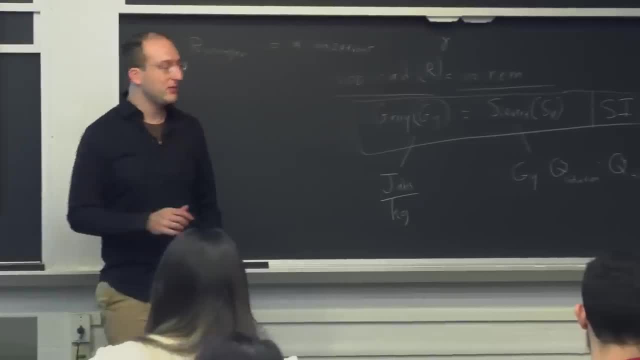 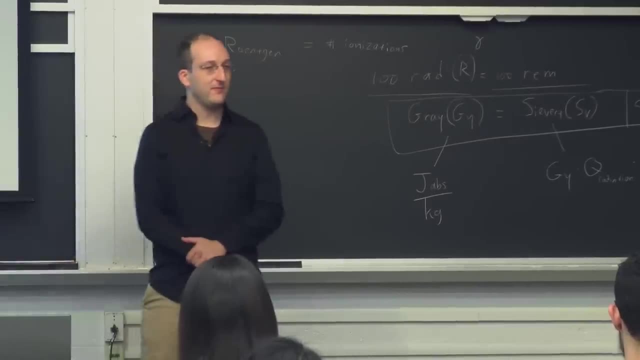 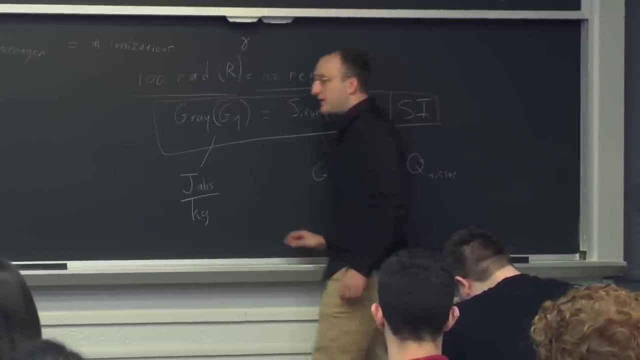 is roughly, but not completely, approximated by the cell division rate, And the radiation quality factor is going to be quite proportional to the stopping power. You'll see a term called the linear energy transfer or LET. This is the stopping power unit used in the biology community. 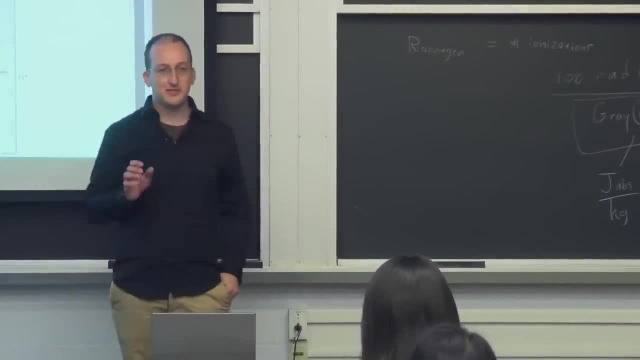 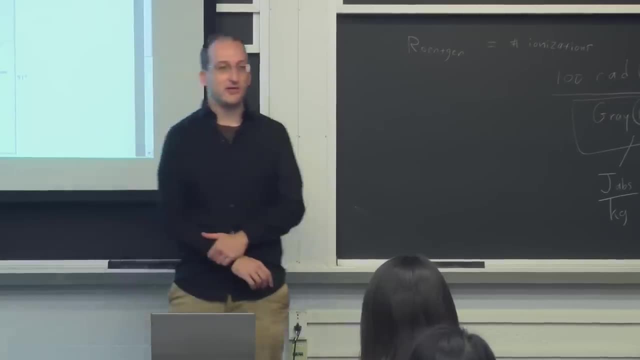 It's stopping power And luckily the Turner reading actually says it somewhere buried in a paragraph. LET is stopping power, So if you start plotting these two together, you might find some striking similarities. I saw two other questions up here. Yeah, 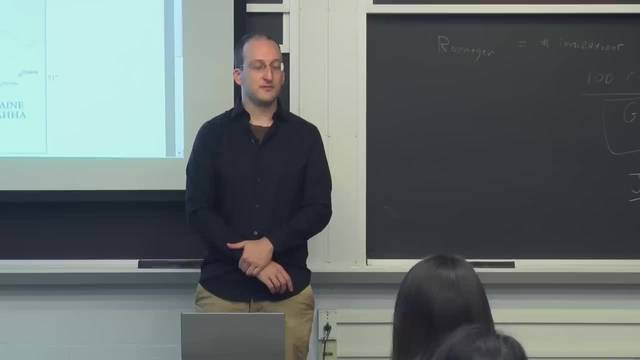 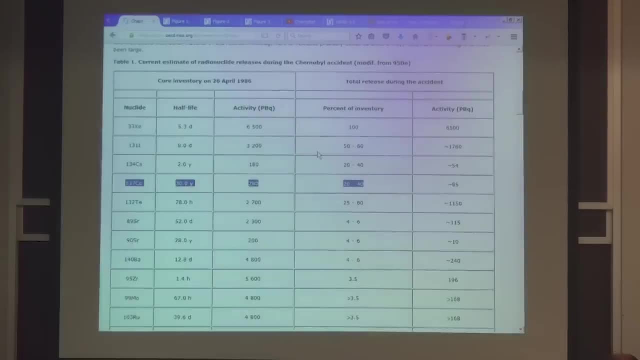 I was going to ask: why is Chernobyl still considered off limits if most of the half-lives of these things are on the range of days to, let two years? Let's answer that with numbers. So most of the half-lives were on the range of days to hours. But still. cesium-137,, with a half-life of 30 years, released a third of an exabecryl. That's one of the major sources of contamination still out there. In addition, if we scroll down a little more, 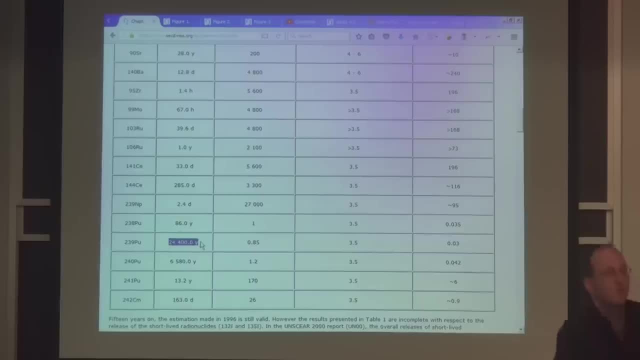 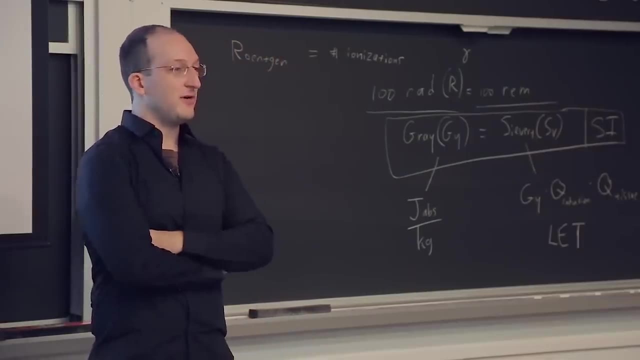 there was quite a bit of plutonium inventory with a half-life of 24,000 years. So on Friday we're going to have Jake Heckler come in and give his Chernobyl travelogue, because one of our seniors has actually been to Chernobyl. 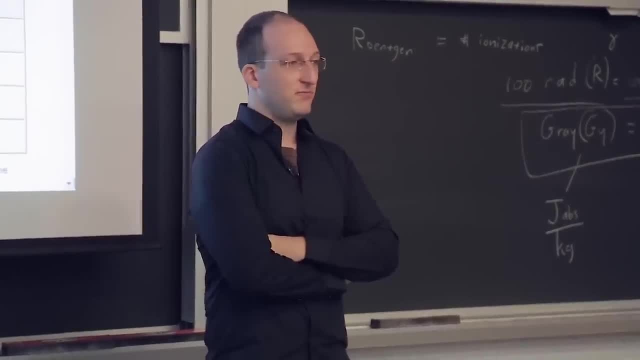 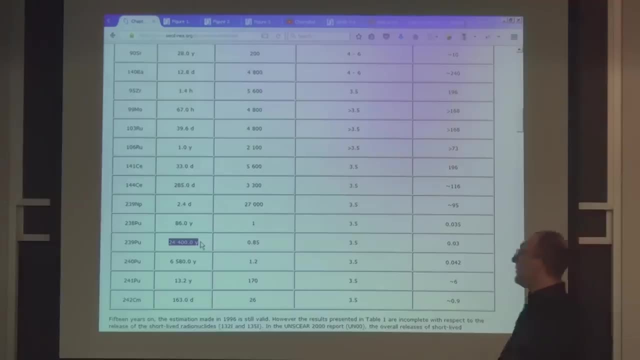 And his boots were so contaminated with plutonium that he can never use them again. They've got to stay wrapped up in plastic. So some of these things last tens of thousands of years, And even though there weren't a lot of petabecryls. 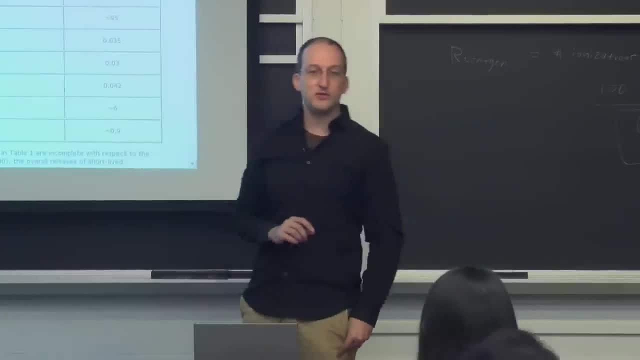 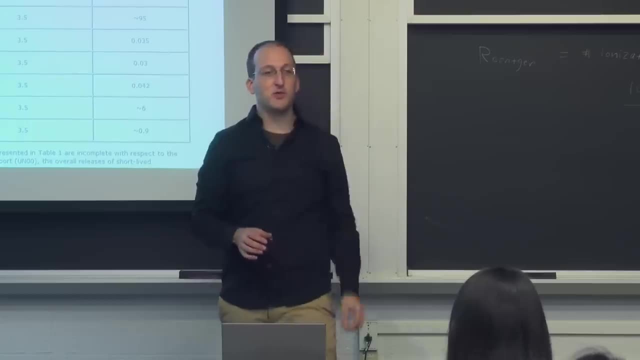 of plutonium released. they're alpha emitters And they're extremely dangerous when ingested. So greens and things that uptake radionuclides from the soil, like moss and mushrooms- So these are the things that are really dangerous And they're very dangerous. 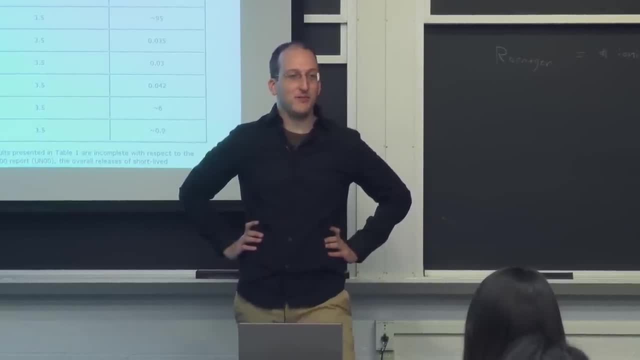 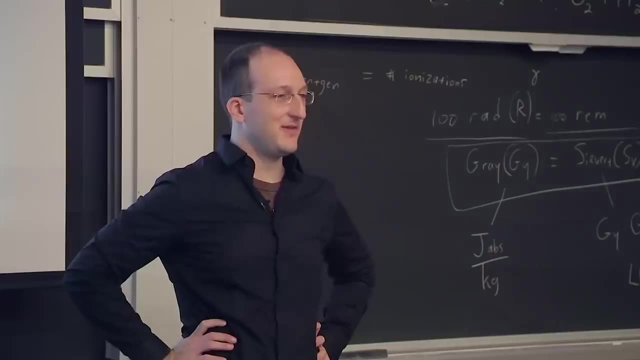 So we're going to look at the other ones. So the other ones are totally off limits. in a large range of this area You will find a video online, if you look, of a mayor from a nearby town saying, oh they're. 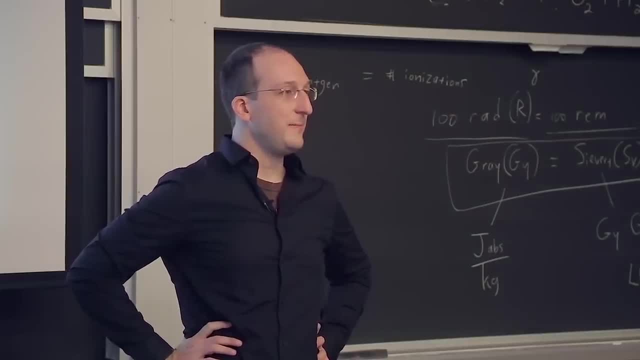 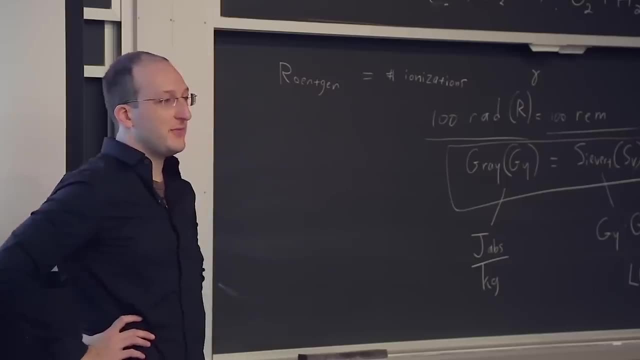 perfectly safe to eat. Look, I eat them right here And I just say: read the comments for what people have to say about that. Not too smart, Yeah. So what's the process now for taking care of Chernobyl? What are they doing? 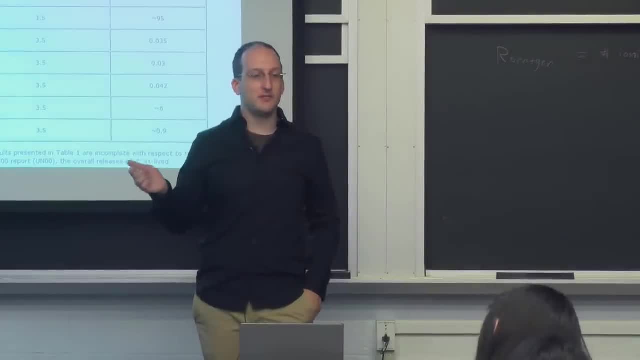 So the sarcophagus around the reactor's there And, let's say, rainwater comes in and starts washing away more stuff into the ground or whatever. We don't want that to happen. Soil replacement and disposal as nuclear waste is still going on. 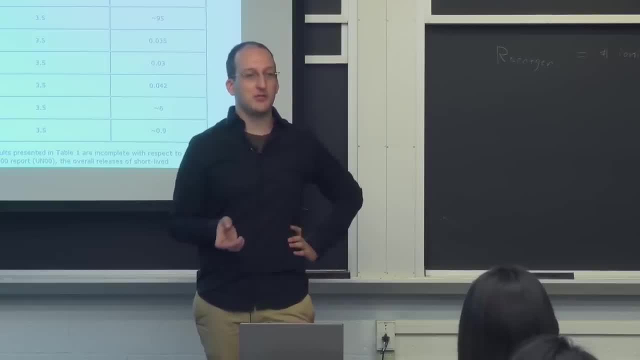 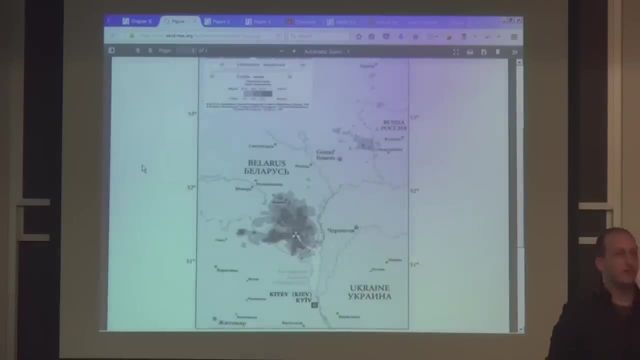 Removal of any moss, lichen, mushrooms or anything with a sort of radiation exposure has got to keep going, But the area that it covers is enormous. I don't know if we're ever going to get rid of all of it. The question is, how much do we have to get rid of to lower? 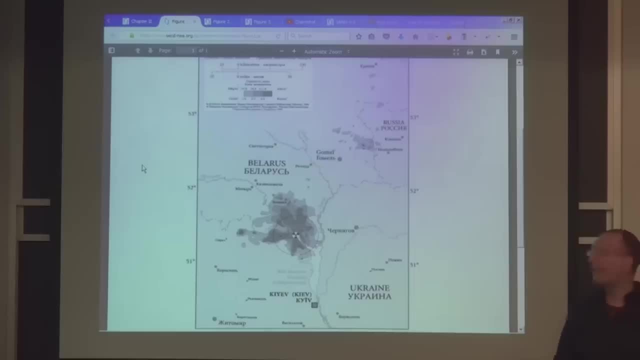 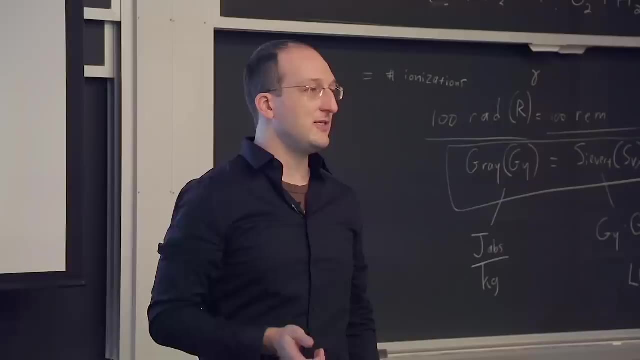 our risk of cancer in the area to an acceptable rate. Yeah, There will likely be parts of this that are inaccessible for thousands to tens of thousands of years, unless we, hopefully, get smarter about how to contain and dispose of this kind of stuff. We're not there yet. So right now the methods are kind of simple: Get rid of the soil Fence off the area. Some folks have been returning And they do get compensation and free medical visits because the background levels there are elevated, but not that high. 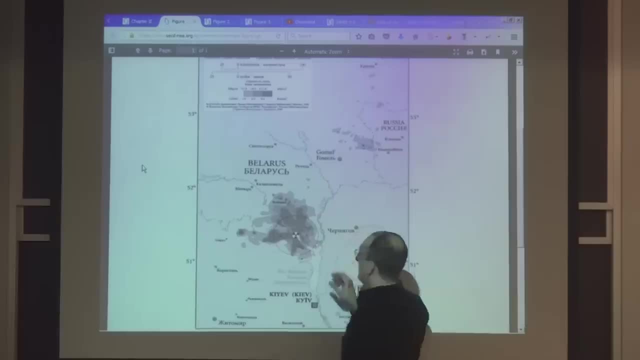 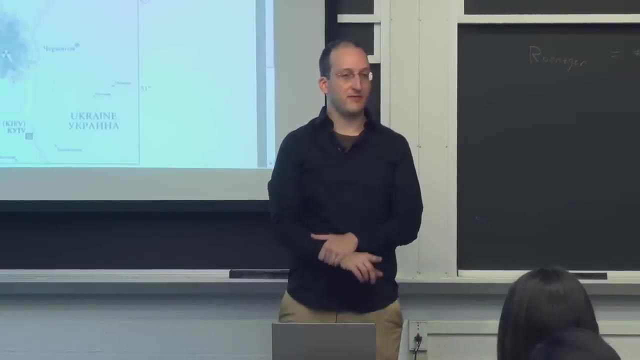 So folks have started to move back to some of these areas, But there's a lot that are still off limits. Any other questions? Yeah, It's like way worse than the atomic bombs dropped on Hiroshima and Nagasaki, because those are like four functioning cities at this point. 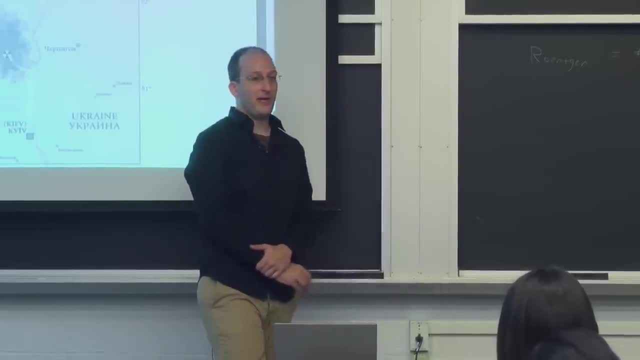 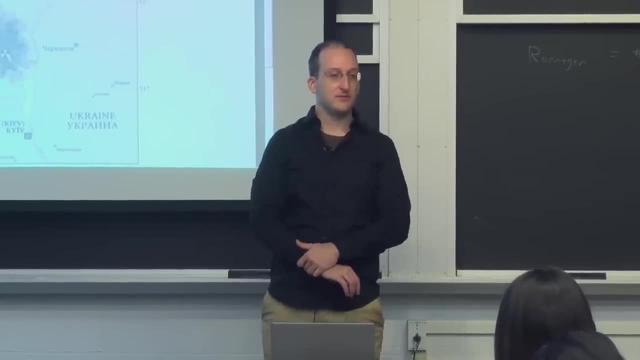 MICHAEL SHORTENBERG- Yeah, the number of deaths from the atomic bombs way outweighed the number of deaths that will ever happen from Chernobyl. But why is the radiation from those bombs not? MICHAEL SHORTENBERG- Oh, not that much of an issue.